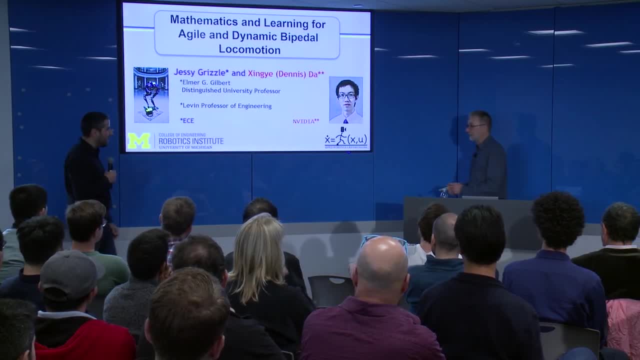 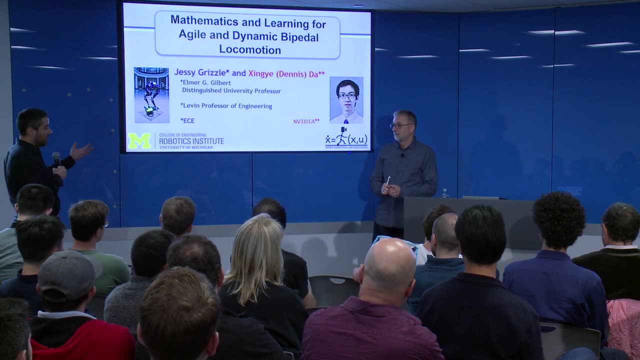 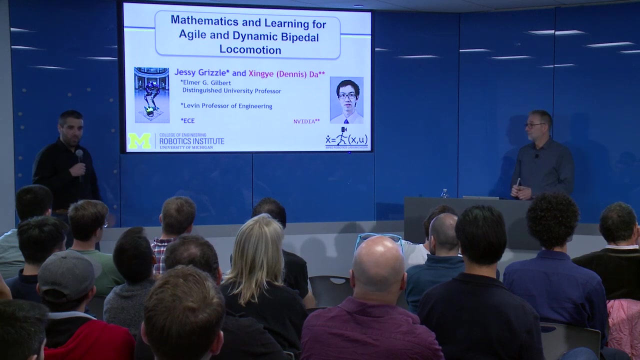 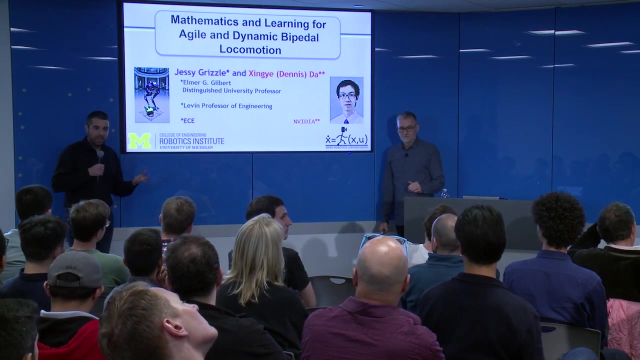 he's also the director of the Robotics Institute, still kind of a new institution at Michigan, which is great to see focused efforts around robotics. I guess what I wanted to say about Jesse is that the sort of a testament that the old cliche of academic freedom sometimes 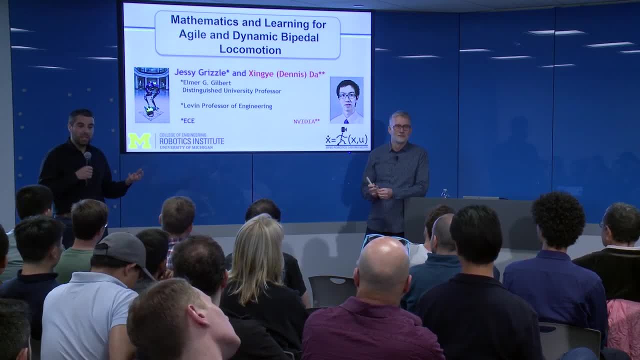 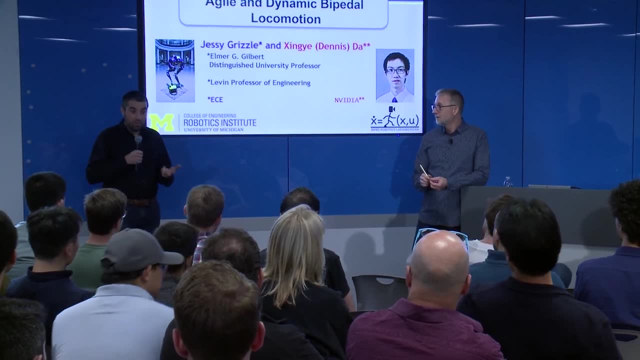 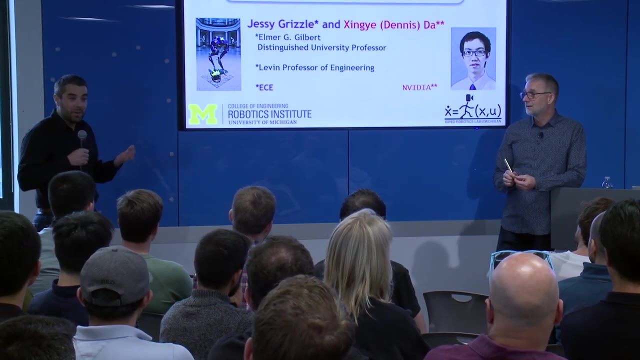 is actually true. We probably know Jesse mostly for his work on bipedal robot locomotion, but it turns out I didn't know about this. we learned the other day that he didn't bother to start worrying about robotics until he was a full professor. 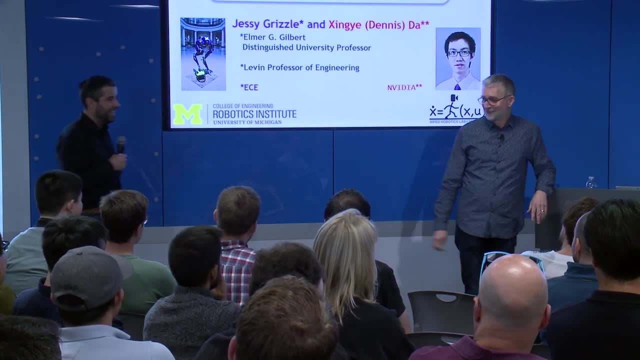 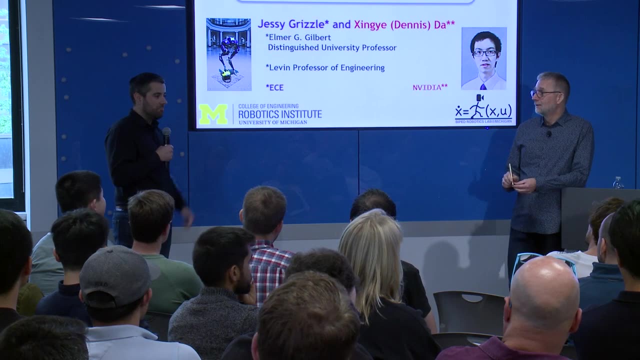 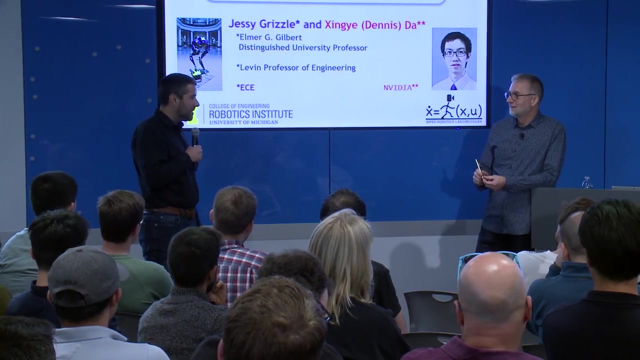 And before that he had had like two other careers with great contributions on power management and emission control in cars, semiconductor industry, many things. And then one day he said: you know what I do controls. It looks like an interesting problem. It looks like 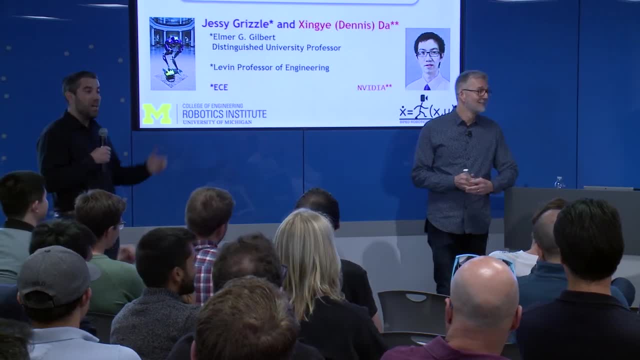 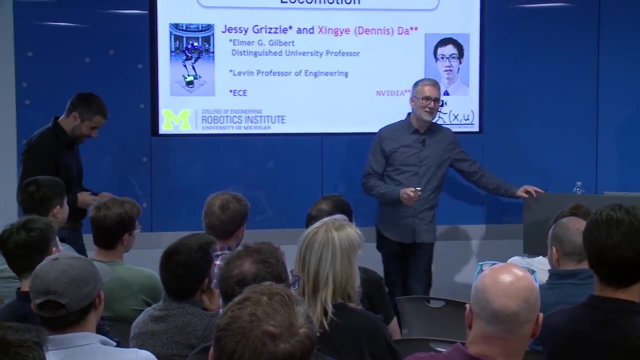 no one else is doing it the right way. So today he's going to explain us what is the right way to do it. A way, A way, A new way, A new way. Never the right way. Thank you very much, Alberto Songbei. I had to turn you down last year. I'm really. 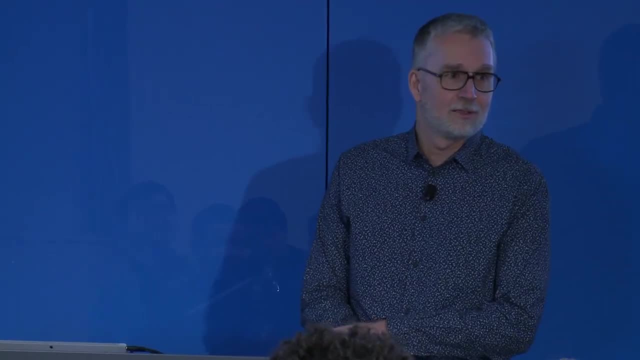 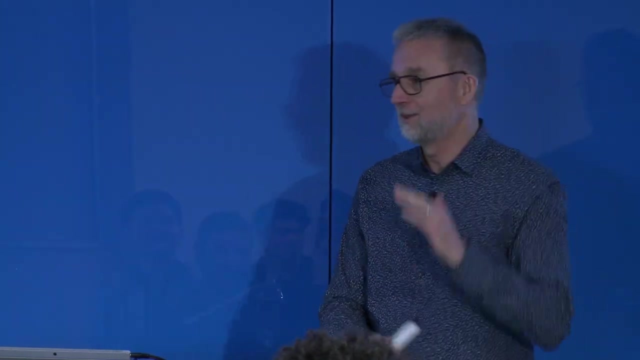 happy you reached out again. I want to thank Fang Zhao and Nima for tirelessly getting me from place to place, and, Lisa, all the stuff you did to make sure that the trip here was easy and well organized. I appreciate that very much too, So thanks for inviting. 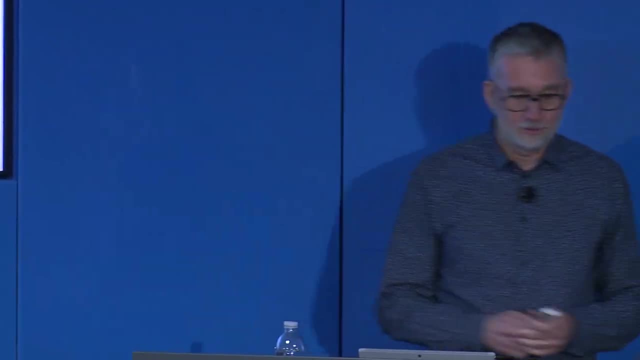 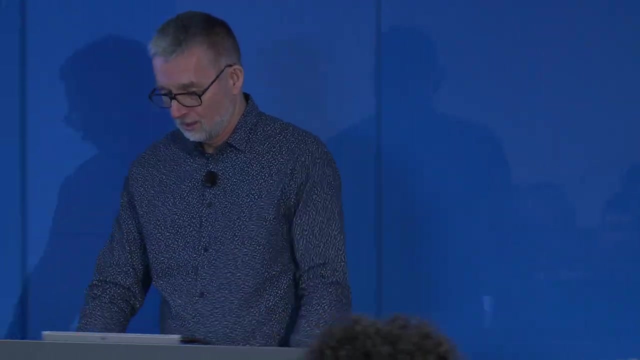 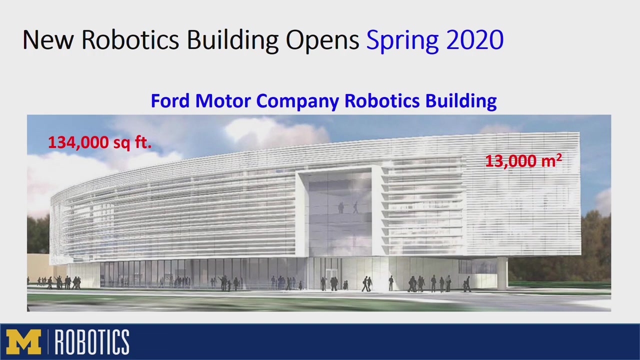 me. This is work mostly by Dennis Da, So he's at NVIDIA Robotics now. He spent some time in Pittsburgh and just recently moved out to the West Coast there. First I'll say a few words about the Robotics Institute. So this is done in collaboration with Ford At. 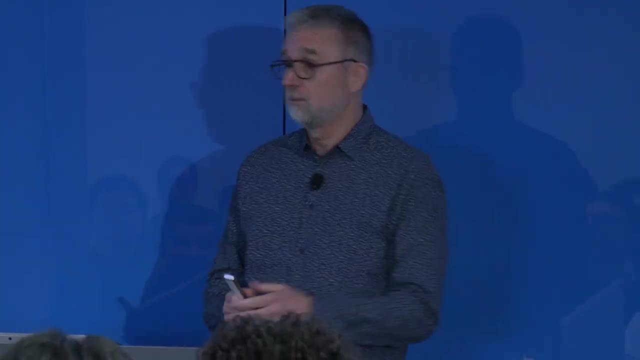 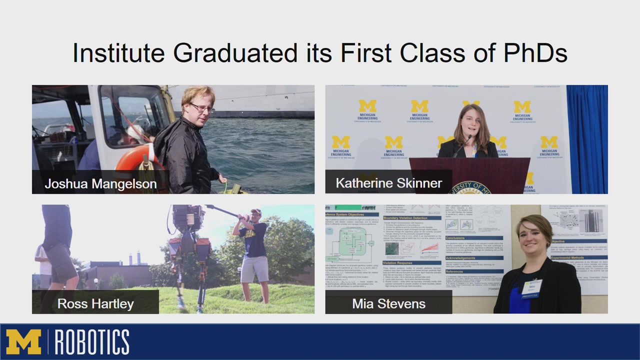 least for us, it's a new thing to have a private company with a presence on campus. We've graduated our first class of PhD students, so we just started year six of the robotics graduate program, So you can get a degree in robotics that has the same stature. 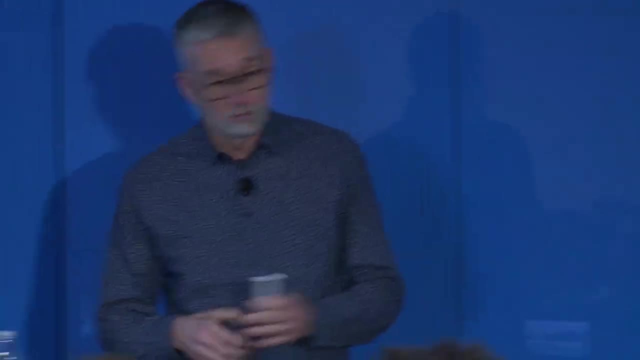 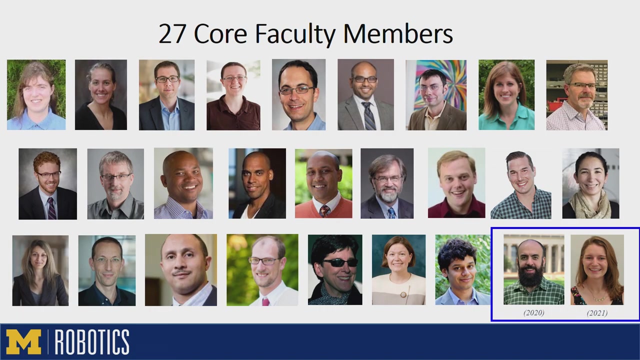 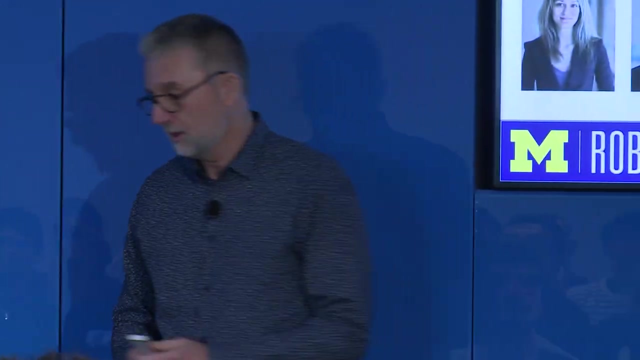 degree in aerospace or mechanical engineering, etc. We're not a department, we're an institute. These are the core members, meaning the people who are doing double service duty to their home department and to us. These are people who are really heavily, heavily committed to doing. 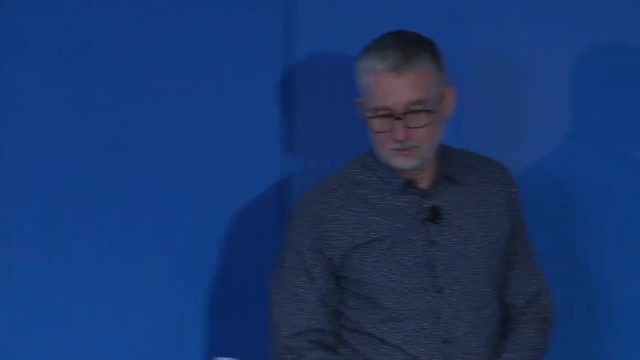 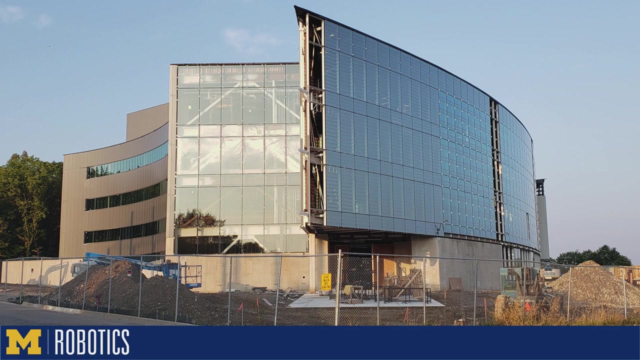 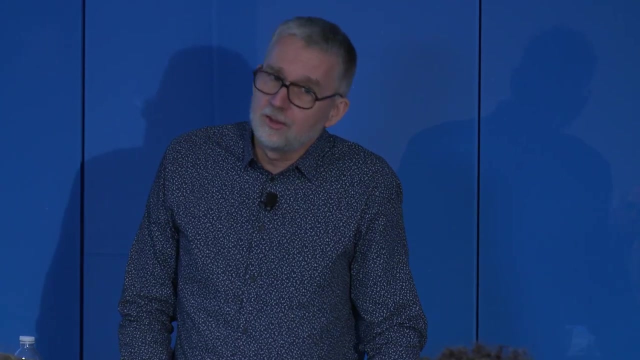 robotics, and we're definitely looking forward to NEMA joining us in September. Katie was one of our first PhD graduates. She'll join us after a postdoc at Georgia Tech, So the building will open, or well, it'll be substantially complete, which is a legal term. 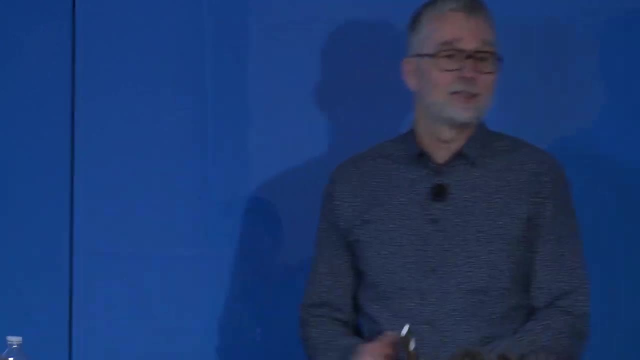 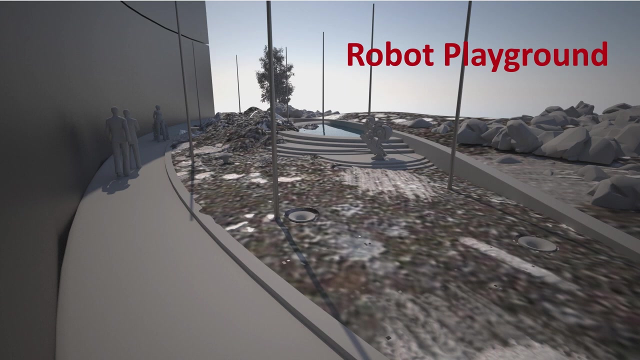 I don't quite understand- substantially complete on Valentine's Day. So if you guys come in the summer, we should be moving in and getting all the labs set up. One of the unique features that's being built right now is it will have a robot. 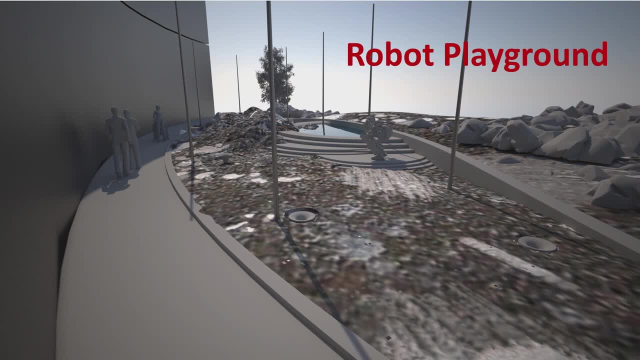 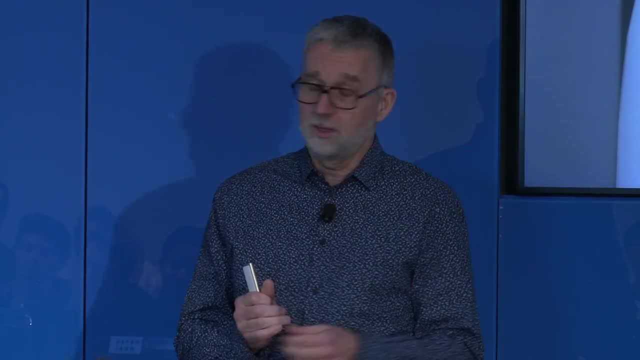 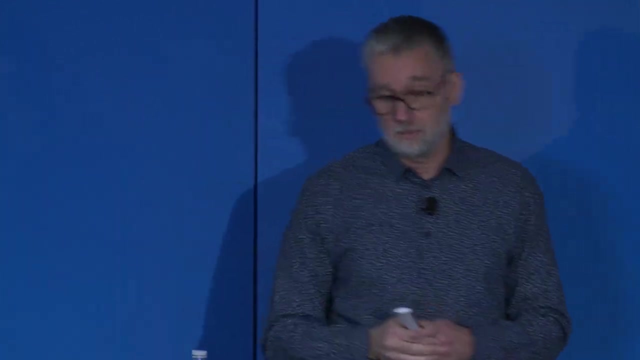 playground attached to it, And if it looks a little bit alien, it's because it was designed as a collaboration between our school of architecture and a robotics PhD student using neural nets. So this is a dreaming and overlaying textures on outdoor environments which came up. 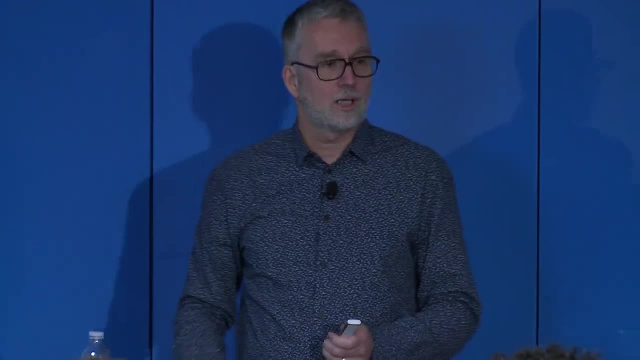 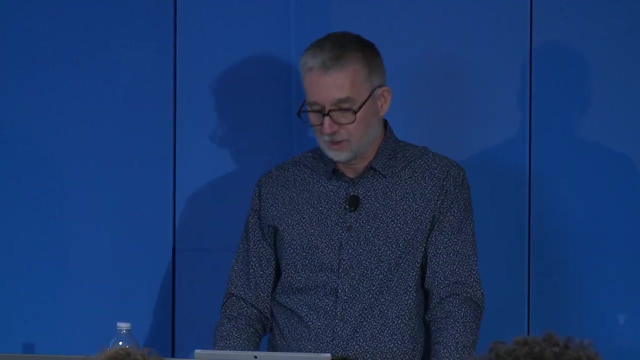 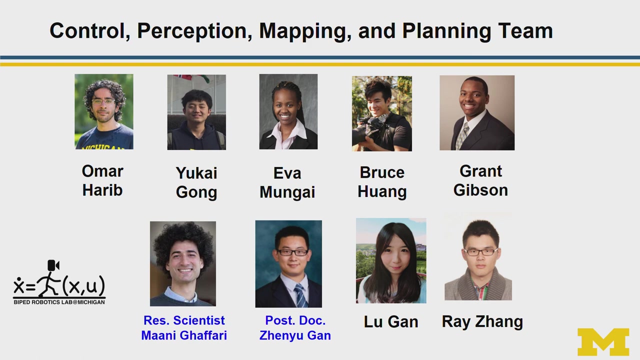 with this And the key thing is all the steps there. they're all different heights and different tread depths so you cannot do anything open loop to walk up on on the on that water feature. So this is my team. I've typically worked with a small number of students, four to 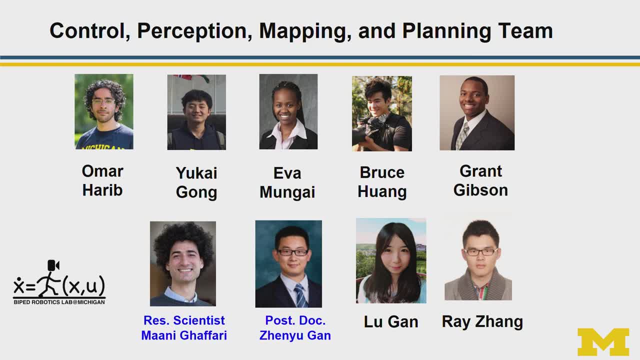 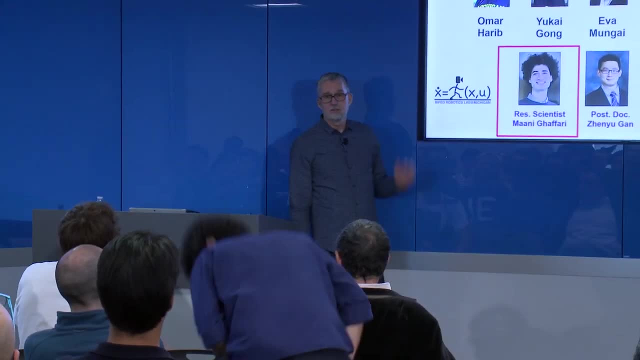 five PhD students, Because Ryan Eustace is at TRI. I've had the great pleasure- part of his group joining mine And so we have- we have Monty here. So Monty stand up. So come on, stand up, it's okay. So he's a research scientist with Ryan and me and he brought in 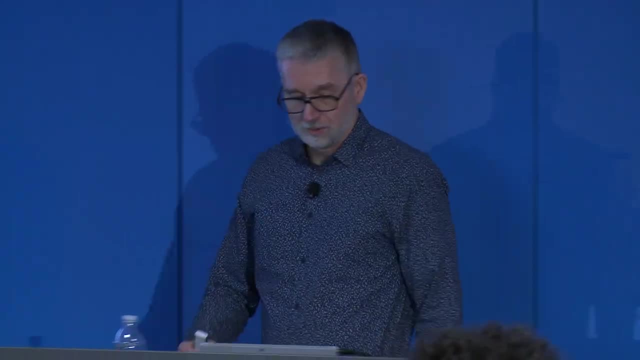 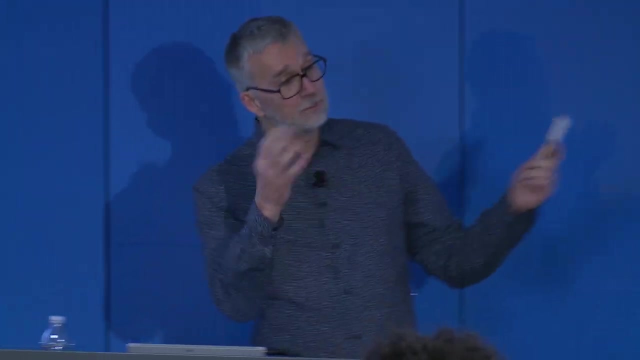 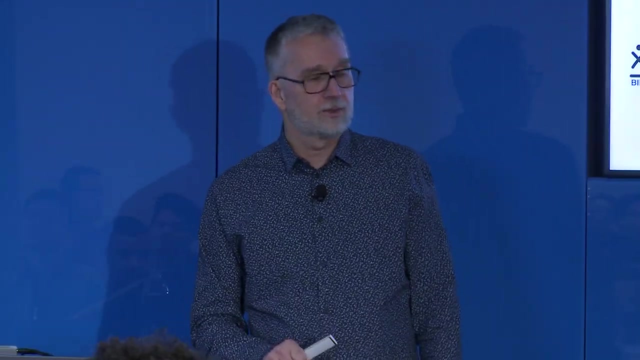 Lugan and Ray Zhang from Ryan's group, and so that's added now that we can go more from blind walking into perception and planning. Today I'll be talking about blind walking, feedback, control, those little boring things. okay, But we spent a great part of yesterday afternoon in Songbei's. 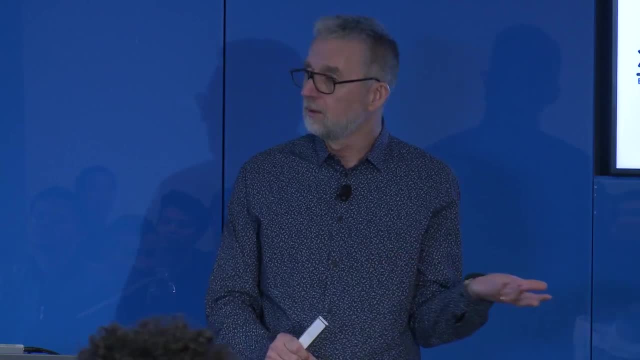 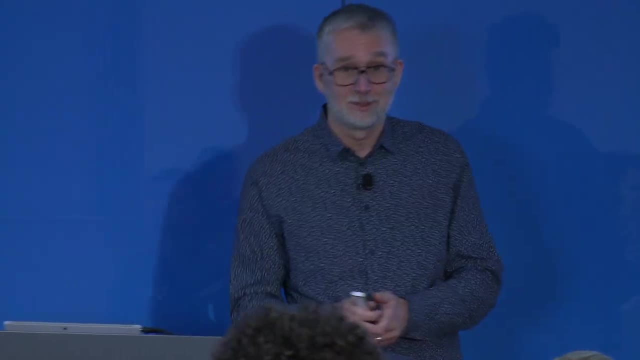 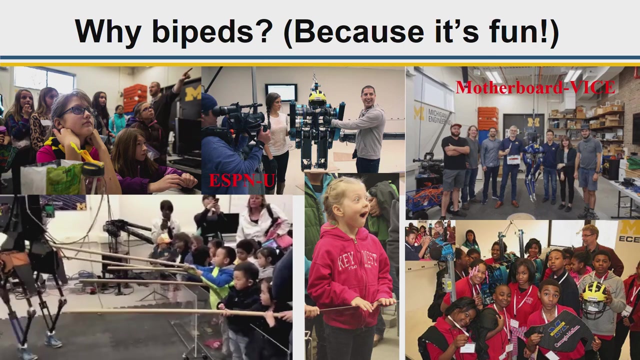 lab going through this and I guess Monty's going to be visiting with Luca a little bit later. So if you want to see more about our planning and perception work, maybe Luca could invite you as well When Monty is presenting right after the this seminar. So I often have to defend why I'm working. 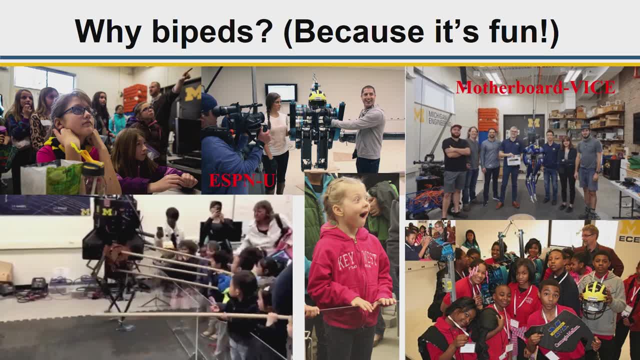 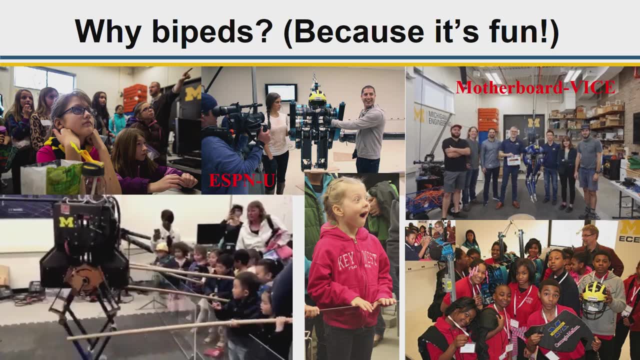 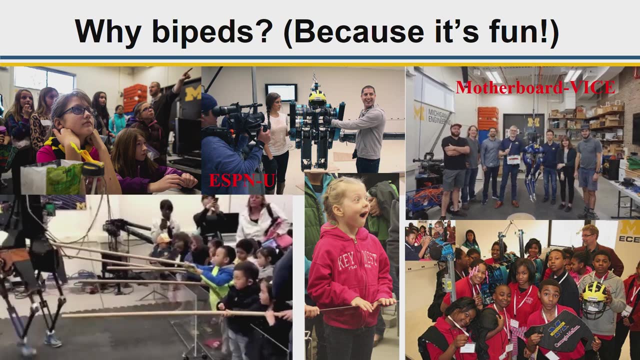 on bipeds and not something more practical like quadrotors or quadrupeds and stuff. and I just tell them I do it for fun, okay, When I used to work on automotive systems and or I used to do proofs and abstract differential geometric methods, in control, no one came to visit me in my isolated office while 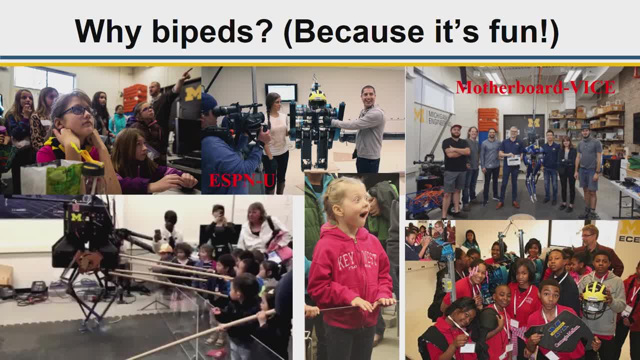 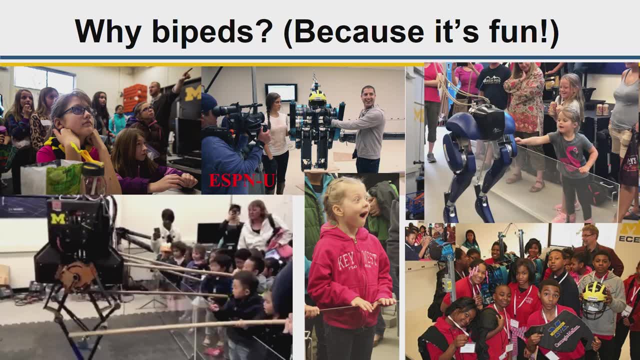 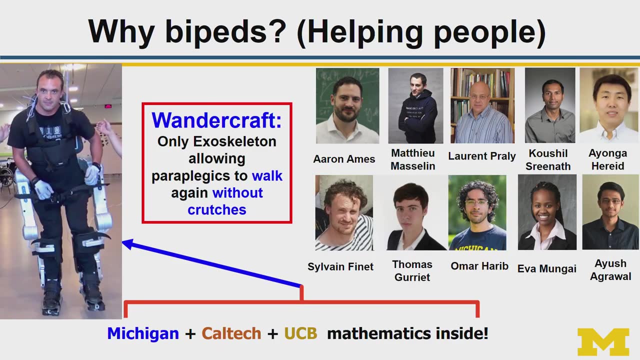 I was working, Nobody cared. you know you don't get these looks of joy when something happens. that only happens when you play with robots. you know we're very privileged to be able to work in this space, But we also we also feel more fulfilled when we can do something practical with this work. 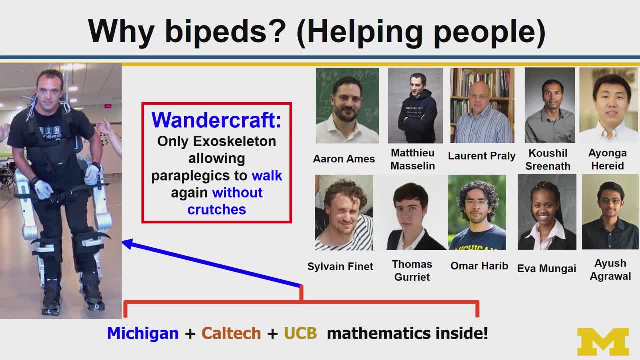 So my lab is fundamentally focused on the mathematics of control for walking. that's really important, But we don't want things that work on only one robot. we want to solve whole families of robots at one time, And so one of the ways that we've taken our work on bipeds like Cassie and 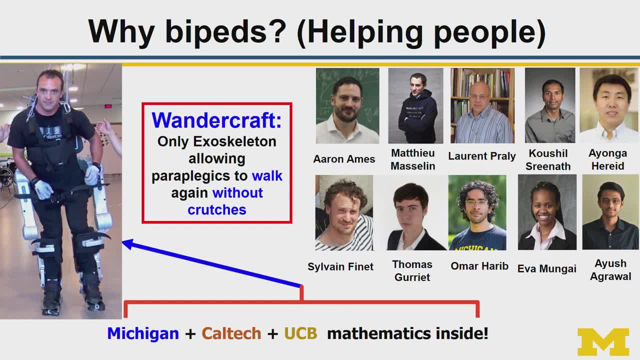 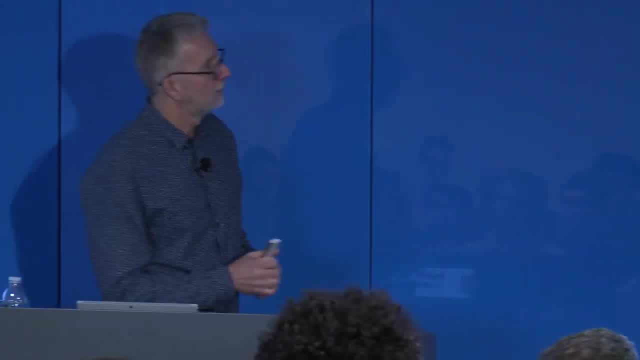 Marlo that we'll see more of later today is we've teamed up with Wondercraft, a startup in Paris, and you might notice a few other people you know, like Kaushal and Laurent Prally and Aaron Ames, etc. to work with Wondercraft to build an exoskeleton and allow the robot to move around, And so we've 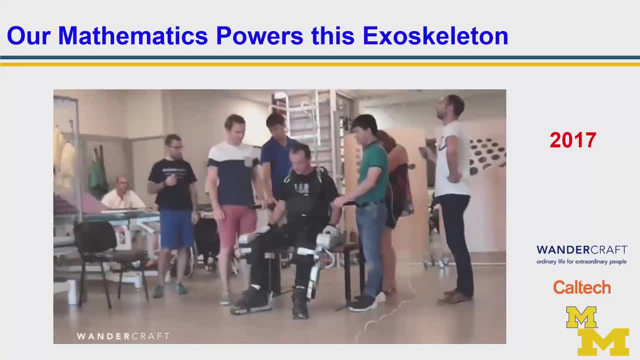 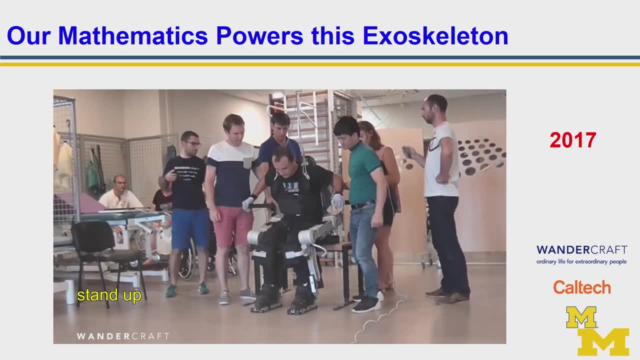 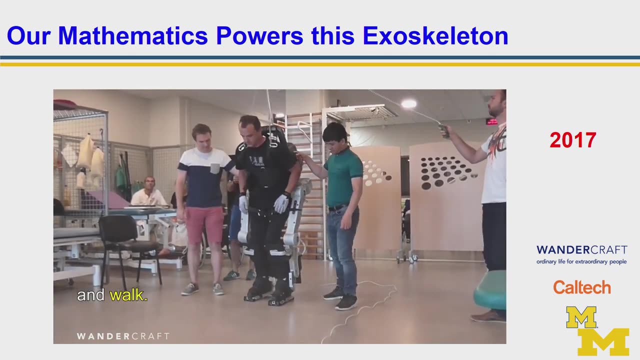 built a robot that allows people who are paralyzed from the waist down to walk without the use of crutches. So this is a two-year-old video. somewhat early in the design scale. Oscar is the first time he's up and walking after his accident. The IRB requires the assistance. There's a safety cable. 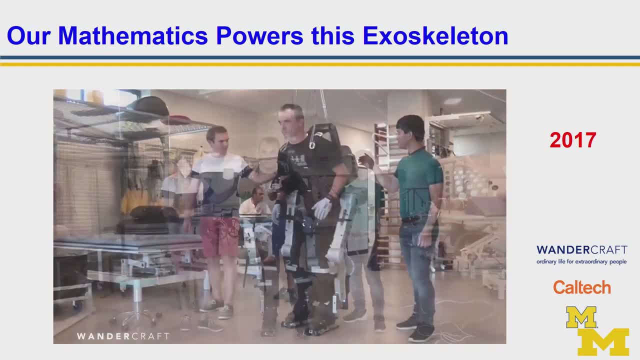 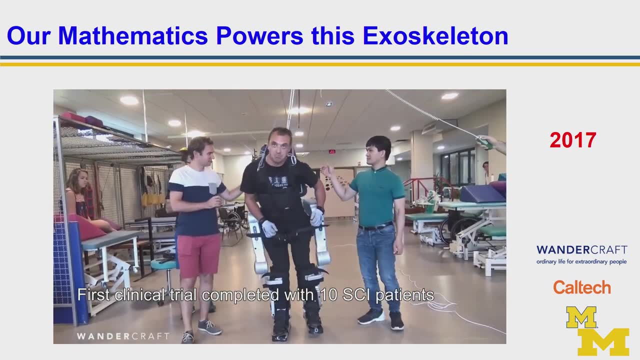 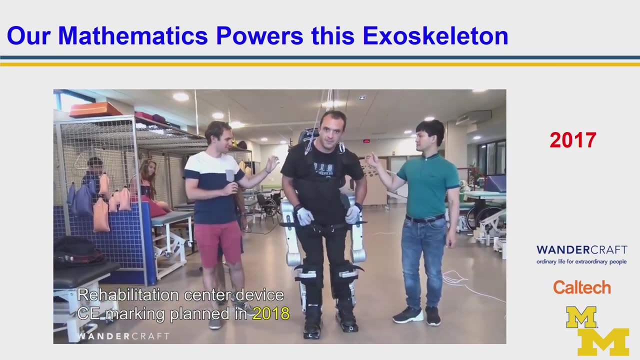 Nothing can happen to Oscar. He's feeling a little uncomfortable, He's starting to get into it. All of the stability is provided by the device, just like we would on Cassie or Marlo, And so they got this going and they've tested it on about 10 different patients. When you're there and you 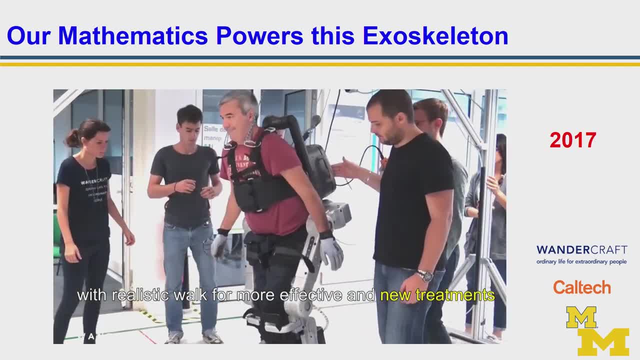 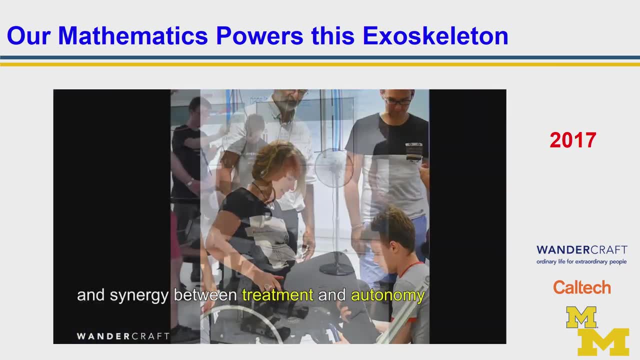 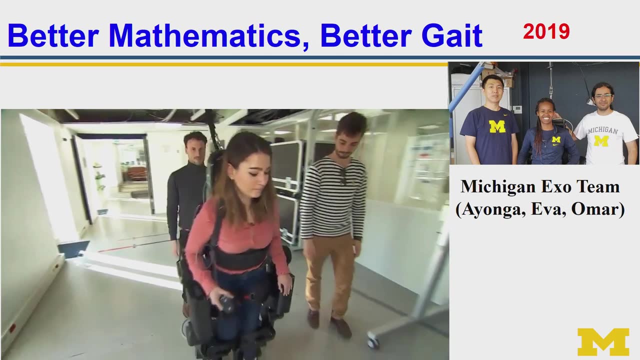 see the parents crying because they're seeing their loved one up and walking. I mean it's. I didn't think robotics would bring tears to my eyes but it has. And if you saw, that gate was kind of awkward. Everybody was leaning forward in it. It's because the mass distribution on the 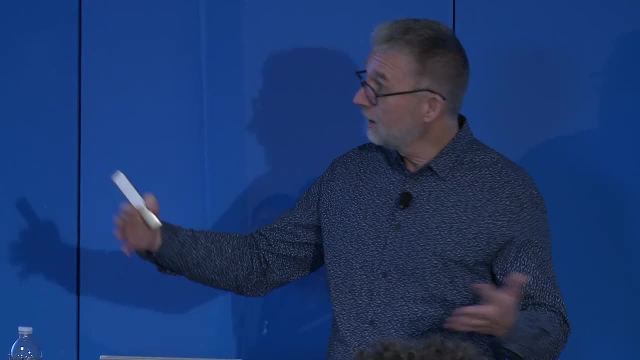 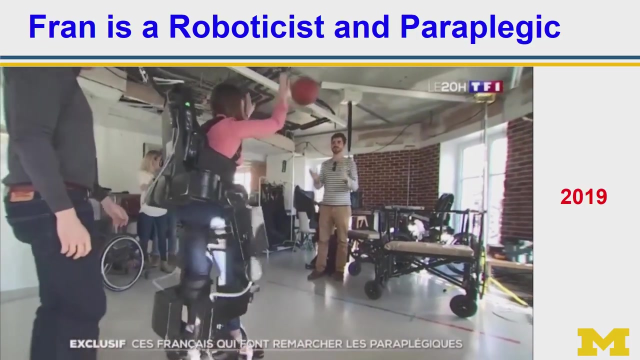 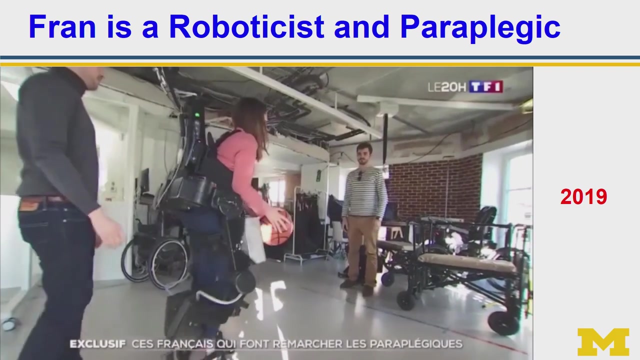 exoskeleton was wrong, And so we helped them redesign the placement of the batteries etc. And also improve the control laws and the trajectories for the gate, And so it's stable enough that you can have independent activity in the device. So these are now being sold. 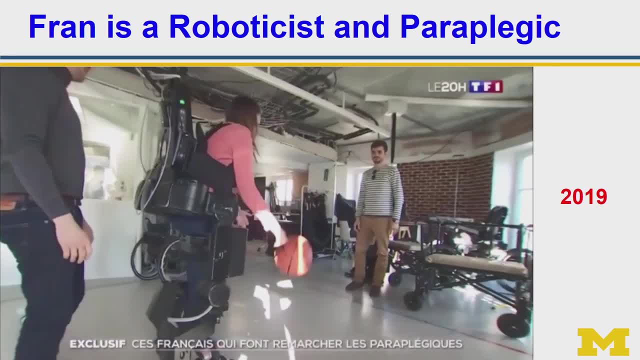 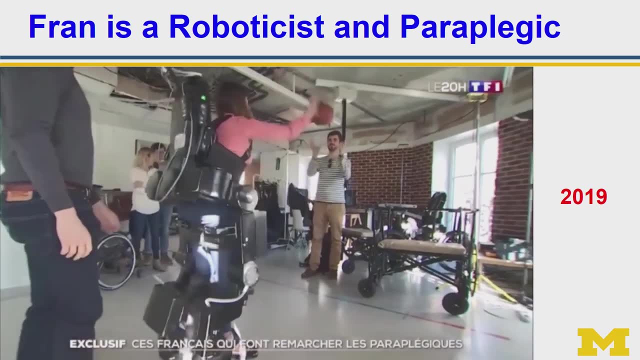 to rehabilitation centers. And, to be clear, they're being sold to rehabilitation centers. And, to be clear, I have no financial interest in this any at all, and neither do my students. We just do it because we want to get our work out. So this is essentially another way of doing open source. 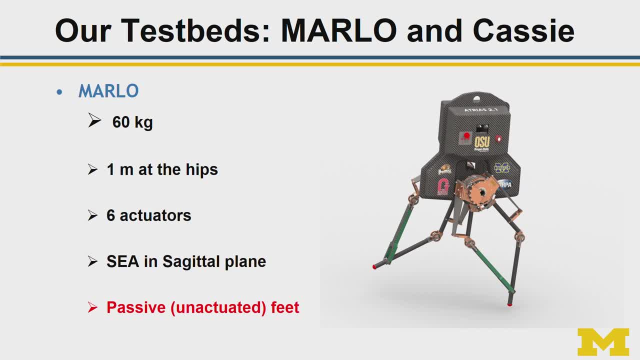 software, Getting it into the hands of companies that will put it on devices that help people. Today, we'll be talking about Marlo. This is an Atrius series robot that Jonathan Hurst built, So this is a program where Sung Bae and I were once upon a time supported by DARPA, until they took 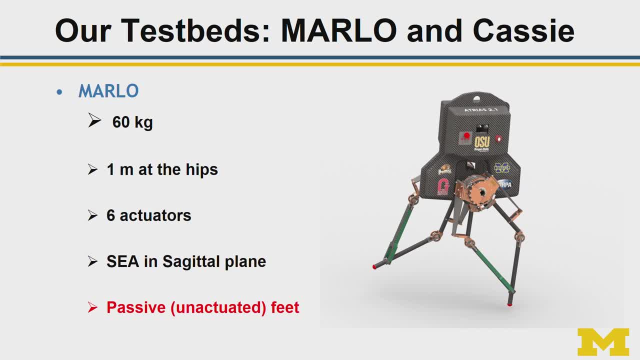 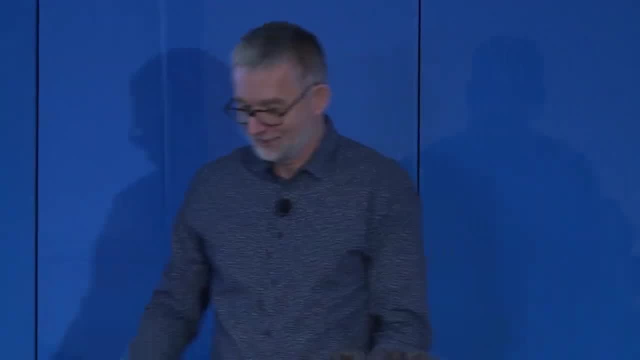 away all of our money so they could run the DARPA program, And we're going to talk about that in a little bit. So the idea is that we could run the DARPA robotics challenge Right? Sung Bae, Pretty much true. So we had to- all of us- rush the design cycles and out of that rush design cycle. 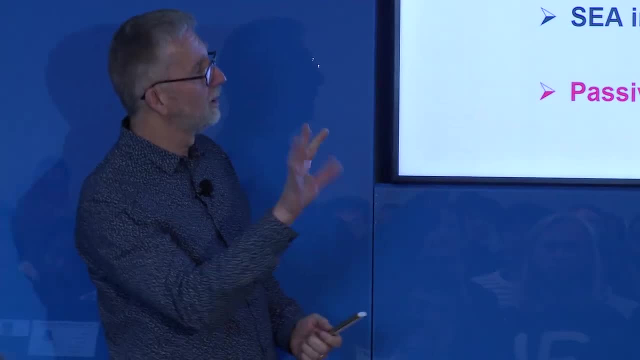 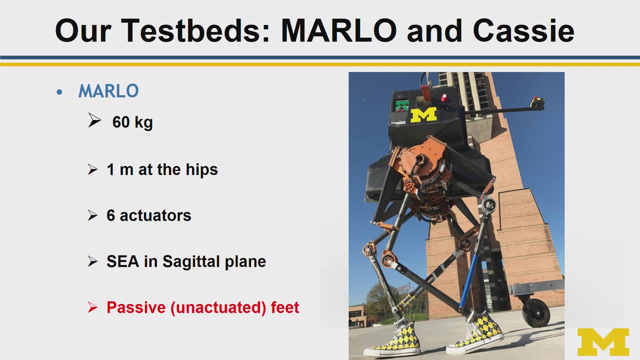 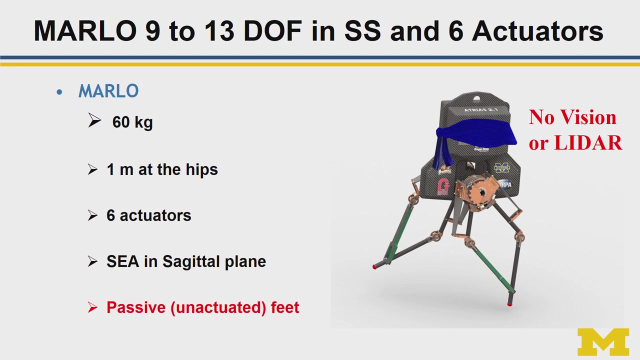 came Atrius, So it weighs about 60 kilograms. It has a two degree of freedom hip, So the yaw motion is missing in the hip. We can also put shoes on it, So mostly we will. it has blades but it looks really nice in these Michigan shoes. 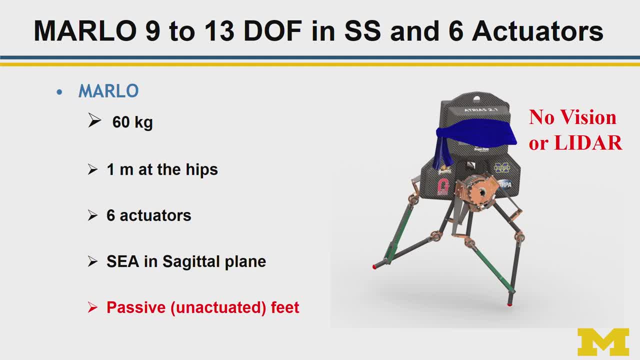 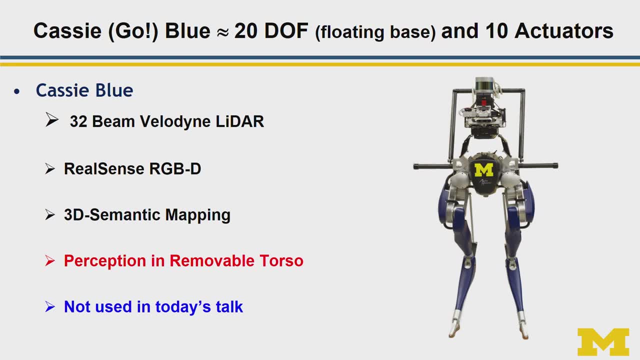 But there's no vision, or LIDAR are on Marlowe. It's completely blind walking. Now this is CASI. If you were here earlier and seeing some of the 3D semantic work, we put a torso on CASI. 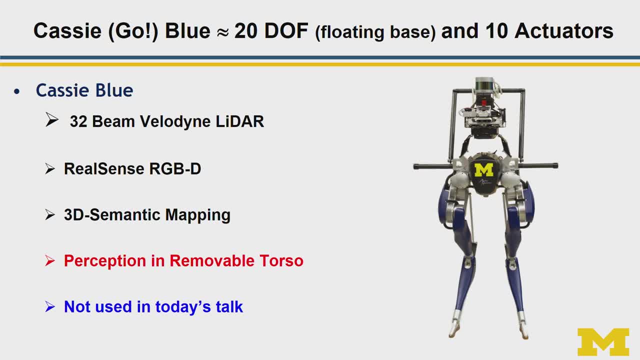 It weighs 11 kilograms. CASI is 30 kilograms roughly. The torso is completely unprotected. So when we use the robot with the torso we have to use a safety gantry. It's just too much time to repair it when it breaks. 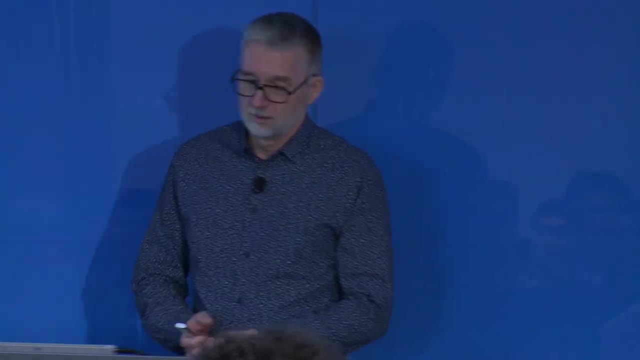 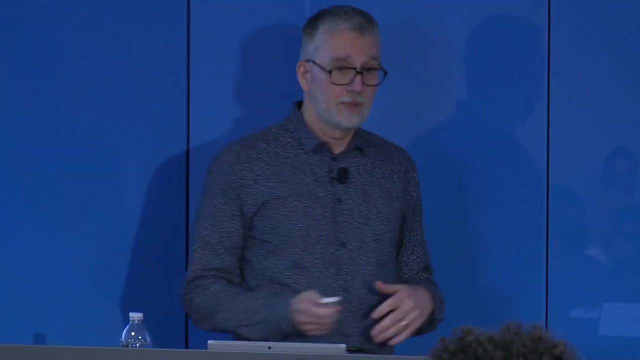 Otherwise, the robot's fairly robust And if you were in here earlier she was falling down all the time. Everything is completely fine with that. OK, so that's my warm-up act. We'll get down into the meat of the seminar. 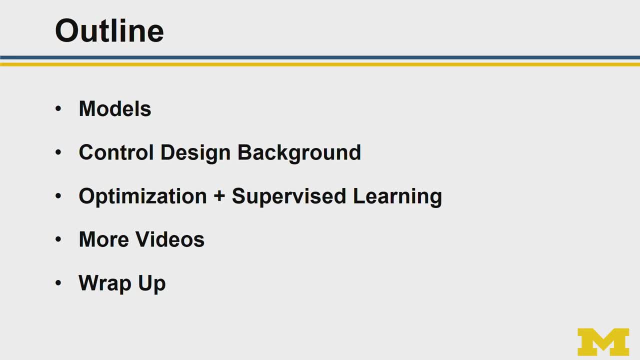 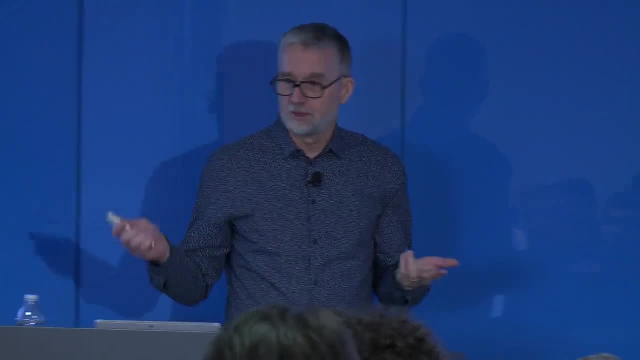 We'll talk about models, how we've done control And so you can see what's new that we're bringing on. And if there's time, we can always show more videos. Everybody has fun with videos. Then we'll wrap up. 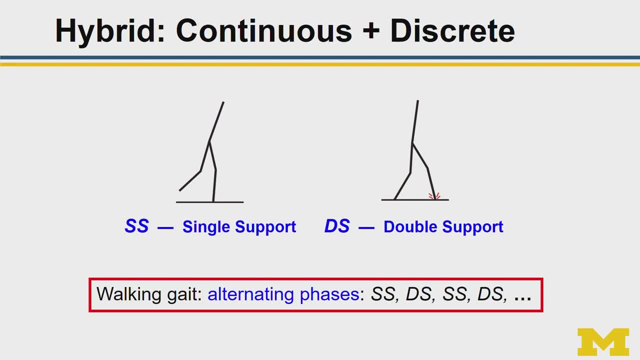 OK, so bipedal walking. You have phases where there's one leg on the ground and phases when there's two legs on the ground. So one leg on the ground we call single support. If the foot's not sliding, then it's. 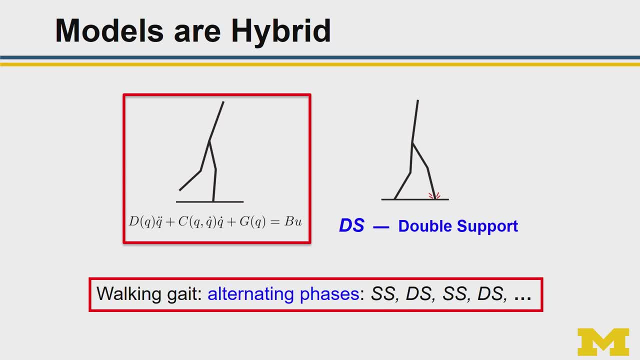 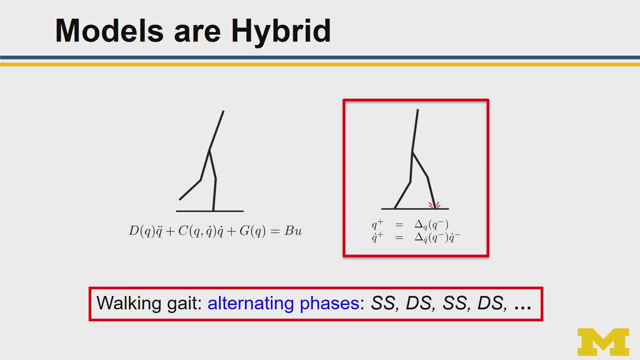 the standard robot equations. You can write them down in the pin form here. You can do floating base. That's your call. Now, when the leg that's not in contact comes forward and impacts the ground, You've got a decision to make on how to model that. 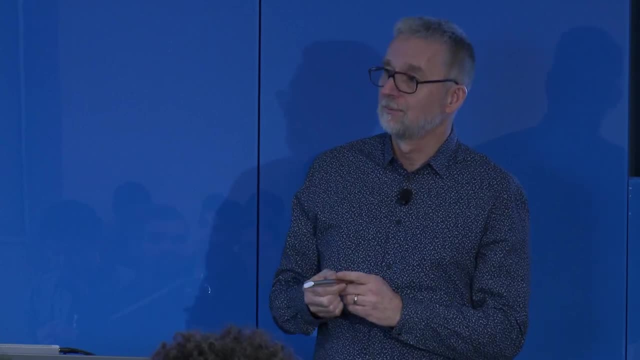 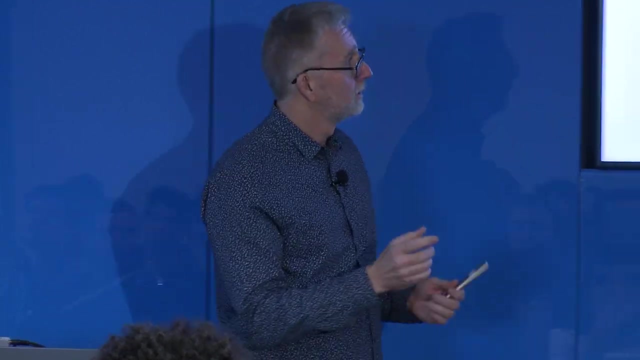 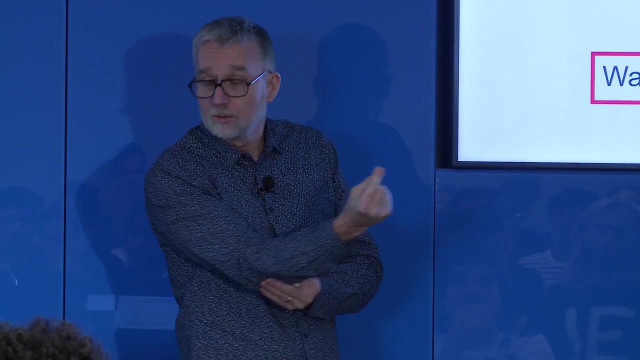 That impact lasts about 20 to 30 milliseconds. So do you want to model it as a stiff compliance, Or do what we do, which is what many in the community do? You take that short period and you shrink it to zero And you turn that force into an impulse. 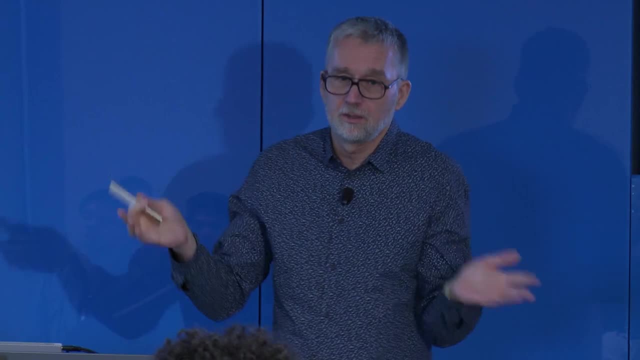 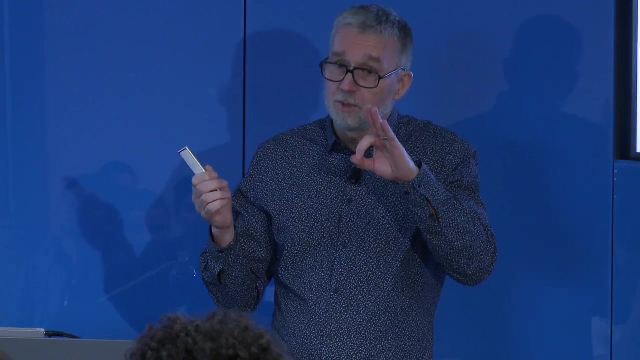 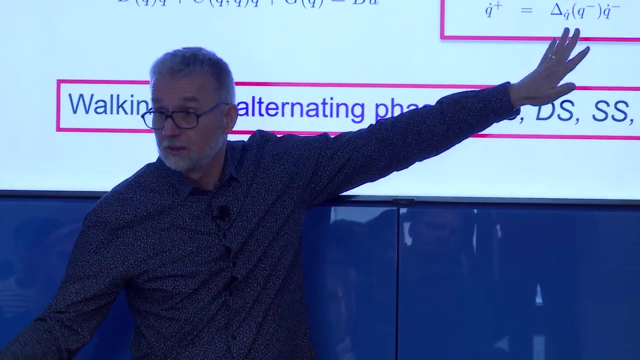 Now, if you have an impulse in a second order linear differential equation, just use your Laplace transform You'll see the position stays continuous but there's a jump in the velocity. So that's what this is: an algebraic representation of that in a nonlinear setting. 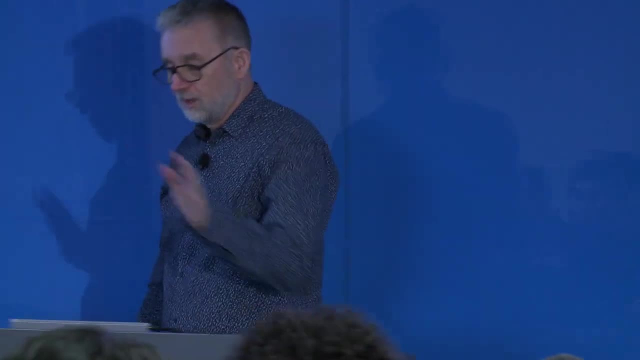 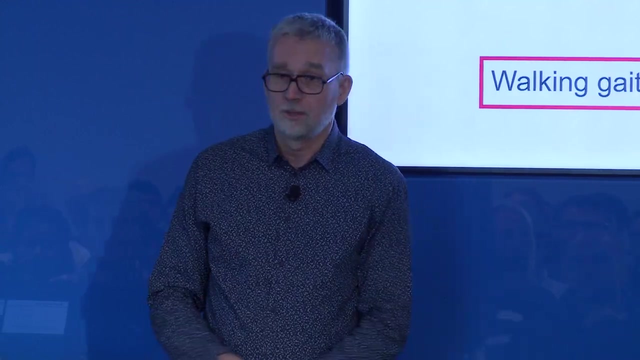 So that's the impact map we use, And the reason we do that is because if we model this contact as a spring, it's very different. in the carpet It's very different. out on the tile It's very different. on sand, It's very different. 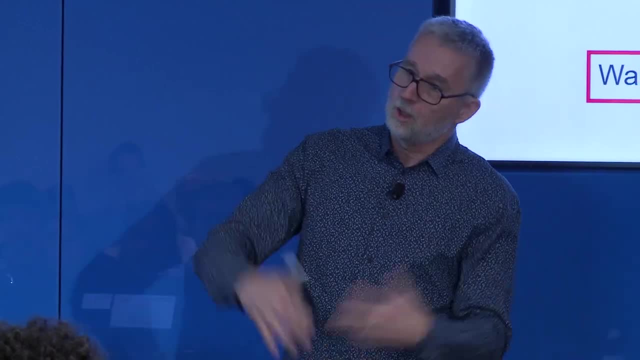 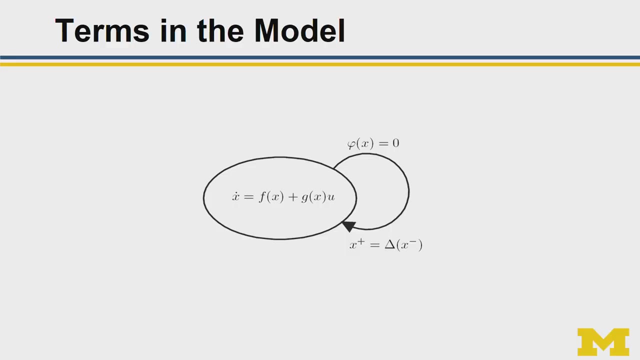 You introduce a whole slew of parameters which makes your model less accurate than if you just use this crude approximation. So that's what we do. So you put it together and you get a hybrid system. It's just a nice Lagrangian. 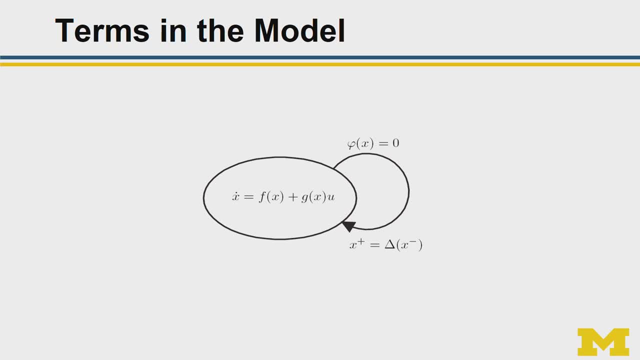 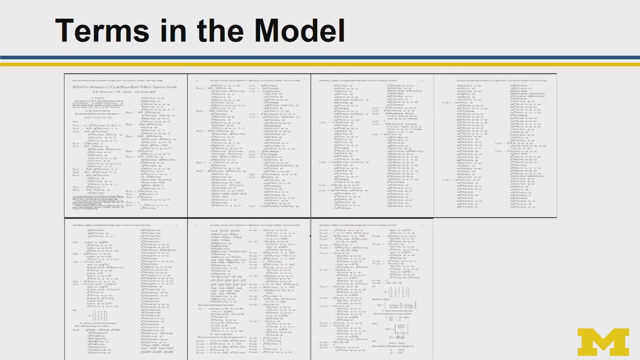 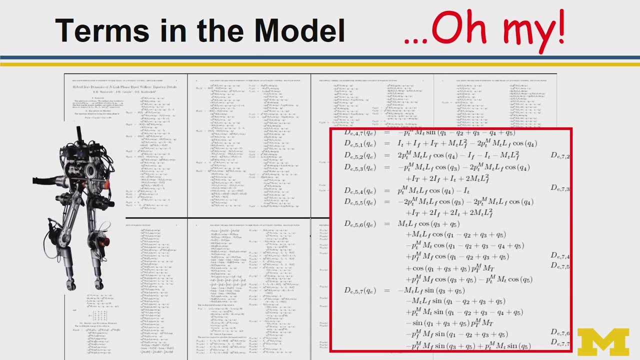 The foot contacts the ground. You have the reset. Maybe you should have two loops, because you have two legs here, left and right. This looks extremely innocent. How could this be hard? Well, the problem is you open up the equations And that's just for rabbit. 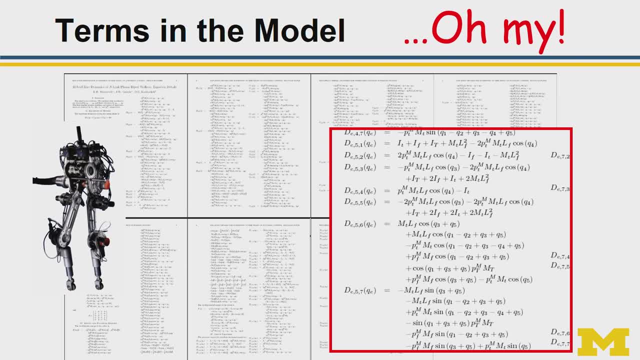 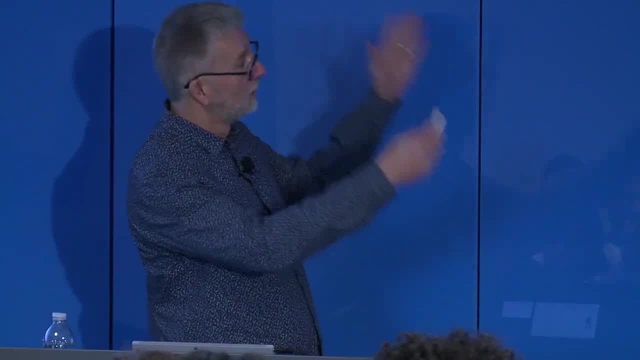 So it's 10 pages of 10-point font And the exoskeleton I show you walking would be about 1,000 pages at 10-point font. So the bipedal community when I came into it was just going like, ah, my hair's on fire. 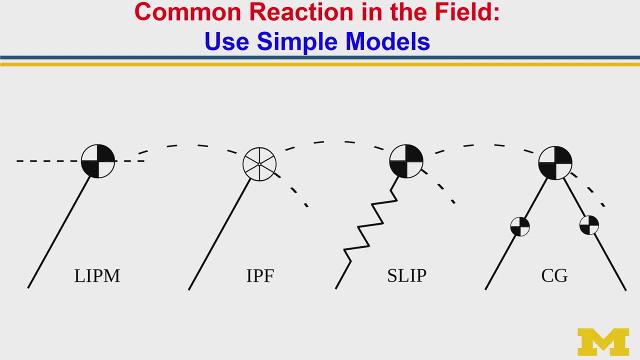 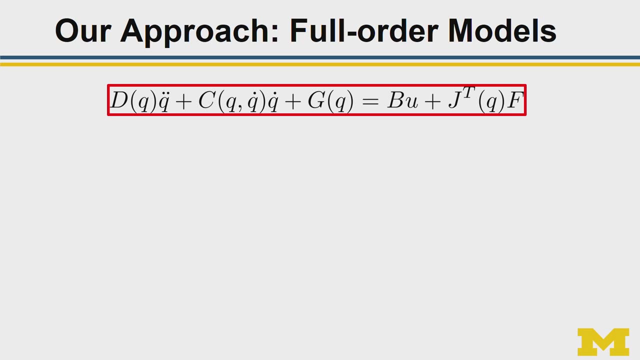 I can't handle this, And so everybody is using these simplified pendulum models. So linear inverted pendulum model: you keep the center of gravity constant. This is flywheel, Spring-loaded, Floated inverted pendulum model From the very beginning in my group. 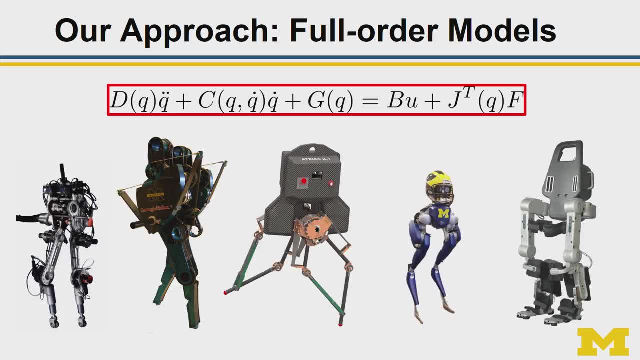 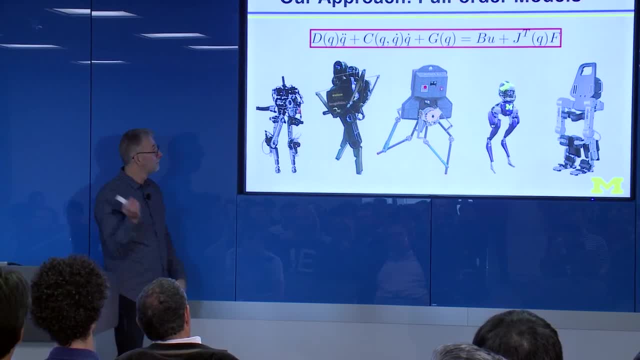 we've been using the full-order model. Whether it's floating base or pin doesn't really matter. So we started that on this French robot. rabbit: It's planar, removes the lateral dynamics. Mabel, also planar, but has huge springs. 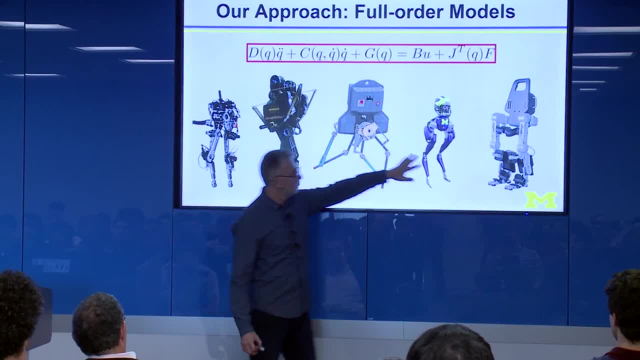 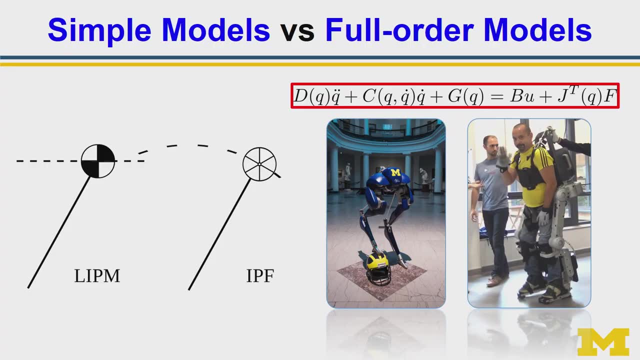 We're really dealing with compliance. This is now 3D, 3D and 3D. So we've kept true to using the full model, And the reason I do it is because on these robots, it's the constraints that make it work. 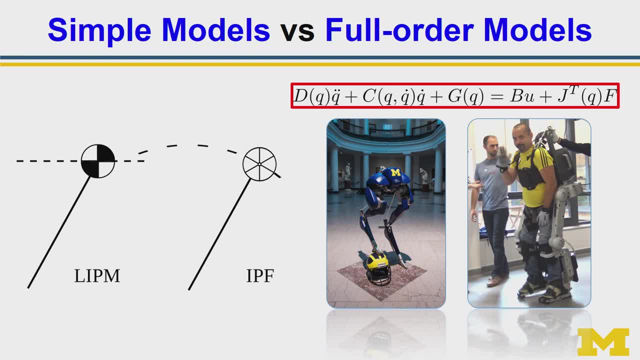 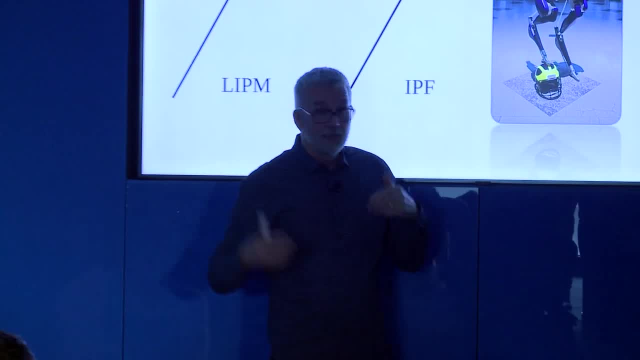 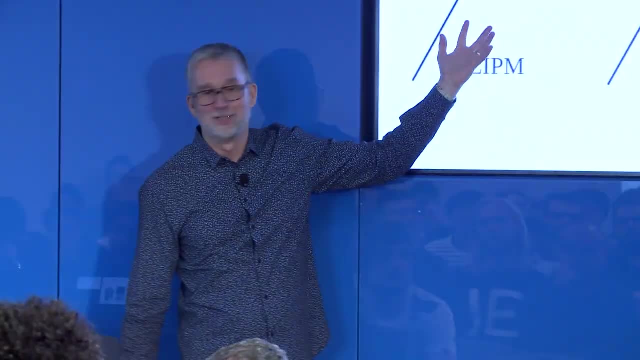 If you understand the torque and power limits at the joints and the workspace limitations and you set that up in your trajectory design problem, then you get things that work. But I don't know how to take those joint limits and represent them over here. 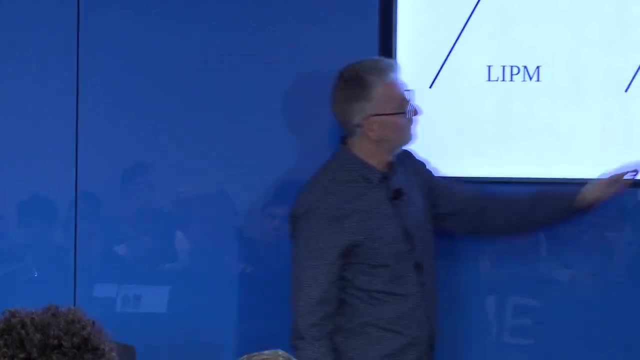 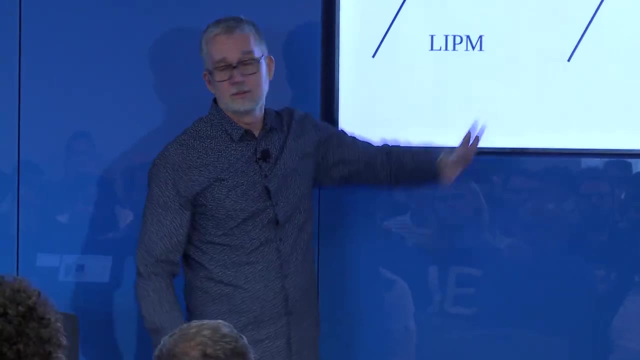 OK, I don't see how to do that, And so we work. We work directly here, So that's just why we do it. There's others who really like to work with this, And I'm glad that we're not all doing the same thing. 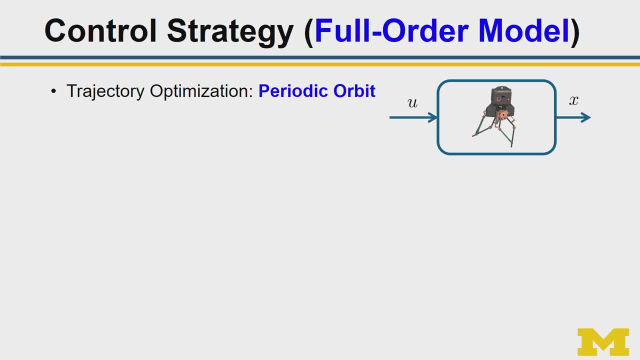 But that's just the approach we take. Our basic tool starts out with trajectory optimization to find a periodic walking motion, So we'll set up a cost function. The trajectory is parameterized, So alpha is a set of spline coefficients or something, And we'll do energy per distance traveled as a cost. roughly. 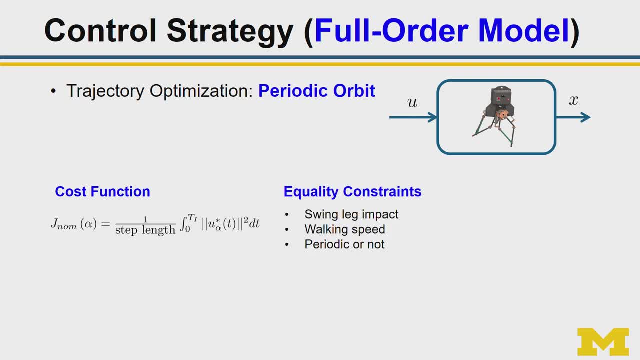 OK, Then there's some equality constraints on the walking speed. Maybe we're periodic, Maybe we're not, But, as I was saying, this is the meat of the problem. It's the inequality constraints that make the feasibility of mapping your mathematics onto the real system. 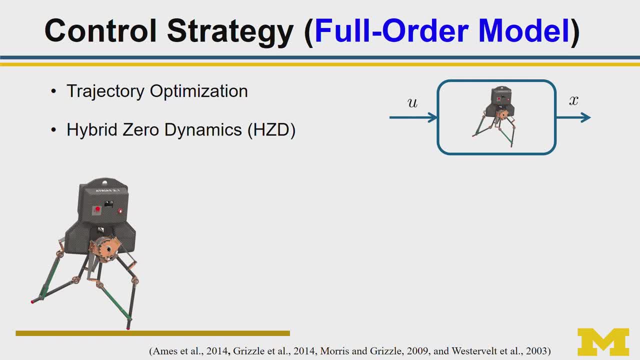 Now there's one other step we go to. So that's just for getting the periodic walking. OK, So you can take one periodic orbit. Can you get a controller from that? So I think this surprised people, that you can take one periodic orbit and from that extract a controller. 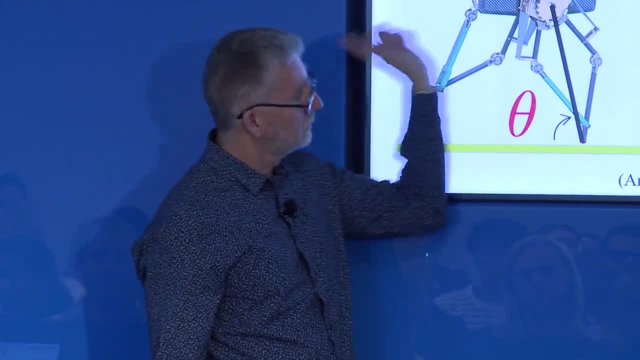 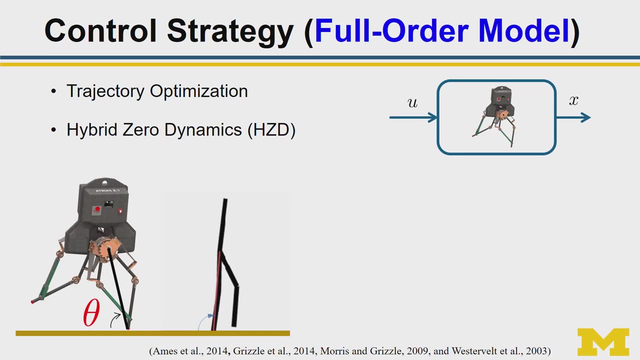 So this is what the method of virtual constraints does. If you have a robot and it's walking, say, forward, there's a natural phase variable that you can use for timing the motion of the other limbs. So you don't have to use time. 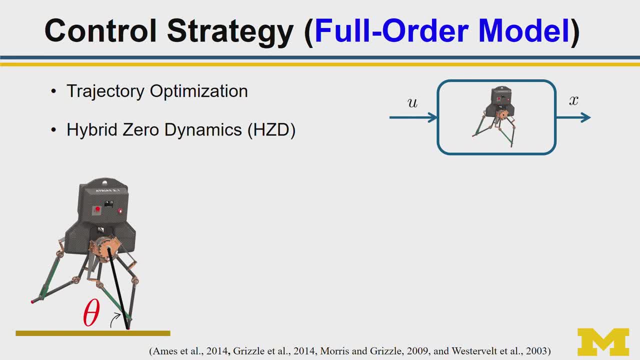 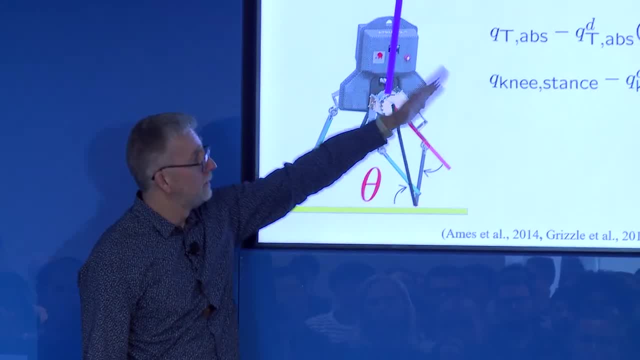 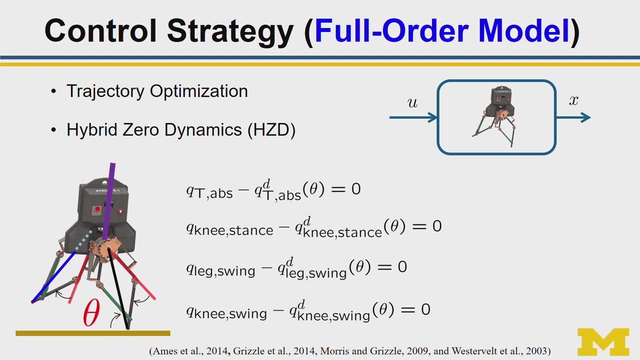 You just have to use the spatial variables- We call that our spatial phase variable- And then what we'll do is we'll program the evolution of the torso angle, the knee angle, the hip angle, et cetera, as a function of this spatial variable. 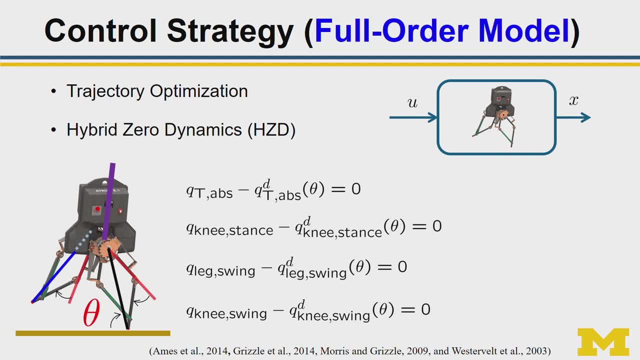 So these are called virtual constraints. You write down: y equals this quantity, You drive y to 0. And you've got a feedback control problem. So the feedback control problem is going to be the same as the one that we have And then implement it on the robot. 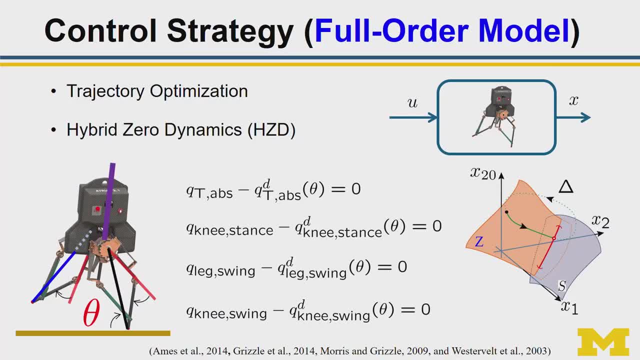 by driving natural outputs represented by these formulas to 0.. And so, if you're successful in that, you've created a set of constraints that give you a lower dimensional problem. It's somewhat analogous to taking a floating base model- high dimensional- and then putting the contact constraint. 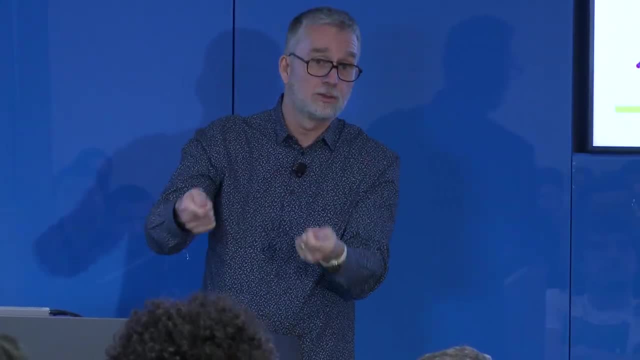 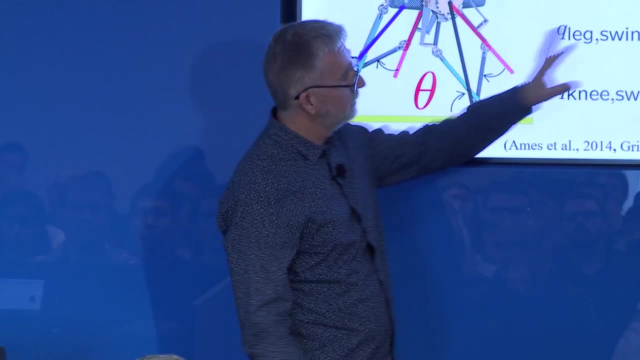 OK, If you do that, you get another Lagrangian system. OK, And you could start the design right there. These are not physical contacts. The actuators are actually doing work on the system. So, in general, the dynamics on this lower dimensional thing. 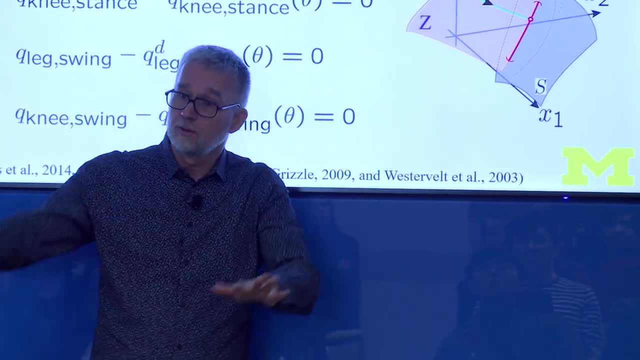 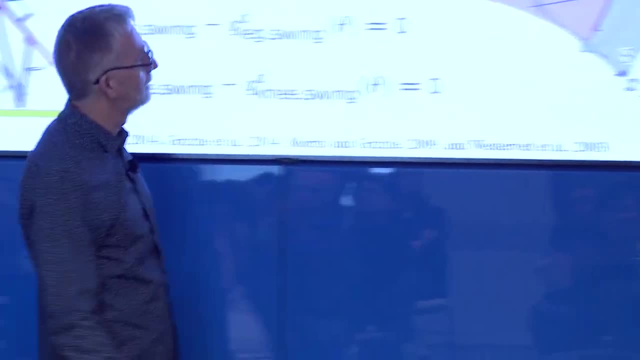 are no longer Lagrangian. OK, so it's not necessarily that there is a pendulum model corresponding to this, because those are Lagrangian, They're Hamiltonian mechanical systems, But that's the idea. You create this invariant surface. 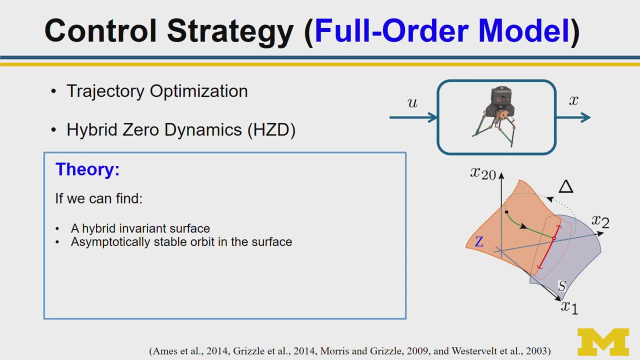 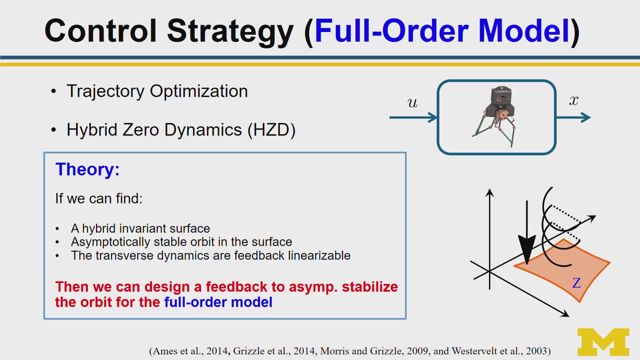 And the theorem says: if you can do it and you can find an orbit within there that's exponentially stable and the transverse dynamics are sufficiently nice- the ones off the surface- then the feedback will result in the full order model being having a locally exponentially stable periodic. 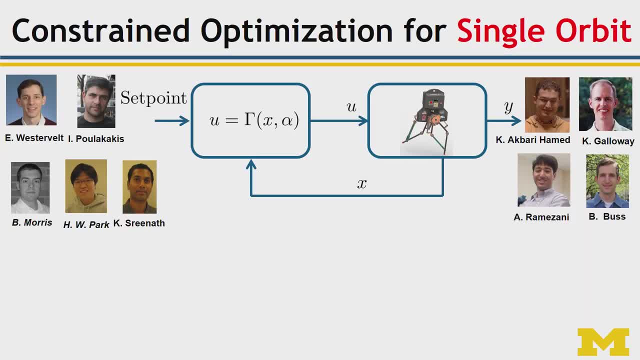 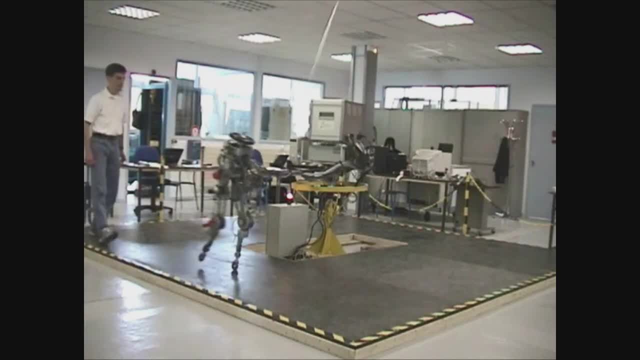 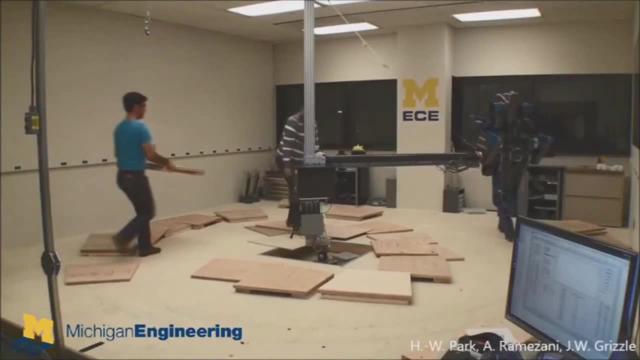 orbit. So those are the basic ingredients. OK, that got us a long ways. These are some of the students who helped develop that. So there's Rabbit with an extra mass and, withstanding disturbances, Mabel, that's 30 centimeter drop off there. 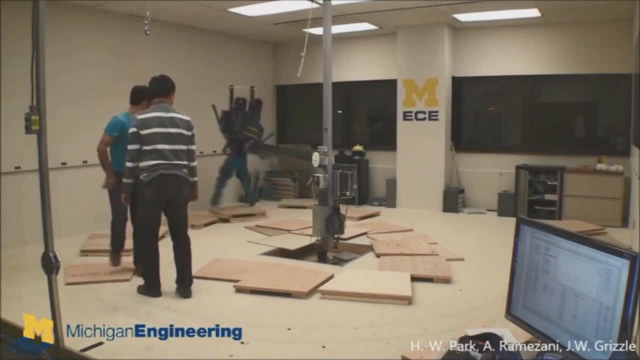 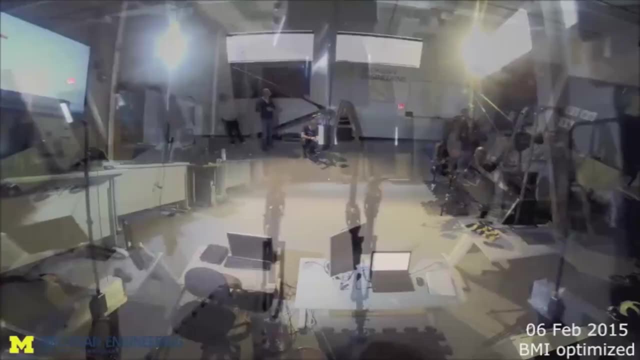 There's Haywan Park. You know him, Alireza Ramazani, who's now at Northeastern Just being mean to Mabel. She's blind. They're putting blocks in arbitrary places. I mean they're just being totally mean to the robot. 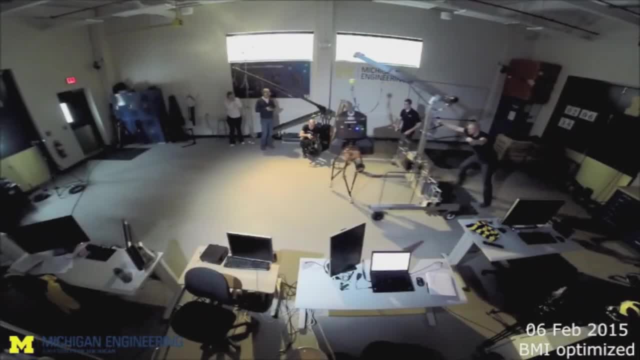 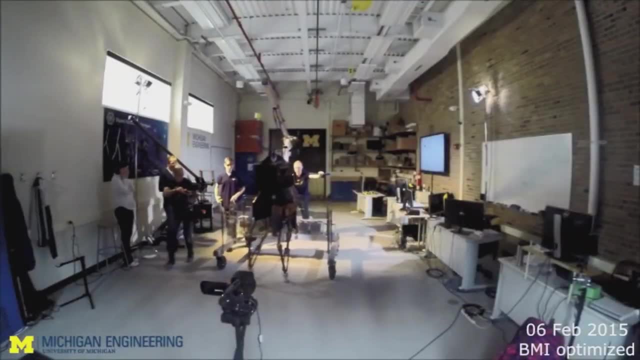 OK. So now we get it on a 3D robot, Atreus, And in the lab, even with camera crew present, it's walking. OK, that's amazing. Anybody done a demo with a camera crew and everything just fell apart. 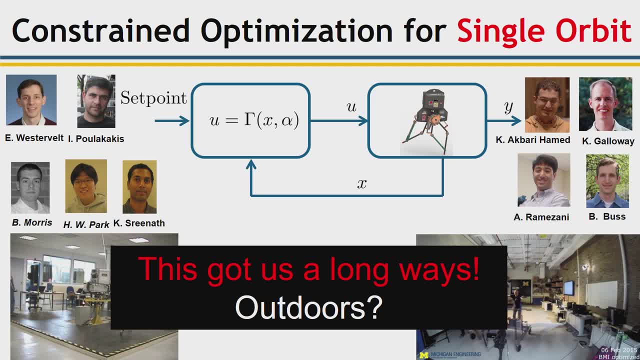 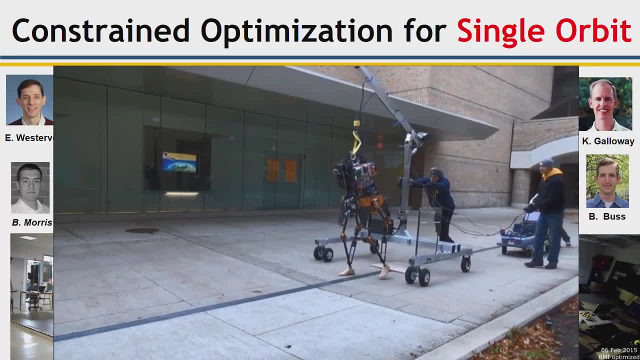 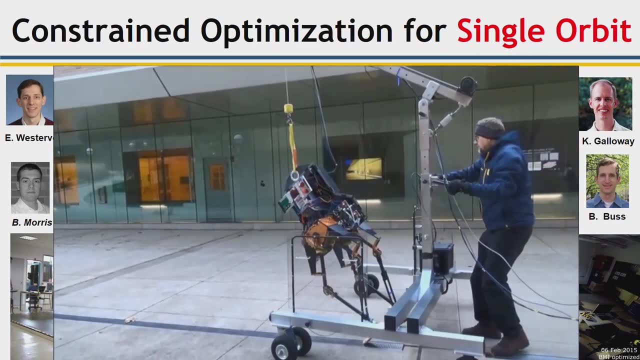 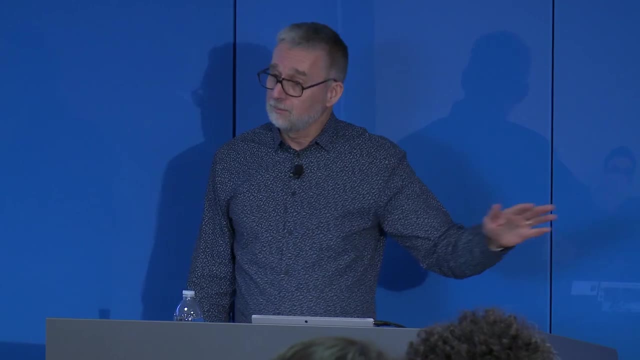 Yeah. so those ideas got Atreus, which our copy, we called Marlo to walk. But here's the robot outdoors. It's Michigan. Those are harmonic drives. The stiction got higher, et cetera. The outdoor sidewalk is not perfectly flat. 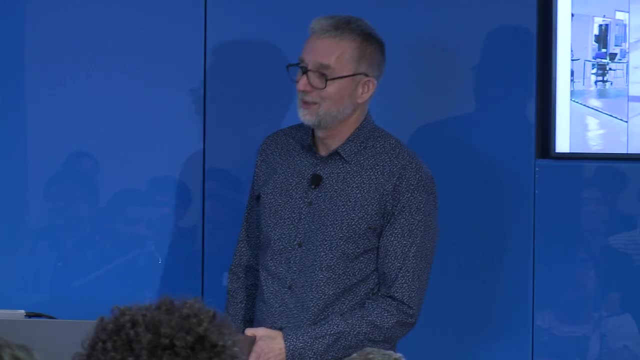 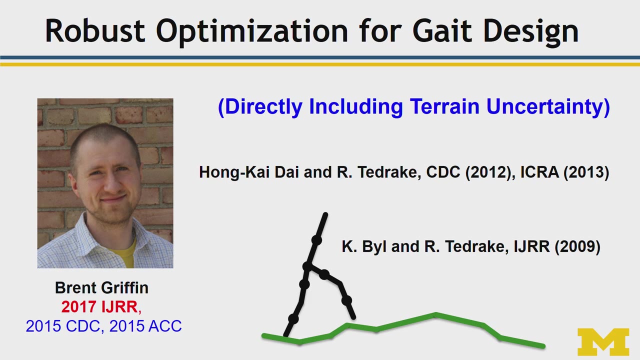 It failed miserably outside of the laboratory. OK, So got us a long ways, but it failed miserably. So, Brent, who was working at the time as a PhD student, I had read a few papers by Russ's group and especially the work by Hongkai Dai. we found inspiring. 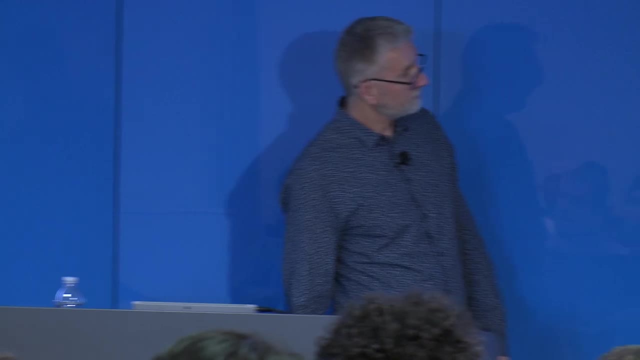 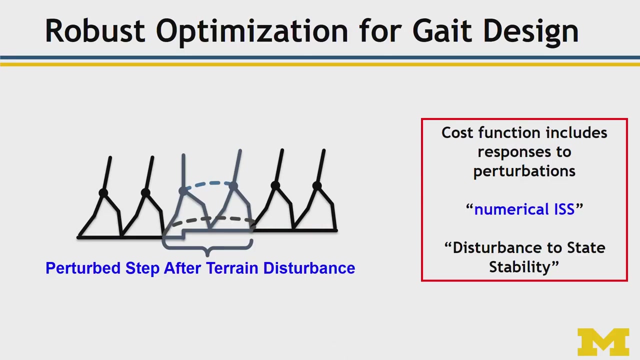 And so Brent took. He took the idea and he did the following. He said: I'm going to design a controller that is a numerical version of Eduardo Sontag's input to state stability. if you've seen that work, It's a way of doing robustness. 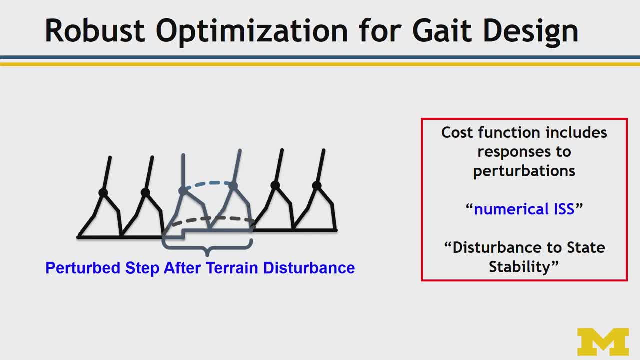 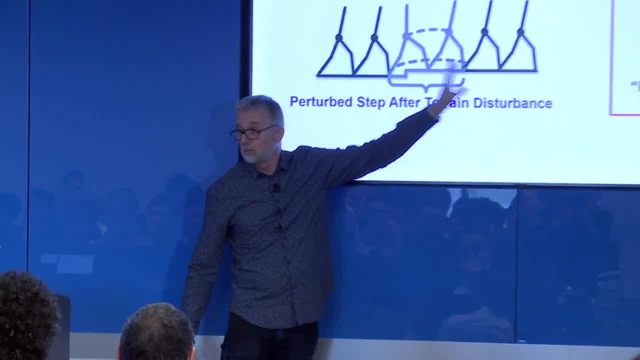 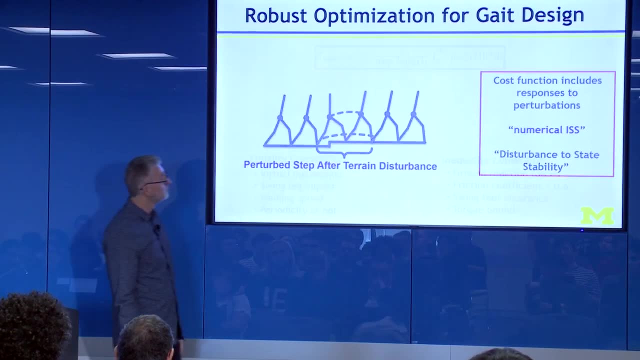 OK, I'll explain it to you this way Before. we're only optimizing the periodic motion and not taking into account how the robot responds after a disturbance, And Brent said I need to take that into account in my controller design. OK, 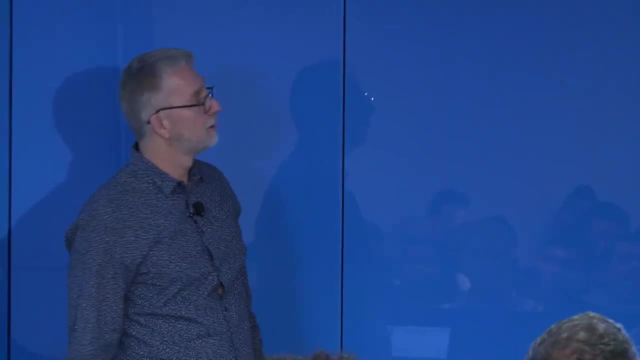 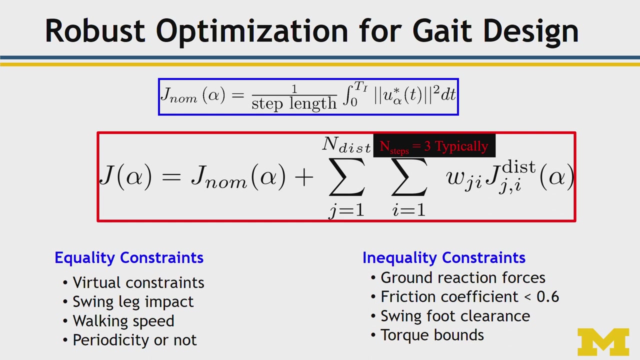 So we set up an optimization problem that had all the basic ingredients for the nominal motion, And then he adds in a set of disturbances. He can have a number of them, He can look at a number of steps And then the weights would be well. 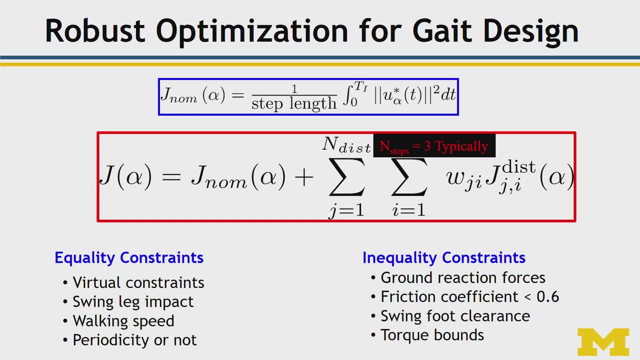 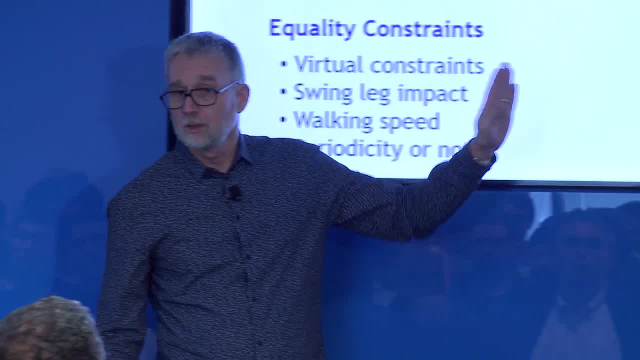 right after the disturbance. you don't want the robot to act like it's near the periodic orbit. You want it to have the transient to adjust and start correcting. OK, OK, But as you go more and more steps in, you want to penalize that more so that you come back. 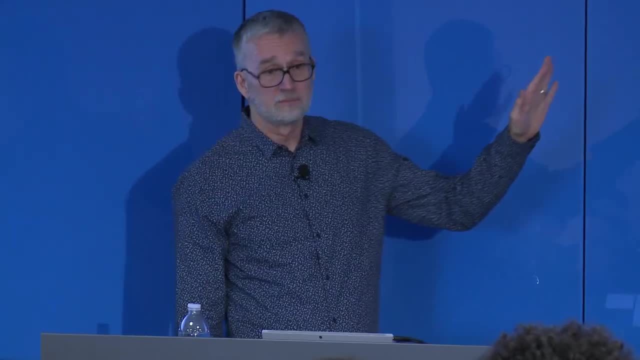 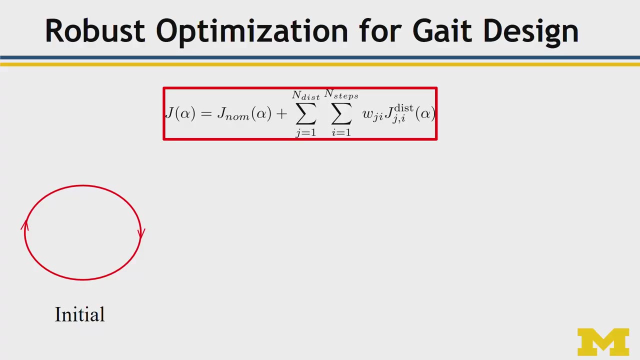 to the periodic motion. OK, It's a very simple idea Graphically. so this is your nice beautiful, energy efficient orbit that everybody wants. OK, And then you challenge it with disturbances, And then you're pushing off and they're not coming back. 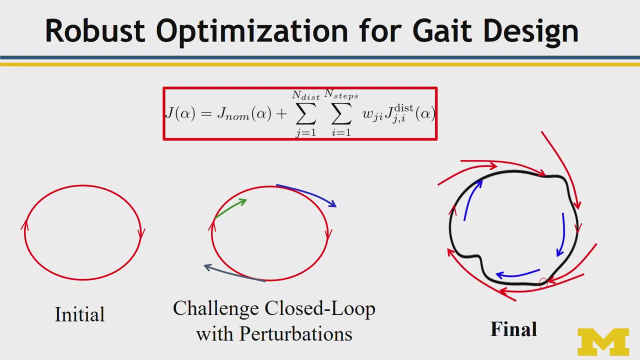 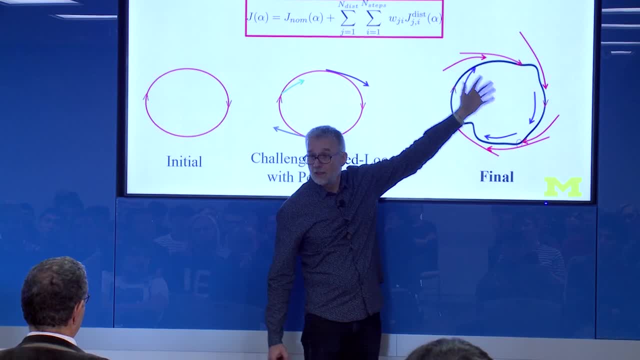 OK, So this is the robot falling down, And then what Brent does is the original orbit. you know, it gets warped in such a way that it's taking into account the disturbances and it is attenuating them. So that's what his cost function was doing. 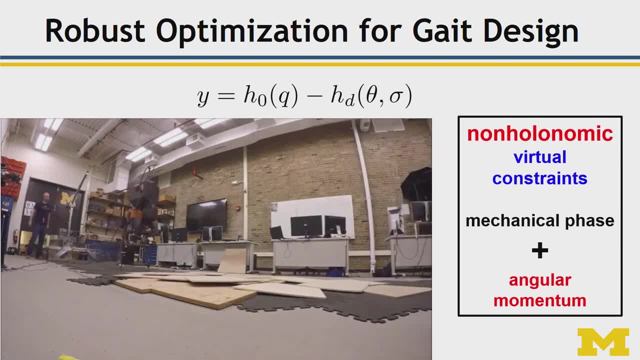 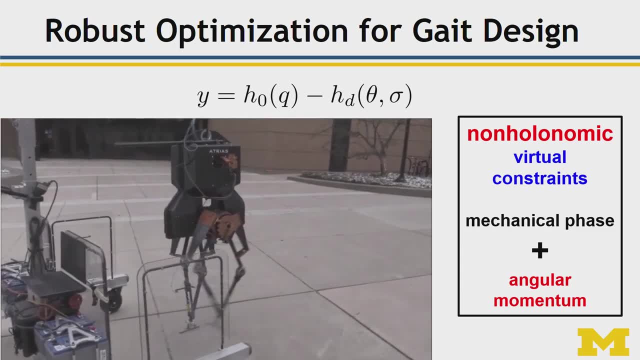 There's Dennis as a young student, as an apprentice, And they just threw him out so he didn't think that Marlow knew ahead of time where those boards were or anything. OK, Just randomly out of the warm lab where the cold Michigan air. 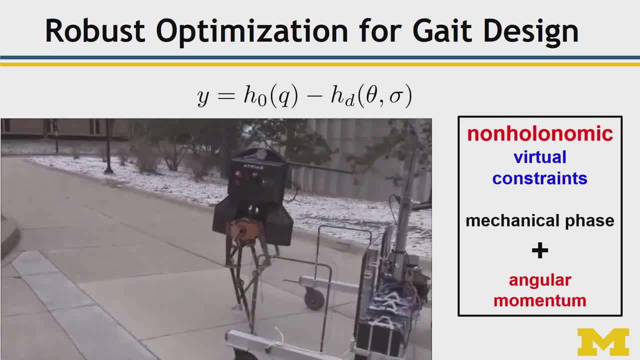 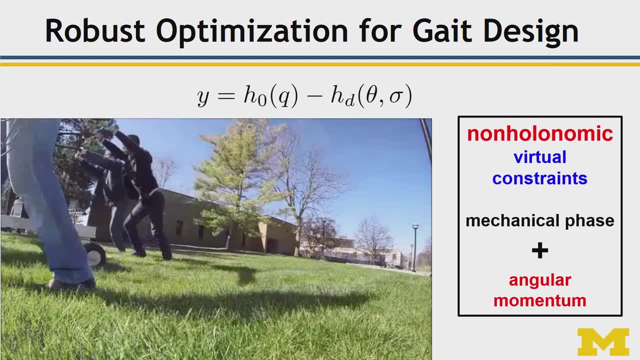 was making the harmonic drives. the stiction get higher and higher. I mean, who knows what the impact map there is right On grass? It was always exactly the same controller, So this was an important innovation in how we were designing controllers. 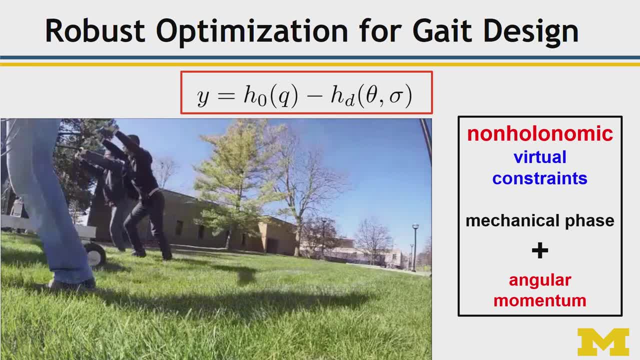 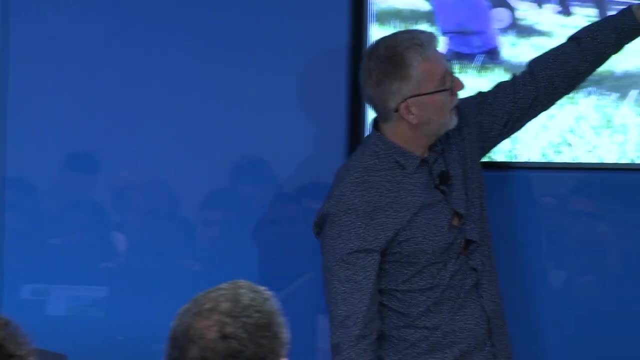 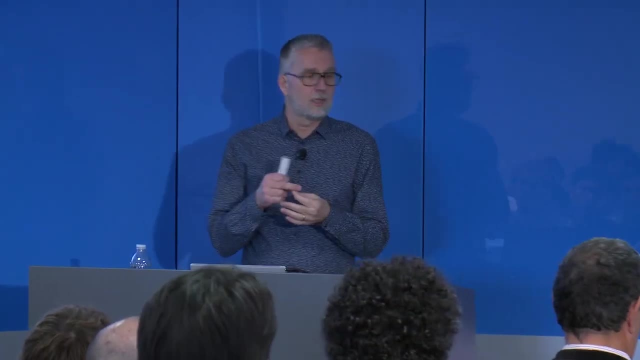 OK. So he was using disturbances to create new initial conditions that the controller had to respond to. So he was designing in closed loop. We'll come back to that. But the other thing he had was he's adding an angular momentum. This sigma here is the angular momentum about the stance toe. 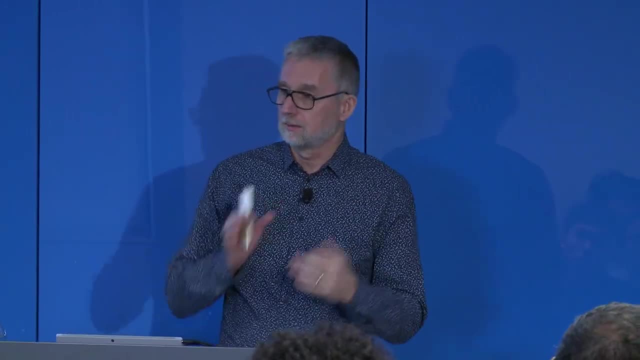 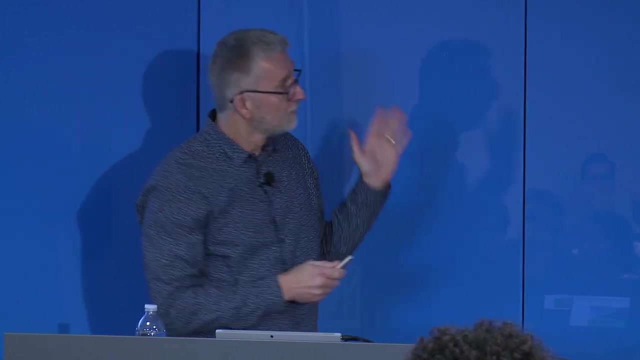 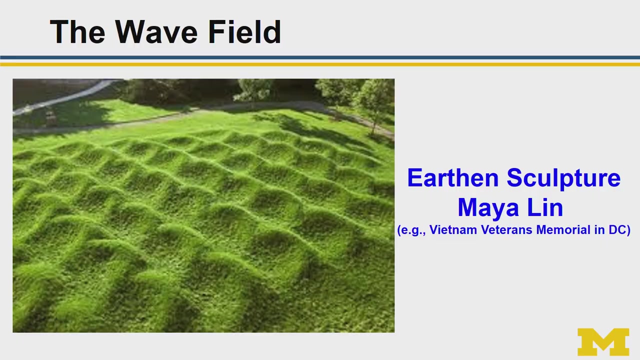 And he'd have components in the lateral and sagittal plane, so into the body motion sideways, OK. So he said, oh, velocity needs to show up in there somehow And did it in a way to preserve the second order nature. And he said, oh, it's a very important part of the structure. 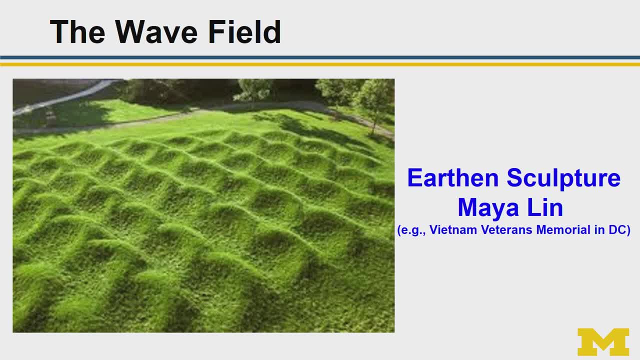 of the dynamics OK. So that looked pretty good. We could just say, hey, problem solved, We're heroes OK. But my problem has been that at Michigan there's this sculptures by Maya Lin, who did the Vietnam Veterans Memorial as well. 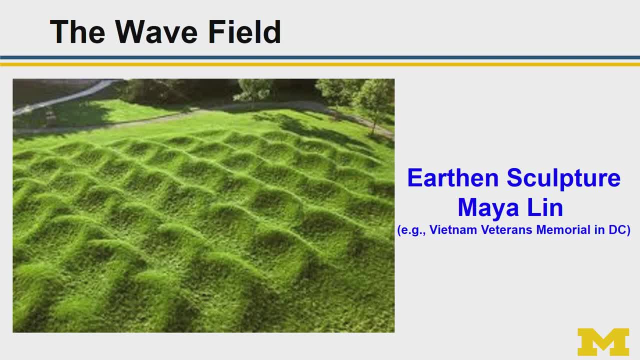 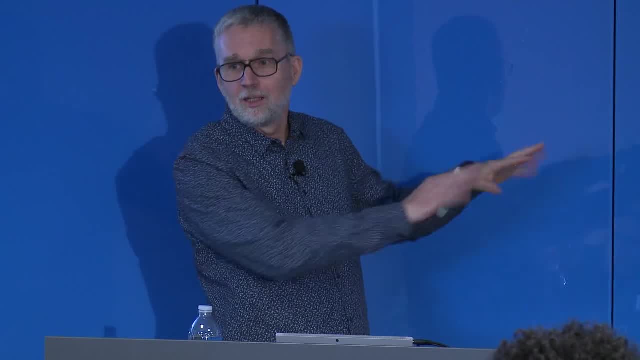 And every time I saw this I would see kids just running across it like it's nothing, OK. So I said, can my robots at least walk across this? And for me it's just been calling to me, OK, So we took Marlo out there. 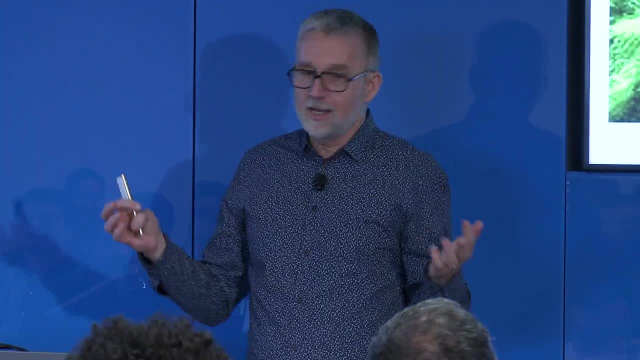 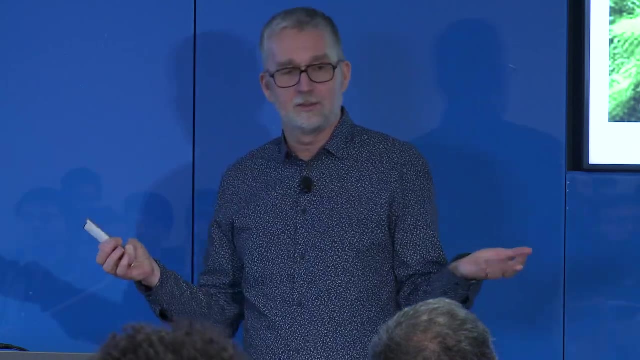 And what happened was the Discovery Channel was filming in the lab And we did all of our usual tricks And then we ran out of stuff to do And everything was going well, that we were ahead of schedule. And they said: do you have anything else up your sleeves? 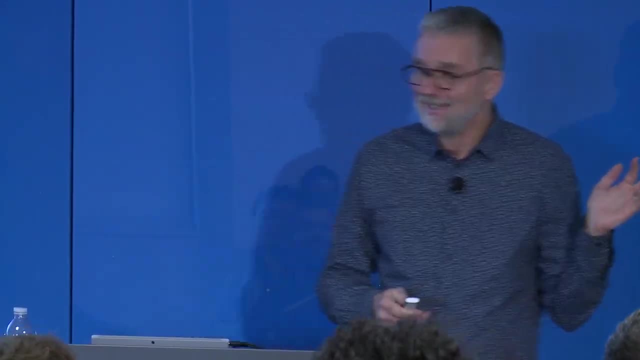 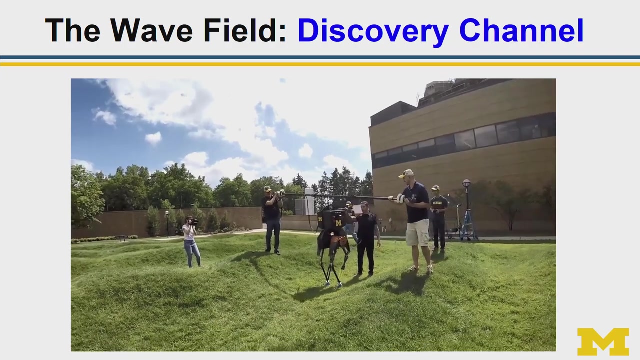 And I said: well, I've always wanted to go to the wave field. You guys up for that Stupid idea, I know, But so we did. Good, There's Brent, There's me, There's our human gantry. 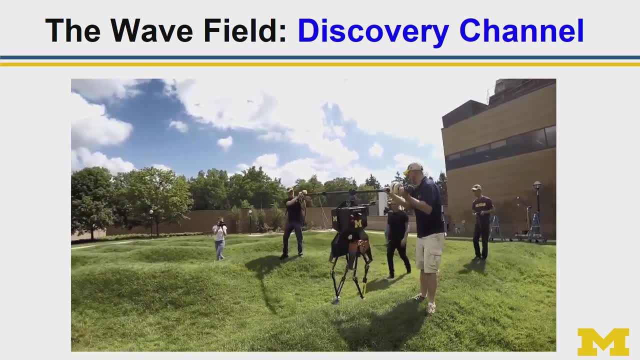 You can see the guy with the tattoos. He's not one of my graduate students. He's way too cool, OK to be a roboticist. Whoa, Whoa, Whoa, Whoa, Whoa, Whoa On camera. 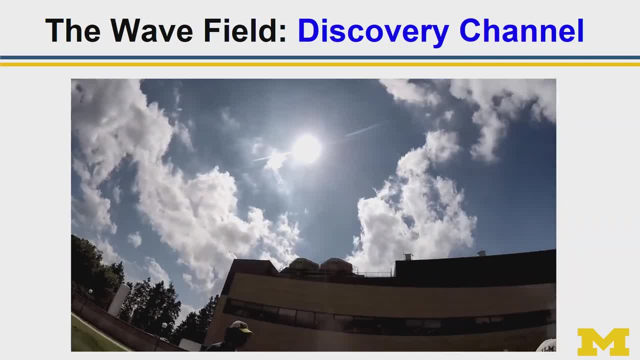 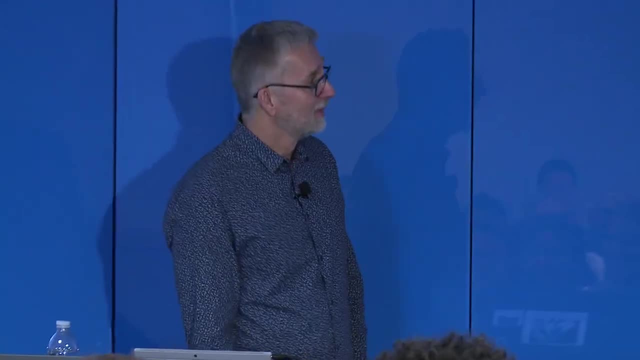 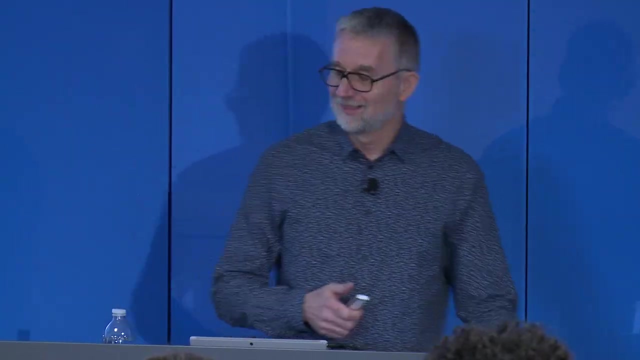 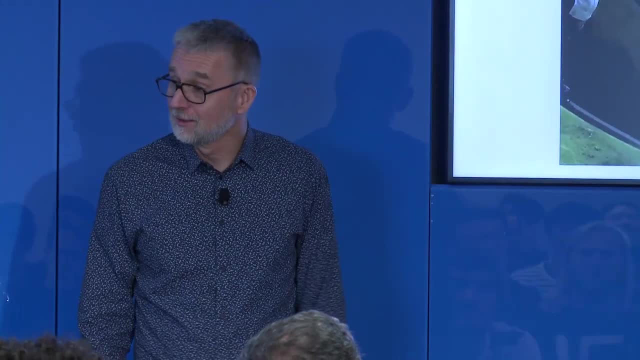 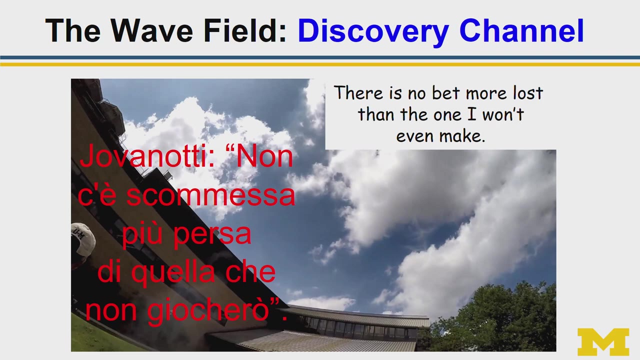 OK, So we failed again. OK, And this is the Giovinotti quote. So he's an Italian hip hop singer. So if you're into hip hop, you want to get the Italian version. And what this quote is saying, that there's 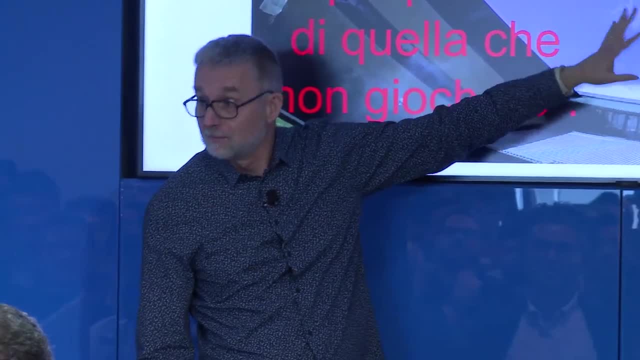 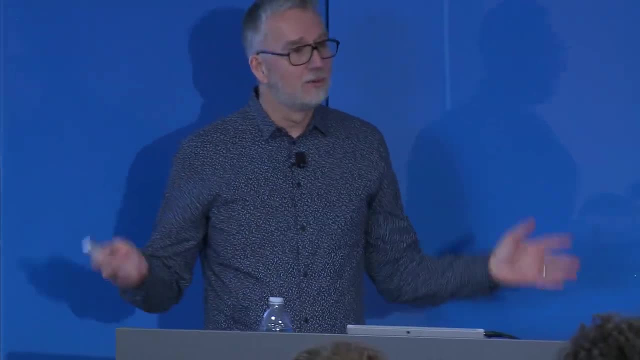 nothing worse than not taking the bet because you're afraid of failing. OK, So we always take those bets in my lab. I don't want to have any regrets that maybe we could do that way field and just weren't courageous enough to try. 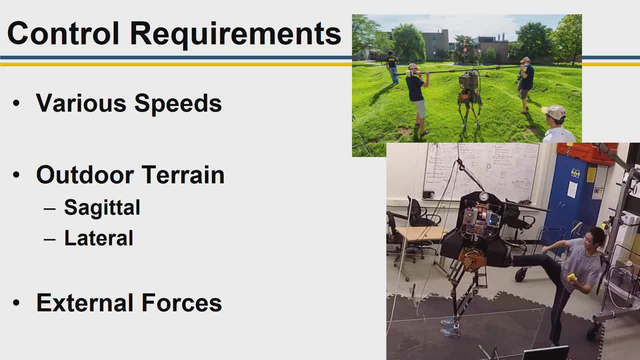 So Dennis saw these failures And so he's getting his act together for the PhD. He's first through his first two years of courses where he has no time. He's learned the lab culture. He sees what's working, He sees what's not working. 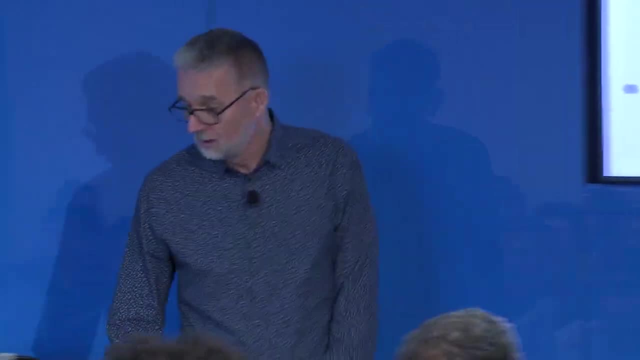 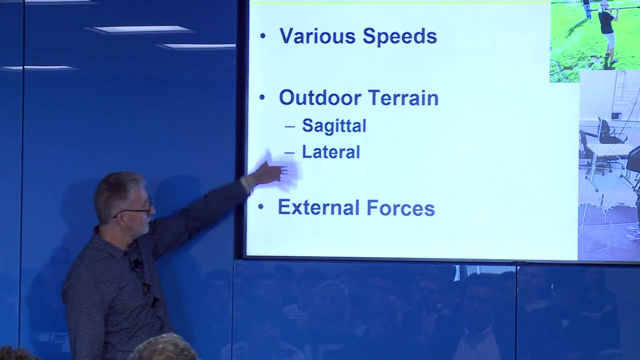 And he decides what he's going to be doing for his PhD in the area of walking And in the end he said he wants to do various speeds, OK, Wants to do outdoor terrain and deal with external forces, And he wants a single controller to work. 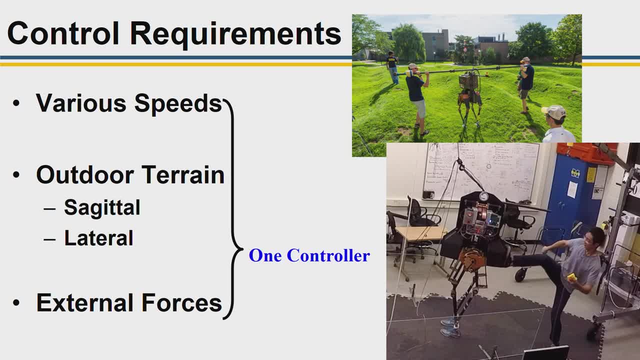 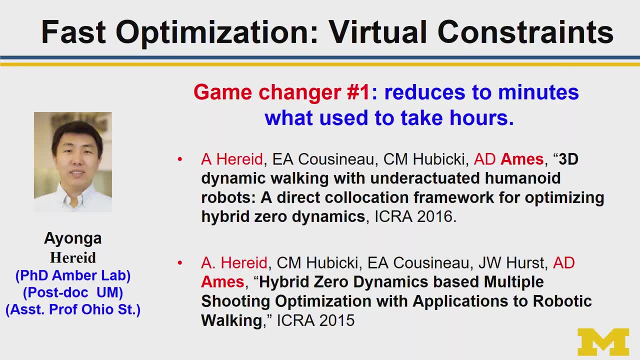 in these types of things. I don't think he wrote it down that clearly When he first got started. I'm sure you've had to kind of coax out of students what they're really after, But that's what he wanted to do. 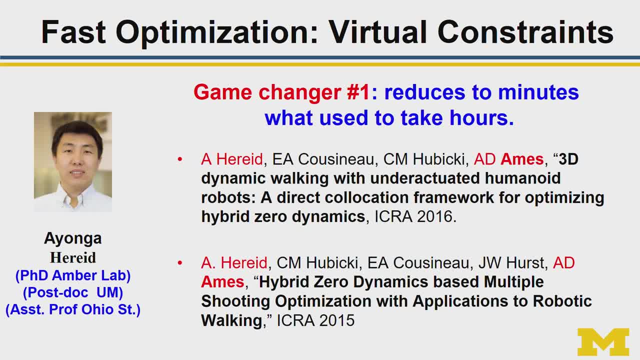 So that's really what I want to talk about now is the core of Dennis's dissertation. Are we doing? well? I'm not speaking so fast, You can't follow me, It's OK? Oh good, So the first game changer was the following: 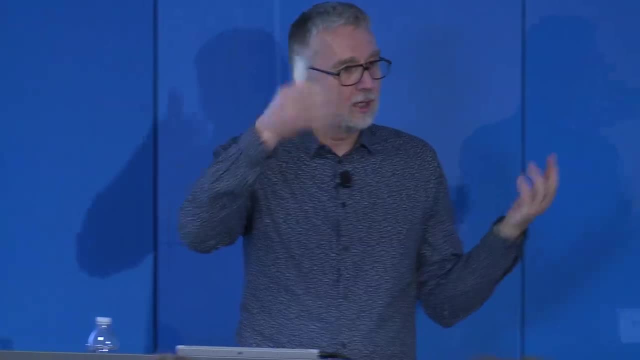 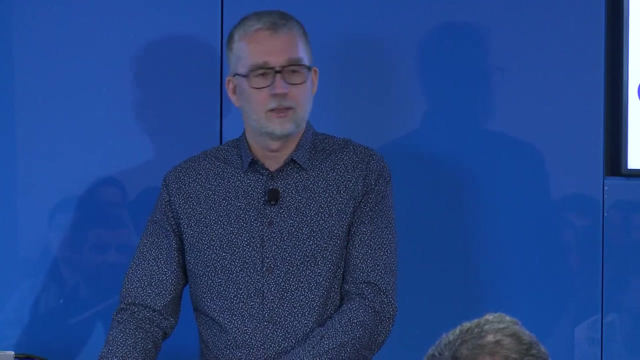 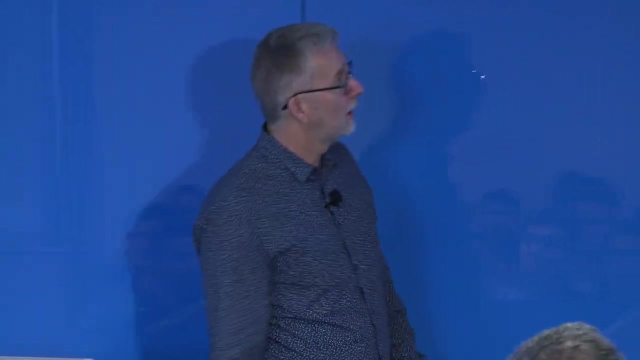 So when Brandt was doing his optimizations inspired by Hongkai Dai, even on that Atreus robot, those codes were running like 11, 12 hours to do a controller. It's not forever, but it seems like it. So it was a long process. 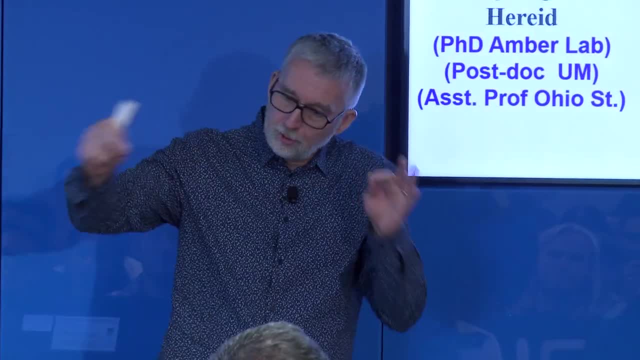 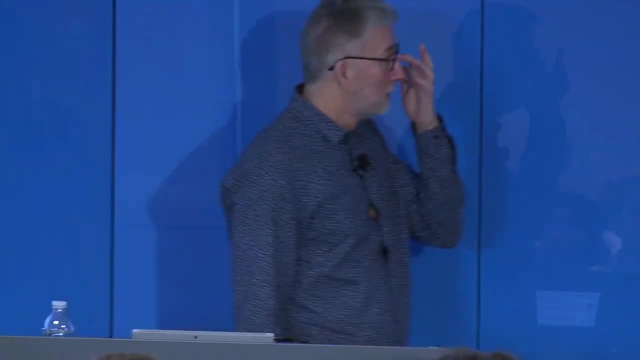 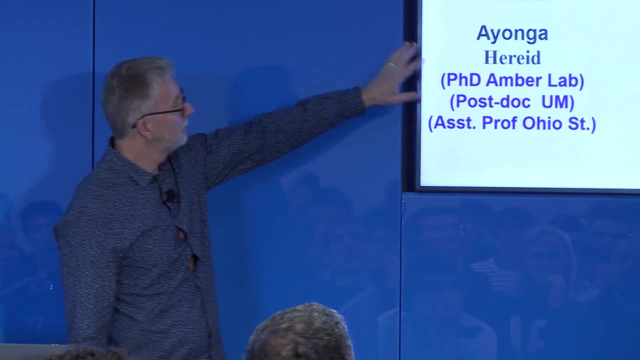 So it was taking us multiple minutes per trajectory, And then we needed many of them to find the response to these disturbances, And so a young guy got it where each of these trajectories can be calculated in seconds now. So he was a PhD student of Aaron Ames. 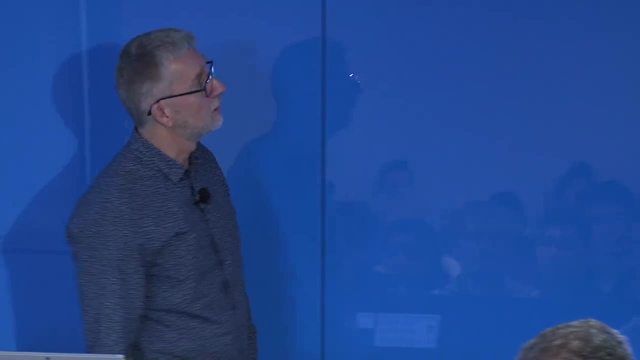 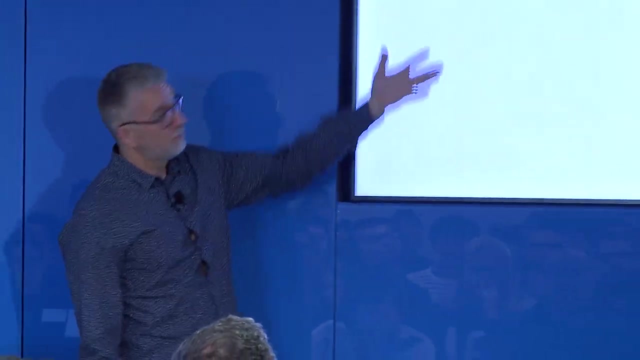 Then he came to Michigan for a postdoc And now he's at Ohio State, So he's game changer number one. He's a really brilliant young man. So we can do These optimizations fast, but we can't do them fast enough. 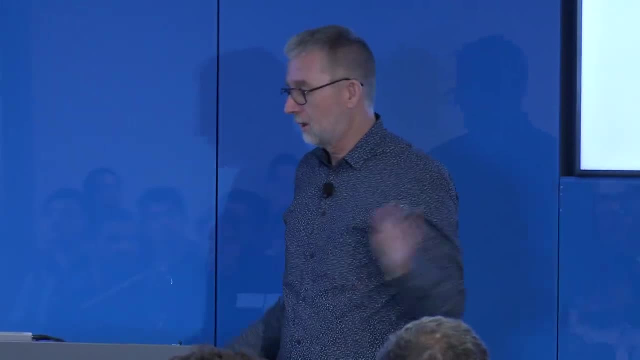 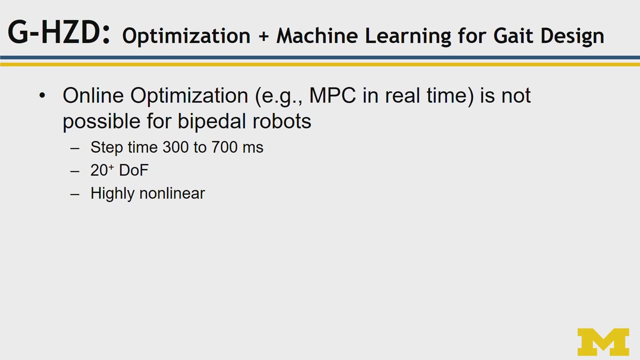 to do them in real time. So there's no model predictive control hanging here. Our step time is under a second And so the optimizations were longer than that. You can't do it in real time And the robot's 20 plus degrees of freedom, et cetera. 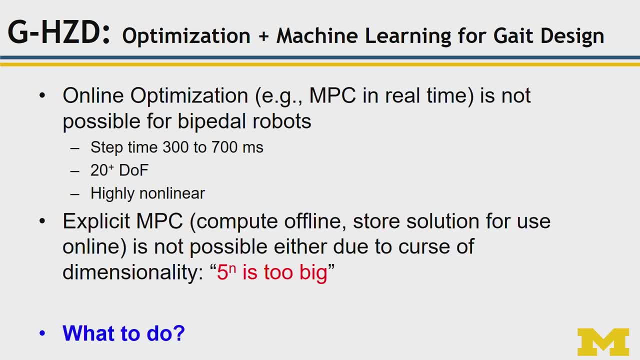 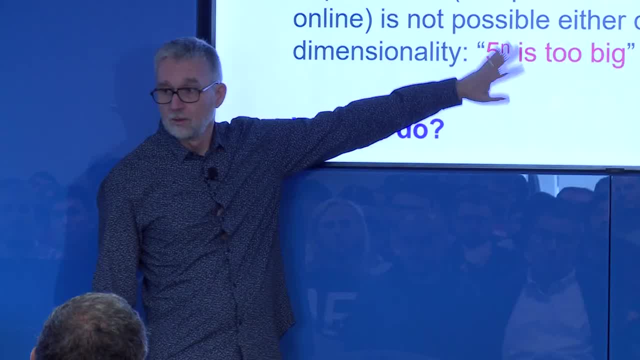 So you can't do it, So you do the calculations offline and you store them right. That's called explicit MPC, And the problem is The number is too big If you only put five samples per dimension and n is 16,. 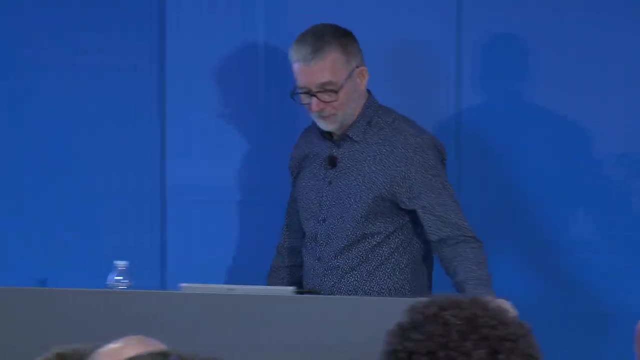 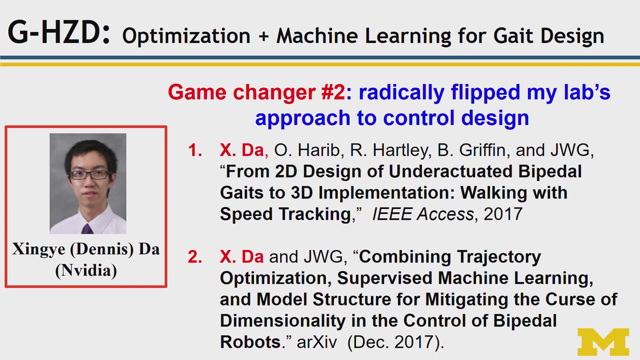 this is over 100 billion trajectories. you have to store Good. So what to do? What to do? So? this is where Dennis came in. So every lab has its biases, especially every lab director, And I was always like no machine learning in this lab. 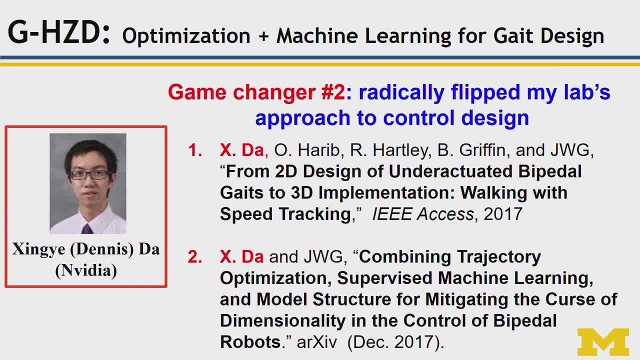 OK, everything we're going to be doing is going to have provable basis, et cetera. Dennis had taken the machine learning classes. I was aware he'd taken the classes. I encouraged him to be up on the technology and stuff. 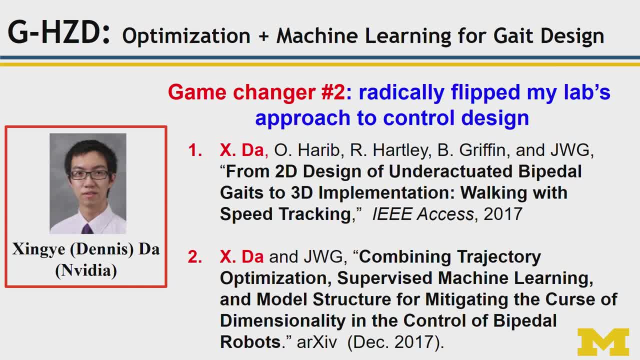 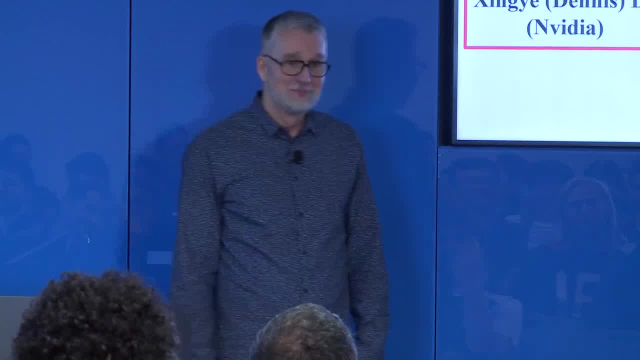 But no, we're not doing that. OK, That's what he did, And he wouldn't tell me he was doing it until he could show me the results. OK, So Dennis is super cool. So let me tell you what he did, though. 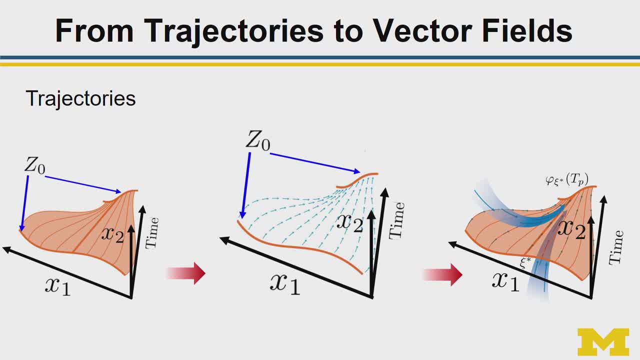 It's awesome. OK, so we don't have silver bullets, but we have something that works really well now in the bipedal community is trajectory optimization, So we can calculate hundreds, if not thousands, of trajectories in a really small amount of time. 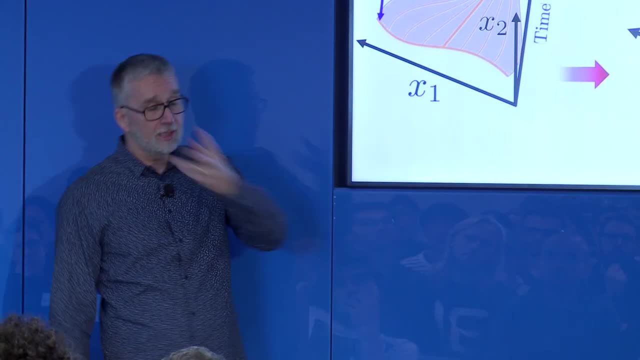 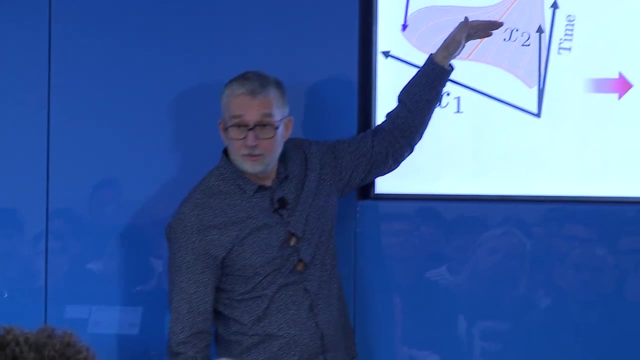 So we can calculate trajectories. Now, trajectories are wonderful until you're pushed off one. Because, then, what do you do? You want to keep following that trajectory and converge back to it. You want to find a different one to follow? What do you want to do? 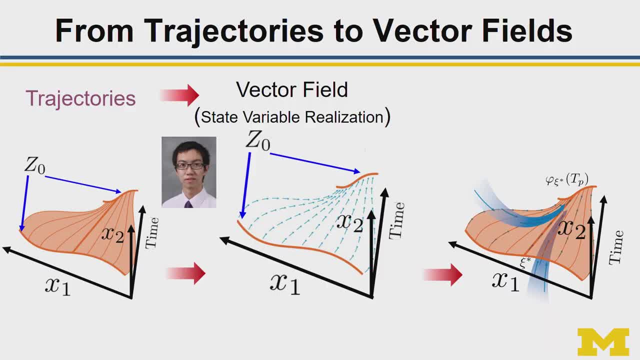 So this is where Dennis' brilliance what he's doing is. he says, OK, I'm going to build a surface And I'm going to find a state, variable realization of it, And I'm going to build a vector field whose solutions are: 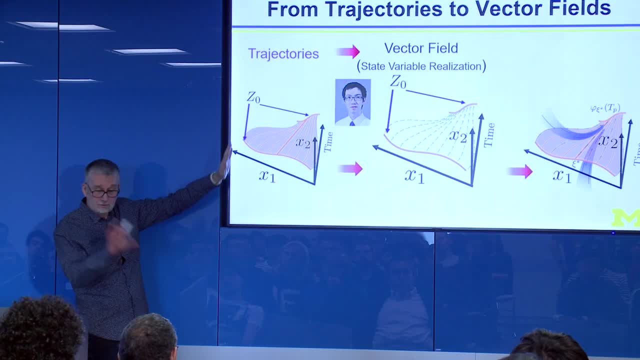 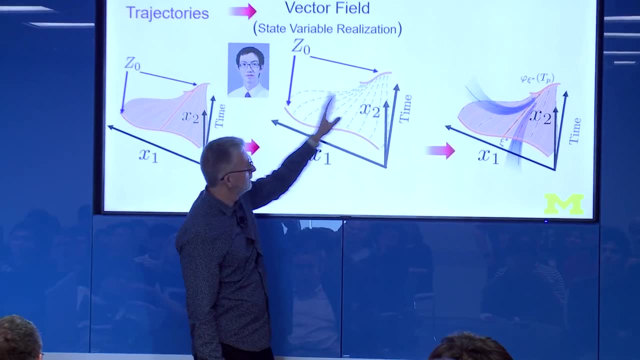 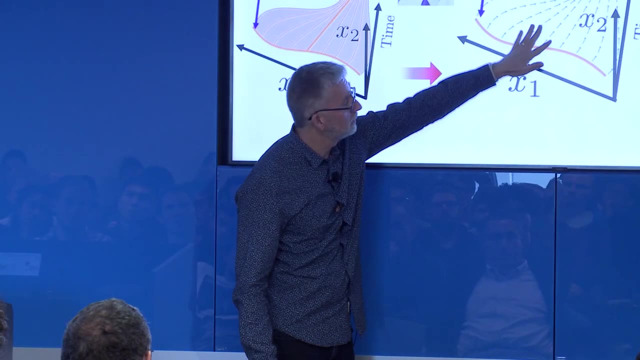 the same as the trajectories. OK, Sounds easy. And then if he has one of these surfaces and it's invariant and the transverse dynamics are nice, we can use our standby trick on the hybrid zero dynamic. So this is the key thing he's doing. 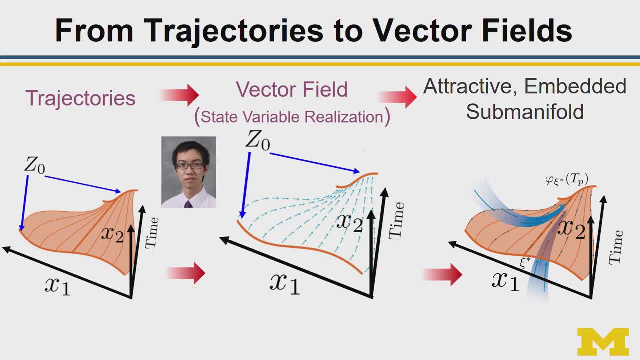 And this is where the machine learning was coming in. So he used machine learning to go from the trajectories to the vector fields, And I'll show you how he's doing that. It's simple, It's supervised machine learning. It's shallow learning. 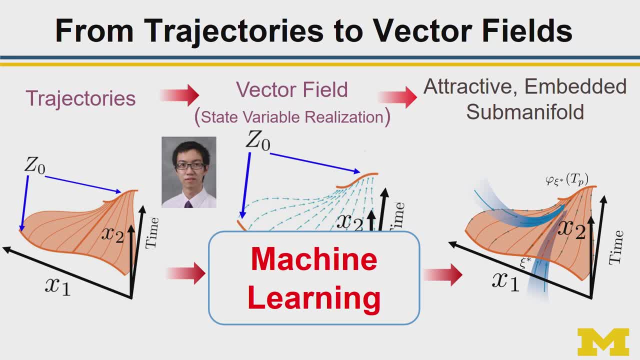 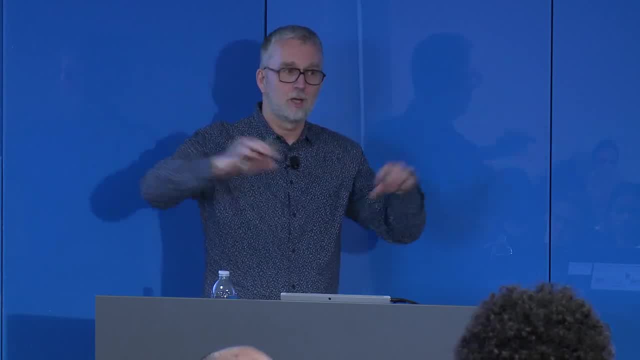 It's not deep, OK, And there's theorems behind the method And the key thing is the machine learning is to build a function that, if it has these properties, there's a theorem that says the closed loop has these properties, So I felt good about it. 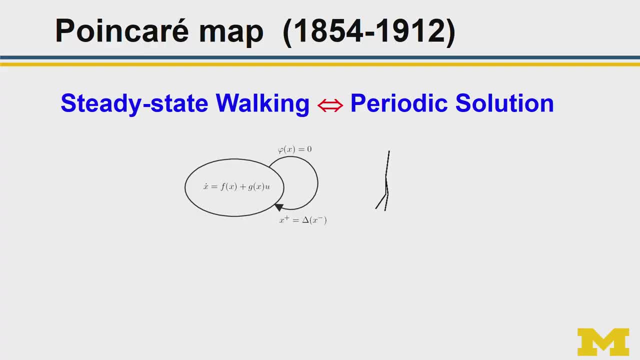 OK, so that's what Dennis did. Yes, Are the trajectories that you could map nice enough so that they can easily sort of form up? Is there a vector field or is there any kind of stochasticity or noise or weirdness in the optimization that? 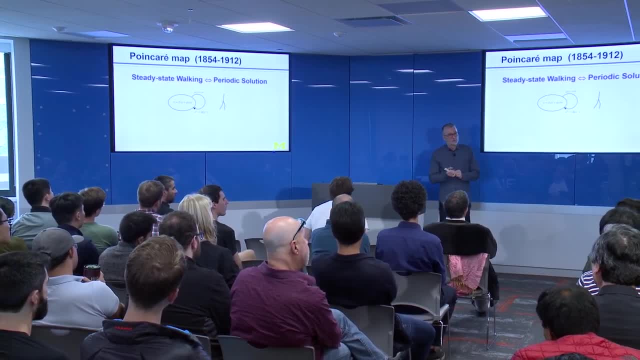 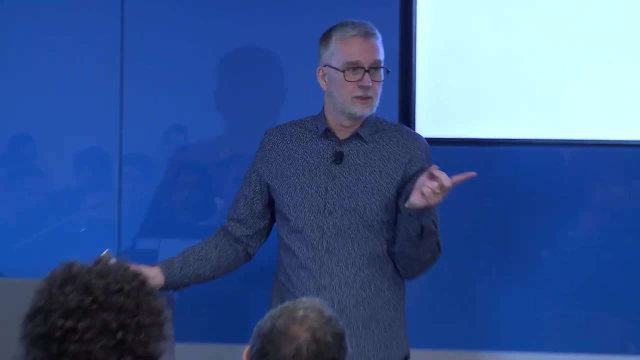 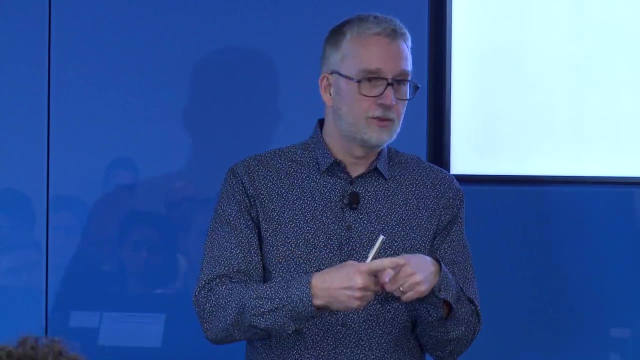 lead to contradictory trajectories. Well, so you're anticipating something that's really important, Because if you have a vector field and it's locally, Lipschitz continuous, you get unique solutions right. So if any of these trajectories cross, that's a topological impediment to this working. 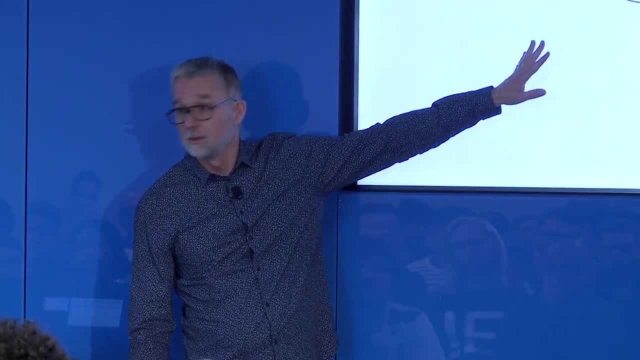 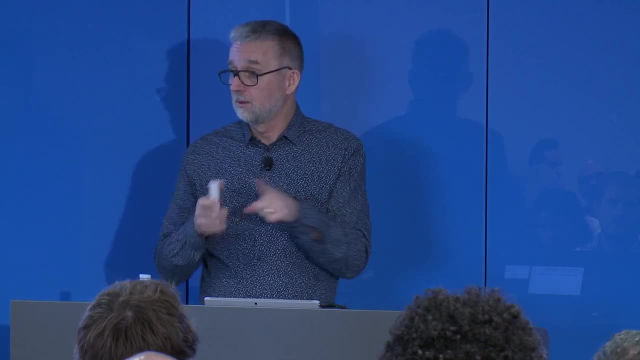 And so that's something that we have, We have to talk about. OK, It's all in a deterministic setting, so there's no stochasticity, But there's nothing in the setting to guarantee this, So let's go back to walking a little bit. 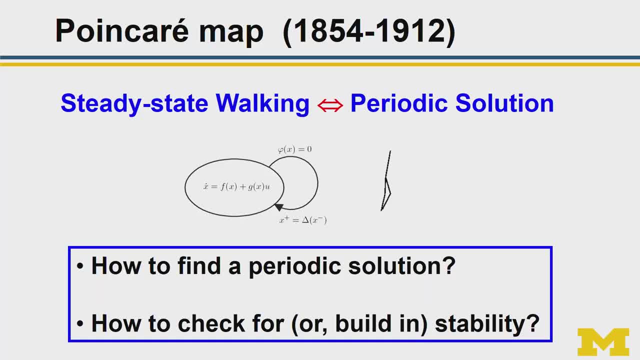 introduce a classical tool. So how do you find a periodic solution in these hybrid models And how do you check if it's stable? We're going to build that into the trajectory design process. So this is work of Poincare, a very, very famous. 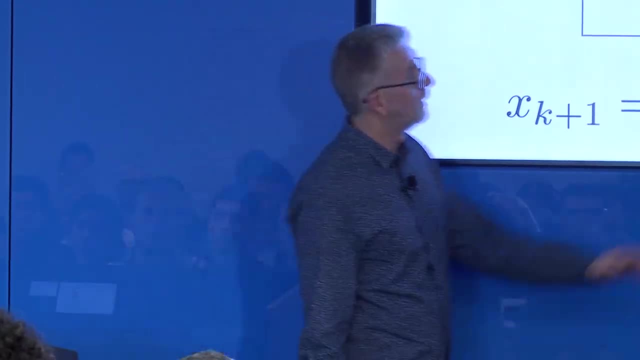 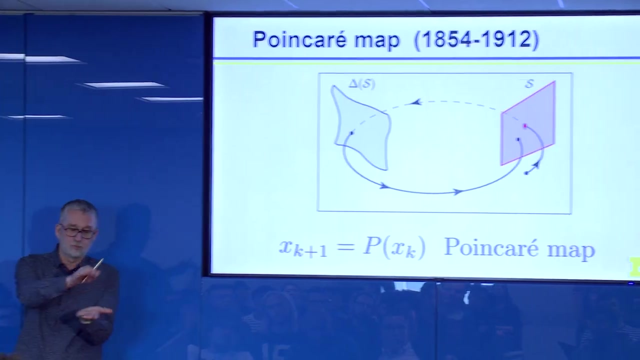 a mathematician just translated into the hybrid domain. So this is a hyper surface, So it's co-dimension one in the state space of the robot, So it's a set of points where the foot is on the ground. So Poincare map is very simple. 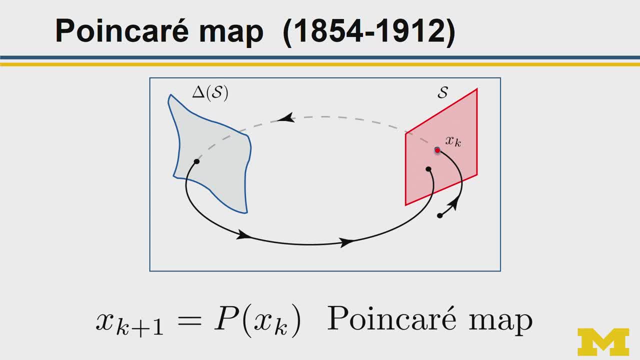 You start out with an initial condition on that surface. You then apply the impact map to it. OK, That gives you the jump and the velocity. Then you follow the closed loop dynamics back around to the surface, And so the Poincare map. 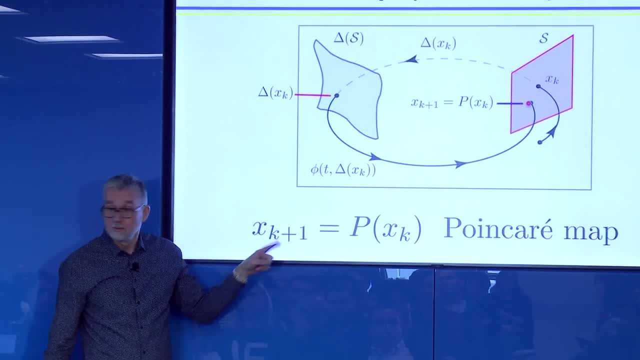 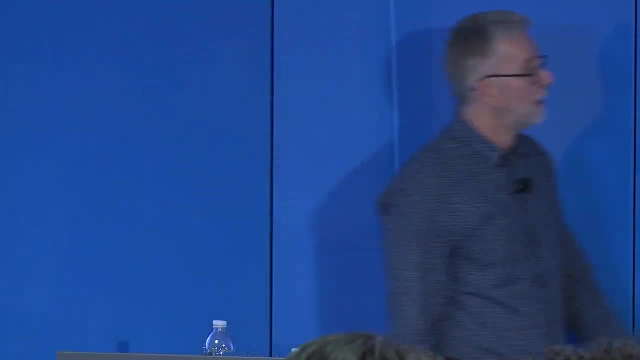 It just takes xk to xk plus 1. So it's hard to calculate analytically, but you can calculate it numerically. So that's the Poincare map, And so to have a periodic orbit, wherever you start should be where you end. 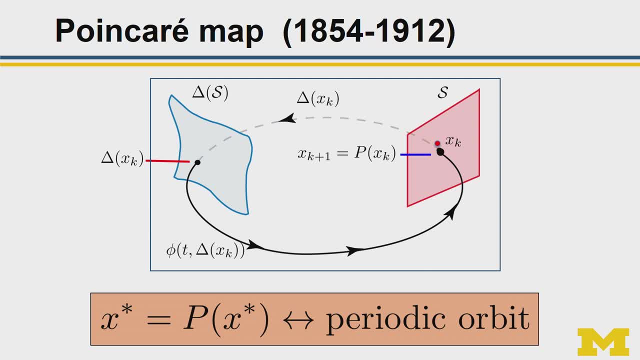 So that's simple. It gives you a condition for checking periodicity And then, if you want stability, you take its Jacobians and you look at the eigenvalues being inside the unit circle. So that's kind of standard dynamical system stuff. 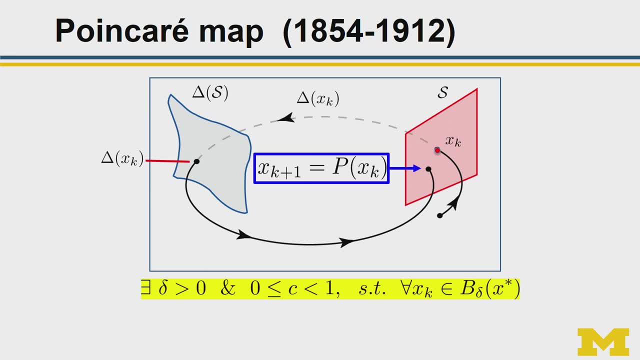 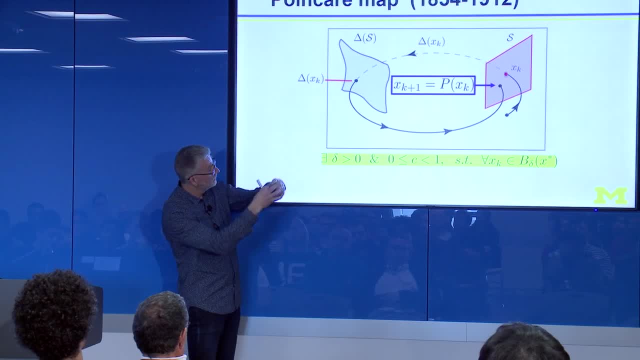 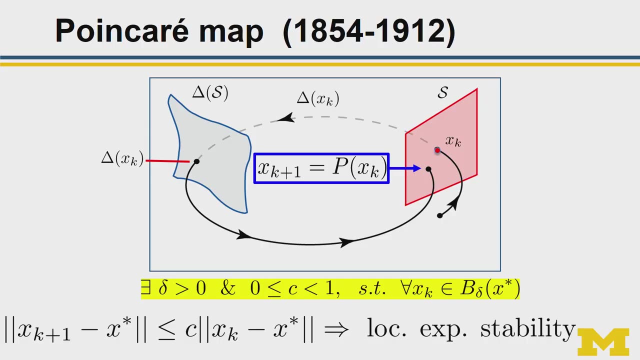 Now there's another way to think about stability, which is more Lyapunov-like, which is: you give me a ball around my point in my Poincare surface and you give me a contraction rate If for every point in the ball, I 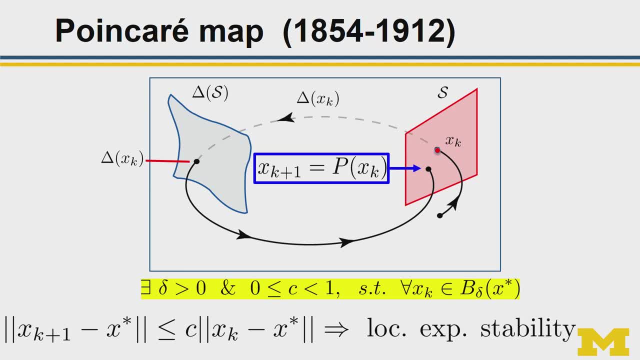 can satisfy that my next point is closer to the equilibrium than my original point by a contraction factor. then I get local expression. That's exponential stability, because this is like the contraction mapping theorem that you'd classically do in class, And so we're going to use this because calculating eigenvalues 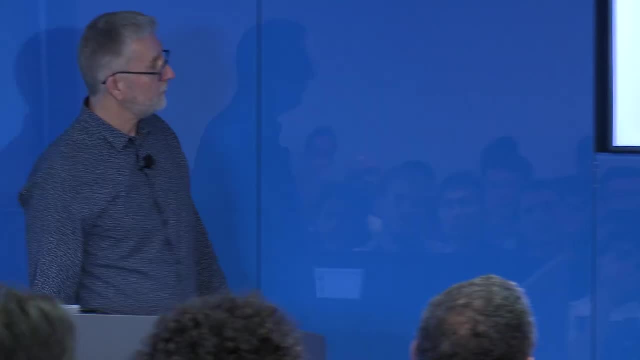 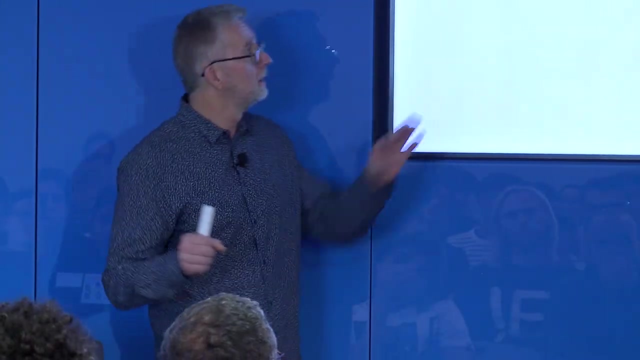 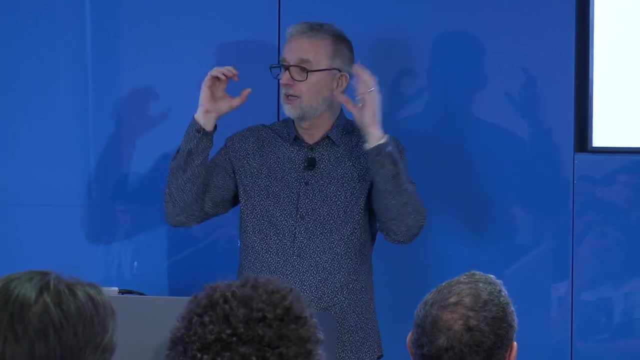 is very expensive. so we're not going to do that. So I want to explain Dennis's setup. I'm going to first explain it. assuming the model is low enough dimensional that we don't have to just build submanifolds, We can fill up the entire space. 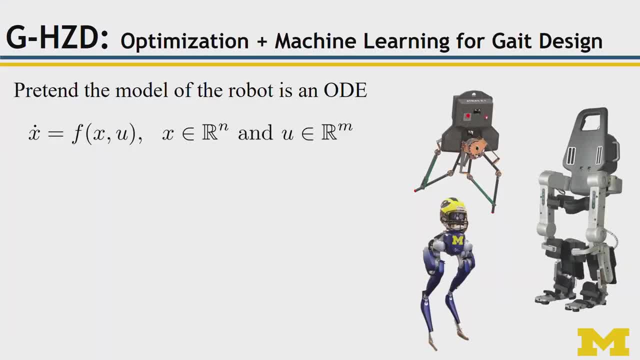 I want you to see the basic idea And we'll actually illustrate it on the most classic example: the inverted pendulum on a cart. Every control person has to solve that problem multiple times in a career to keep their control creed going And to take away another technical thing. 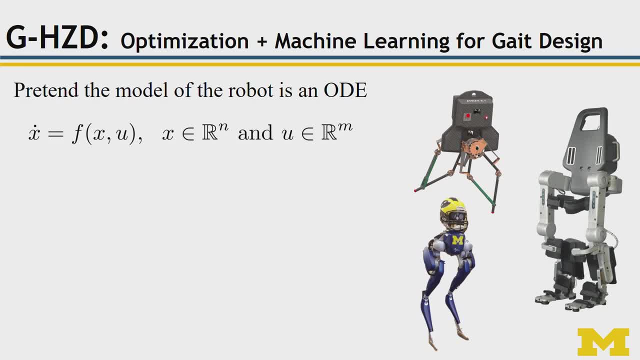 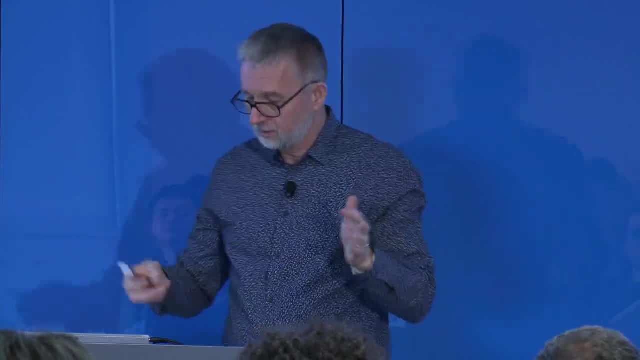 I'm not going to work on a hybrid model, I'm going to work on an ODE. It's just bookkeeping to do the hybrid stuff, as you'll see. But I still need Poincare maps. And you're going like: why would you still need Poincare maps? 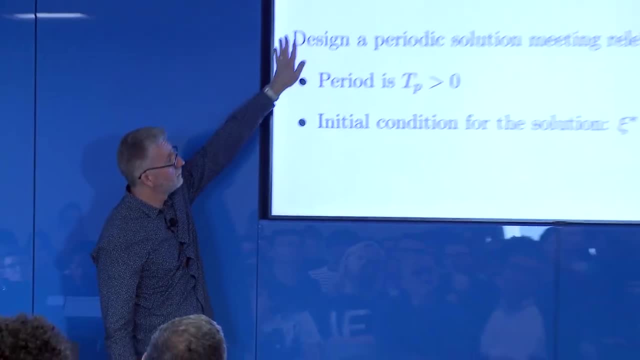 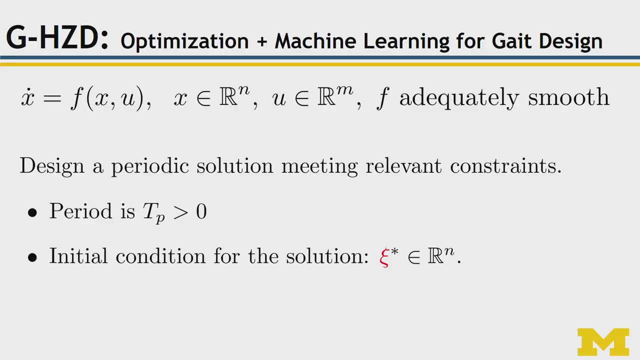 Stay tuned. OK, so we have our model. We find a periodic solution meeting all the relevant constraints that we talked about. It has a period, It has some initial condition. I pick a point in there and just call it an initial condition. 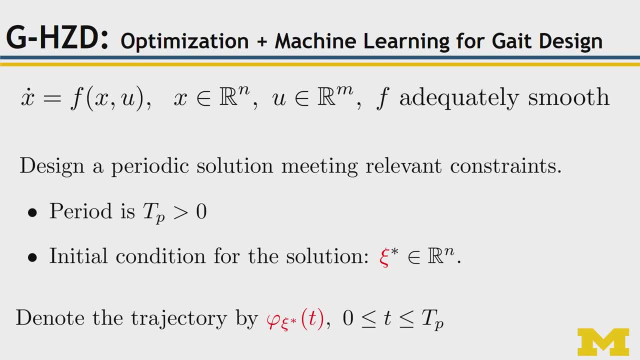 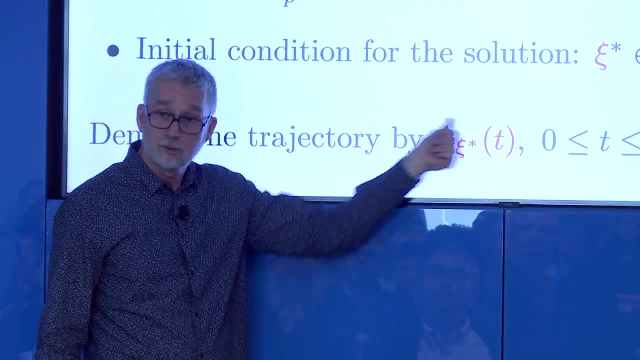 And I'm going to do some bookkeeping here. I'm going to keep track of the solution indexed by the initial condition. So that's what this subscript means on phi, And there'll be a u eventually. I'll have here Which is the corresponding input. 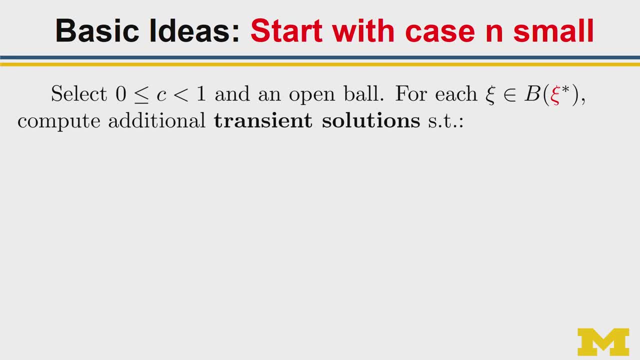 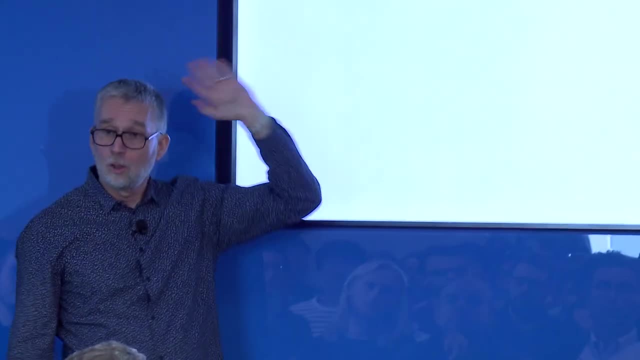 So that's the starting data. I want to select a contraction rate: 0.9.. Just pick a number, an open ball about my initial conditions, And if I can keep meeting them, I'll keep growing the ball. I'm going to compute a whole bunch of other solutions. 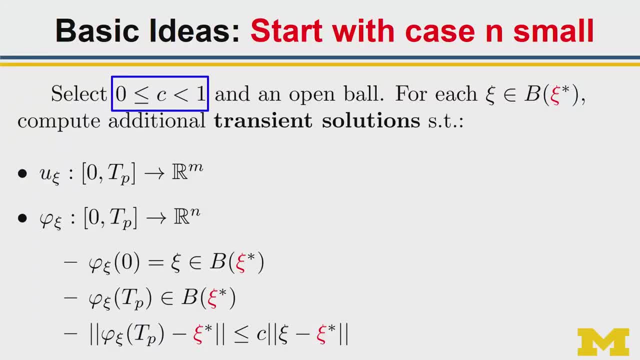 that meet the following conditions. So u indexed by the initial condition, the solution indexed by the initial condition, And for simplicity they're all defined on the same interval. They don't have to be, but just keep the bookkeeping clean. So they start in the ball, they end in the ball. 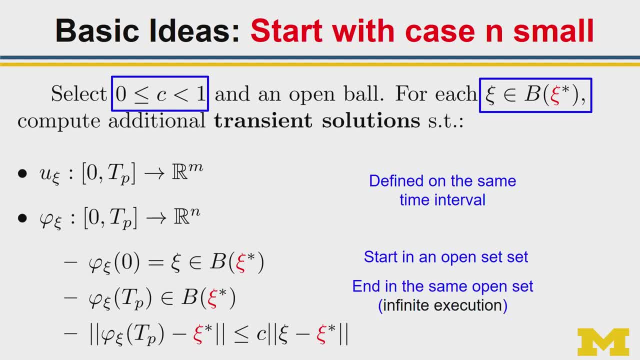 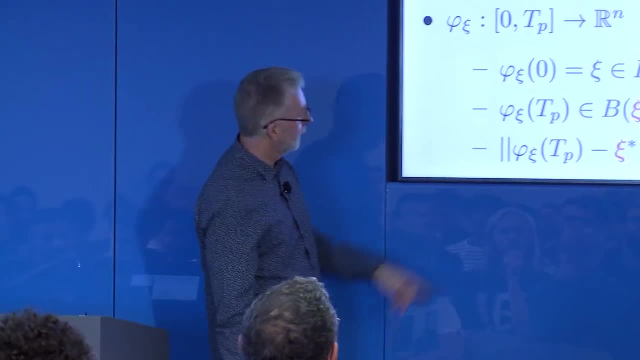 And then the language of computer science. I now have infinite executions. And then my contraction condition is the other thing I impose. Why do I do that? I'm trying to build a statement: stable periodic orbits. I want trajectories that are contracting. 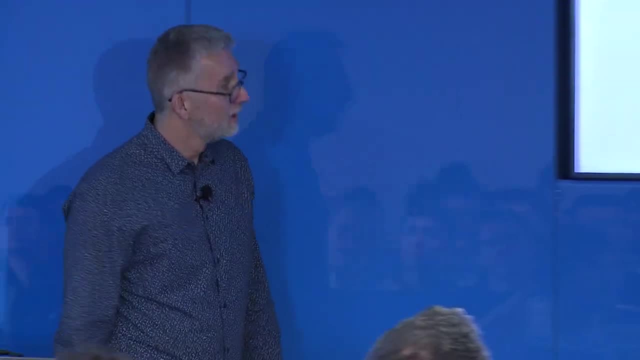 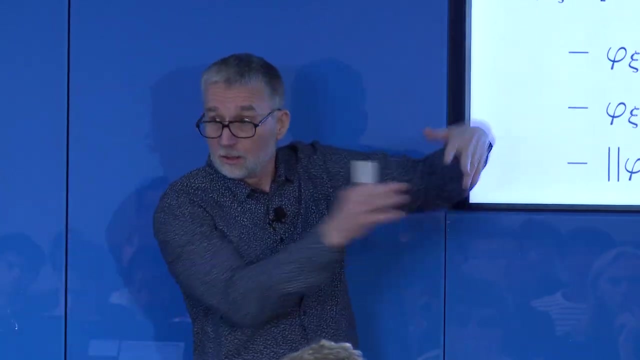 And this is inspired by the Poincare analysis we just did. Now it could be that we can't find any solutions like this, So that's telling me something about the control rate that I have. It could be I can only find them for a small ball. 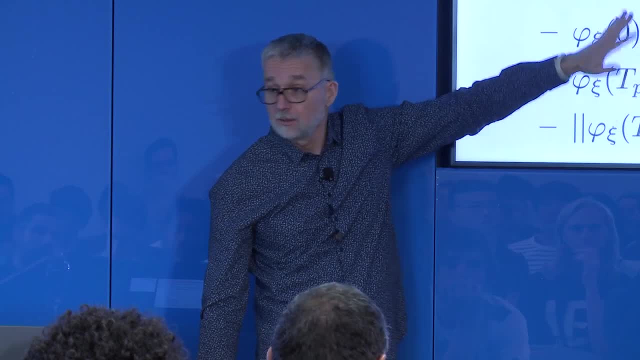 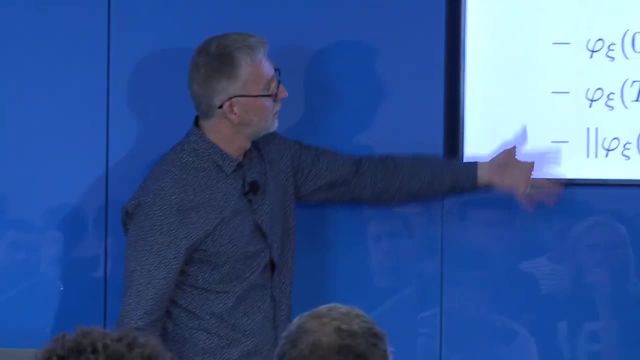 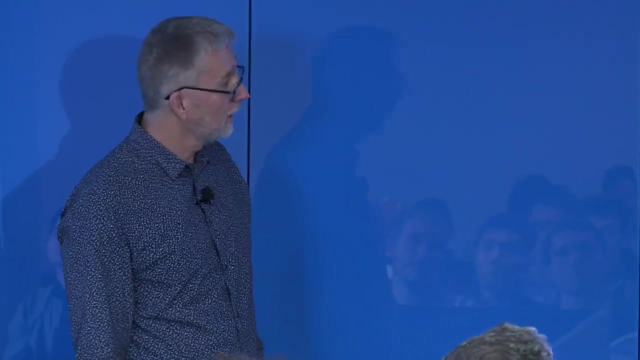 And that's telling me something also about the power of my actuators and things like that. So let's assume that we've settled on a size of a ball and a contraction rate And we can build this family of trajectories. How do I get a control solution out of that? 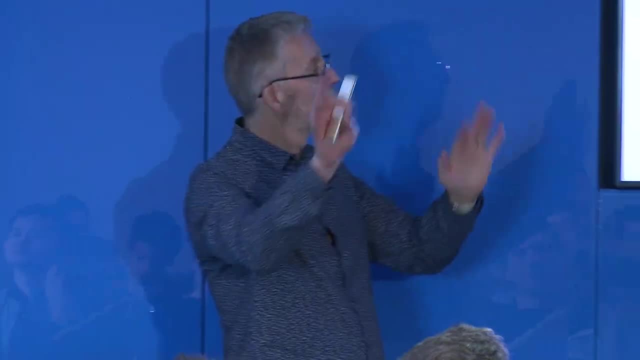 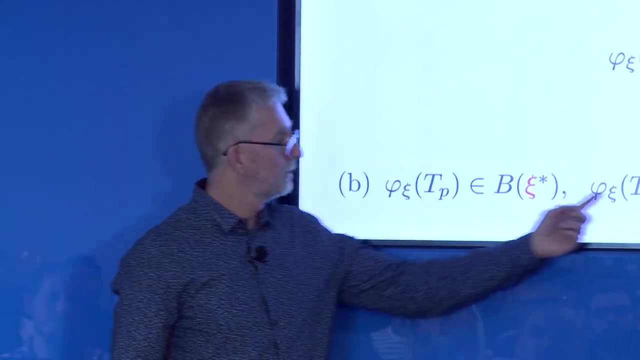 So you can build that trajectories doing many things. Dennis was doing something like MPC, in that he would take his horizon to be three times the period And he'd put a terminal condition that after three steps you were back at your fixed point. So this was the original condition. 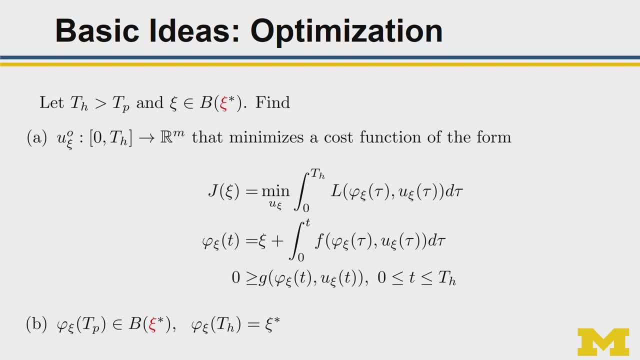 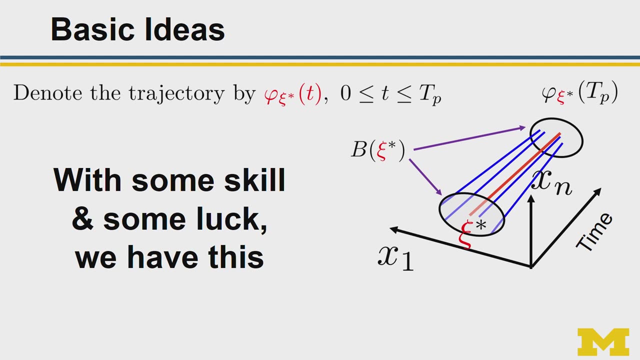 for getting stability in model predictive control. But you don't have to do that. But that's what he was doing: Cost solutions, constraints, invariance, all this stuff. So anyway, that's how you get it. So now everything has gone beautifully well. 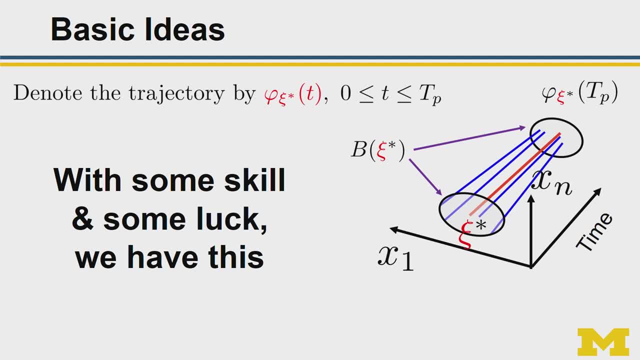 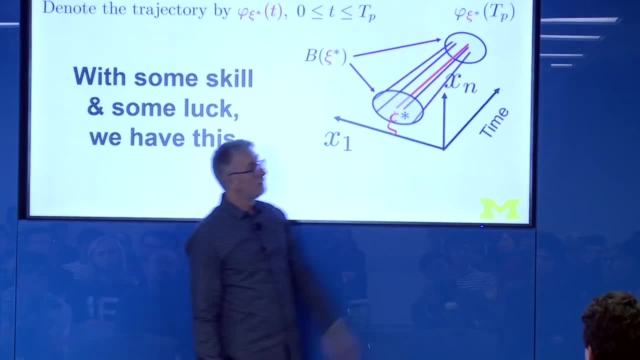 So, a little bit of luck, a little bit of skill. Sometimes it's better to be lucky than highly skilled. But whatever, Here's our initial condition We're flowing through, And then all those trajectories are of length: capital, TP, That's the interval they're defining. 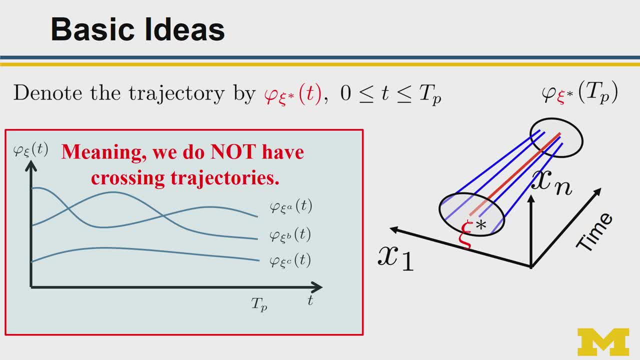 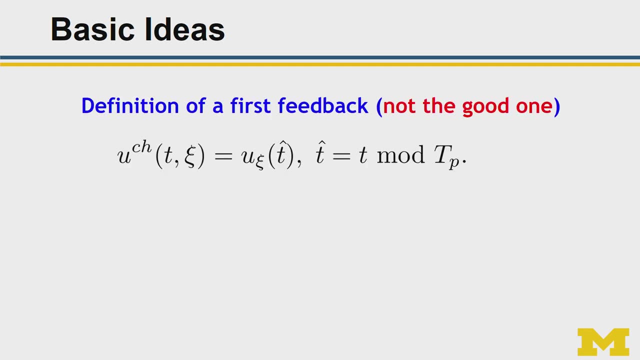 They're defined on And the luck. I mean we don't have this, Because I want a vector field And this means I don't have unique solutions. Now I want to build feedbacks And if I put them to my system now, I'm 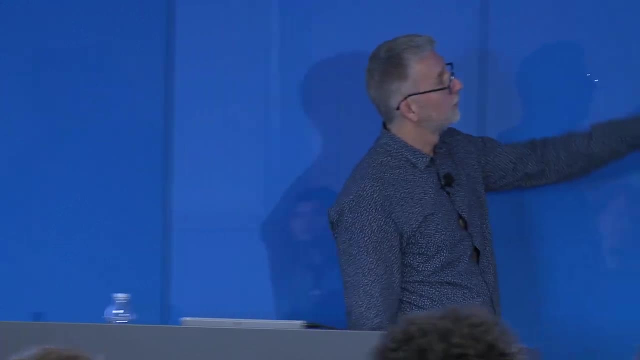 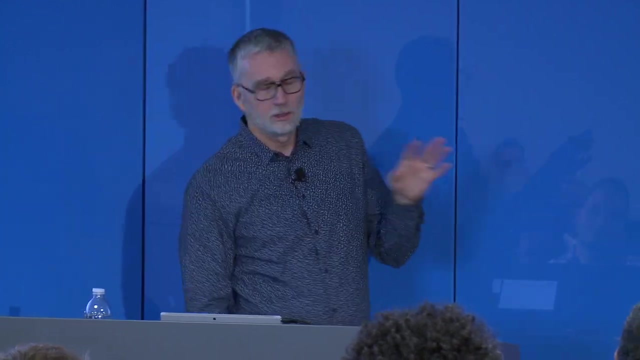 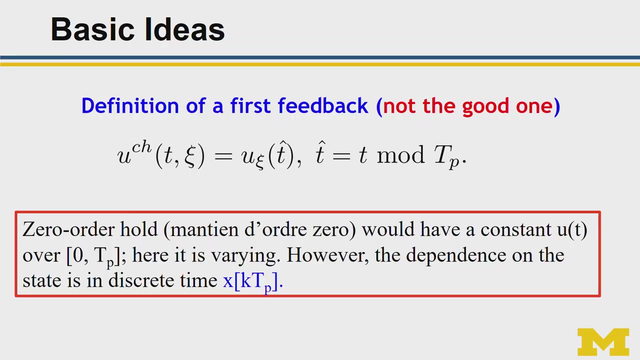 really building the closed loop vector field, And so that's what you see in the case of working with the complete model. So I'm going to give you a first feedback that looks like sample data control, So my feedback is for a given state at time 0,. 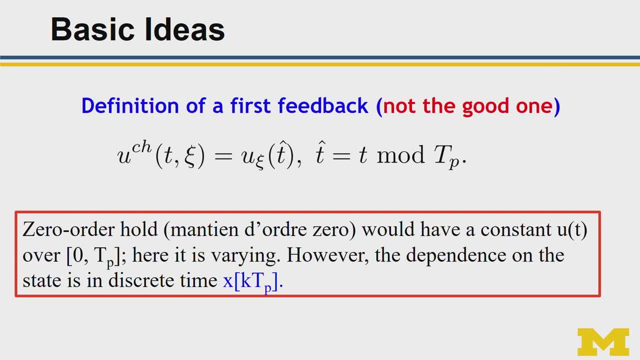 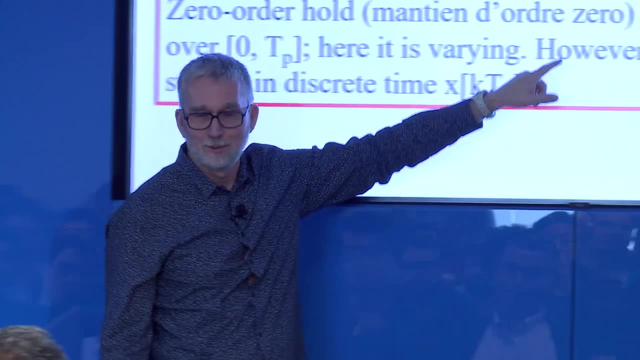 I follow the control associated with that And then, after TP seconds, I update. So this is like digital control: Every TP time step I just update. What's different than what What Jean-Jacques would like to call a, is that we're allowing the control to change. 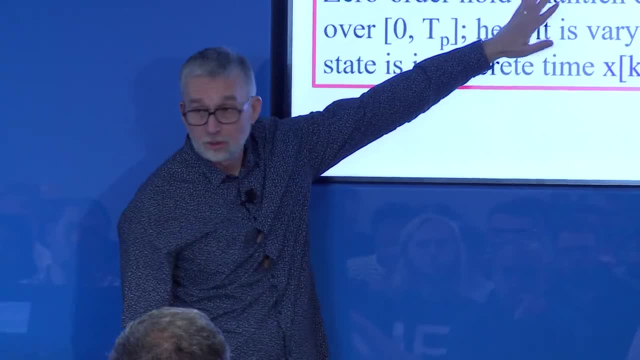 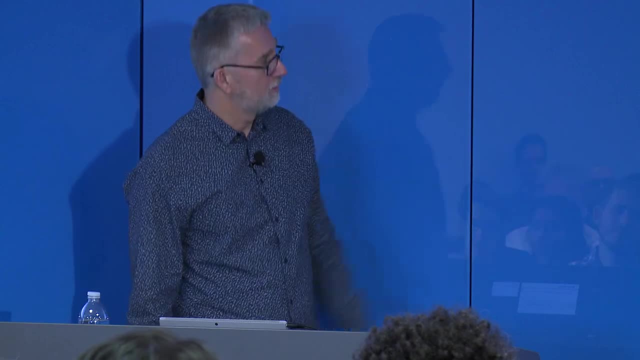 during that period. It's not constant, But it's still just digital control here. It's being updated at the period And warning: it's not a good feedback controller. So it's really a discrete time feedback controller. So how is it working? 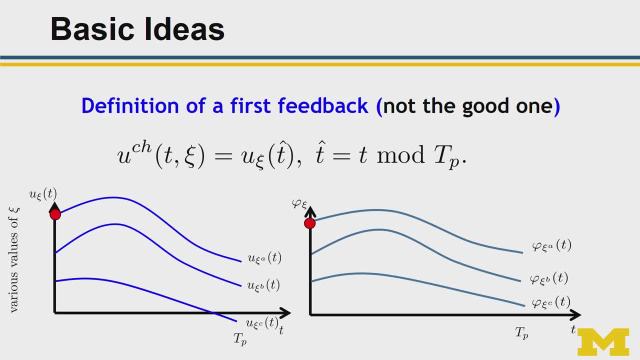 Just to be clear: Time 0, I have an initial condition And then I'm going to update. I apply this control And I've already computed the trajectory so I know where it goes right. So then I follow it back. 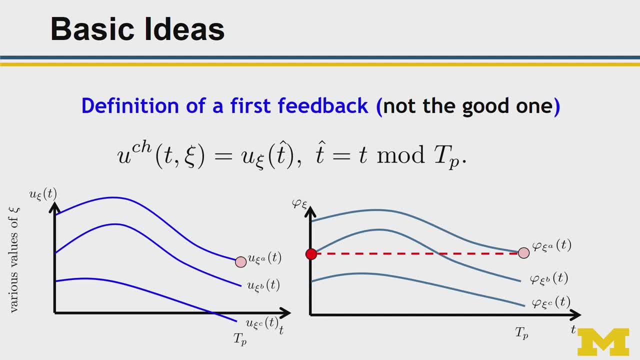 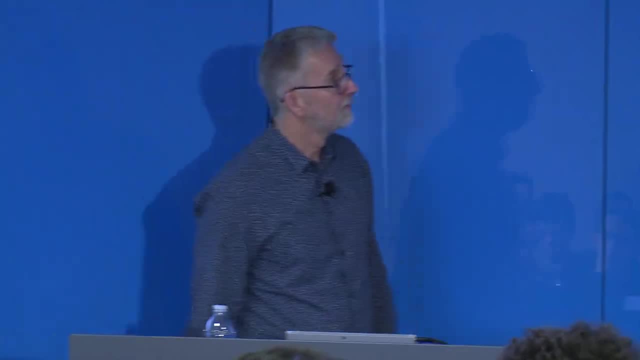 I've got a new initial condition Now. I've got a new control signal that I apply, And then you keep doing this. So it's sample data control. Is the system stable? Well, No, No, No, No, No. 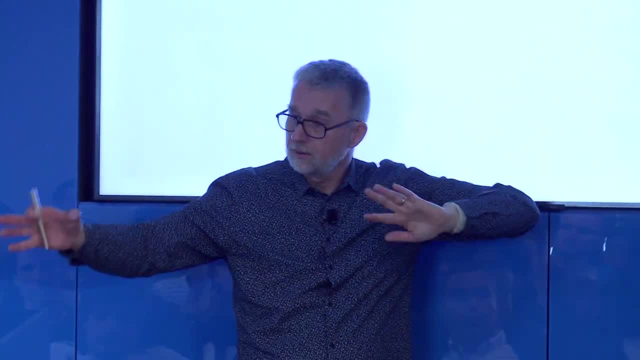 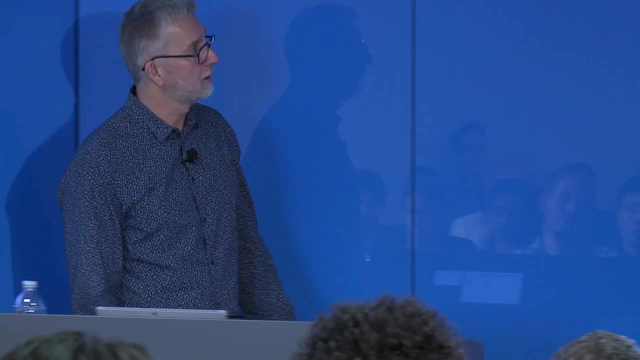 Digital control is a hybrid system, A continuous dynamics of a discrete time controller. My switching surface is t, equals the period, And so I'm appending time to the dynamics. It's evolving as t dot equals 1.. And then, when I reach TP, I reset time to 0. 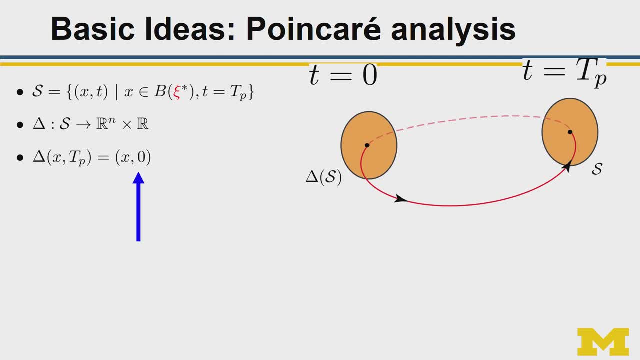 So I'm going to apply my Poincare analysis to it. So I take a point, I apply my impact to it. It just resets the time, doesn't change x. Then I apply my feedback control, I get a new xk plus 1, okay, And they all satisfy this. So by 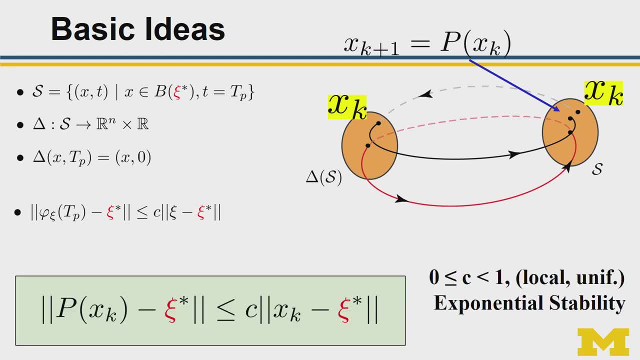 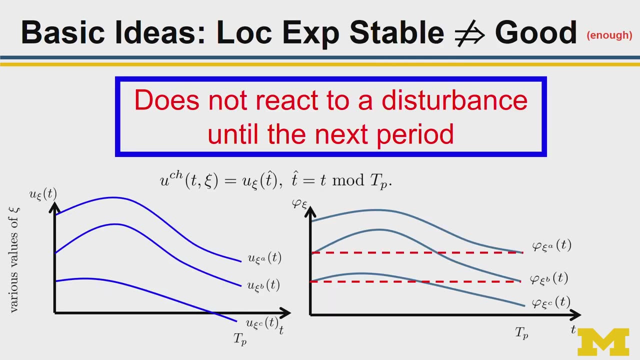 my Poincare analysis, this system is actually uniformly exponentially stable. What's wrong with uniform exponential stability? We work really hard to get it okay. Nothing's wrong with it, right, Okay? the problem is, this thing does not respond well to a disturbance because you're following the trajectory you get. 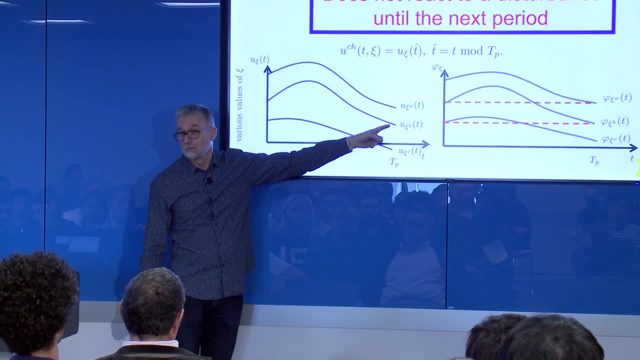 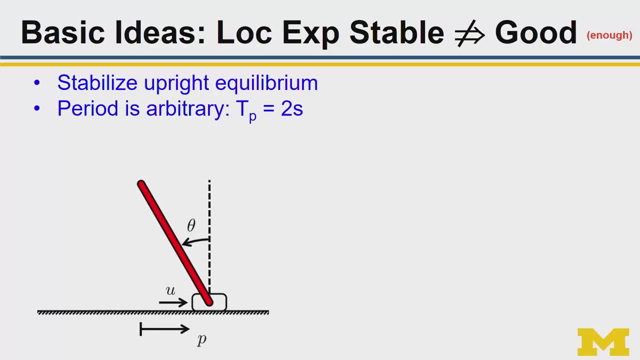 kicked off. you keep following this control. It's digital In between the samples you don't update, So that's why it's bad. So here's the inverted pendulum on a cart. We choose an arbitrary period because it's time. 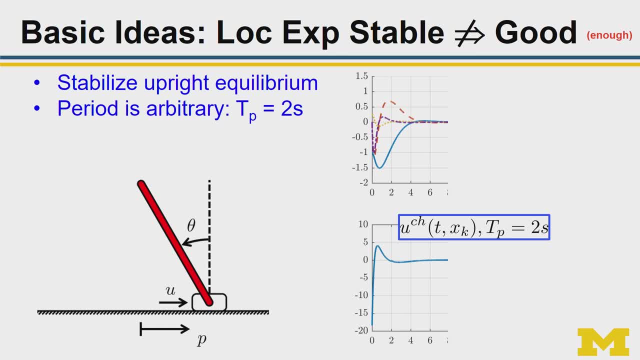 invariant. It does super well. This is what any MPC controller would give. And the problem is you do a disturbance that's half a second before the next update, and then you have a disturbance that's half a second before the next update, and then you have a disturbance that's half a second before the next. 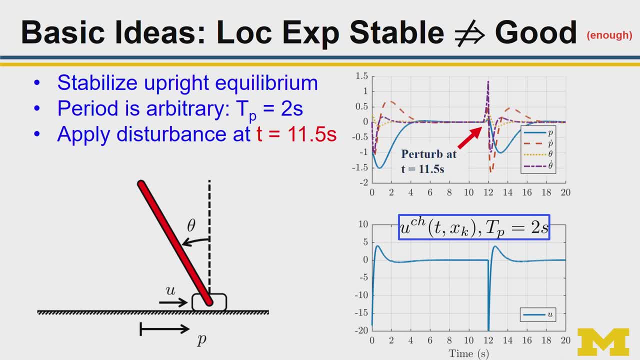 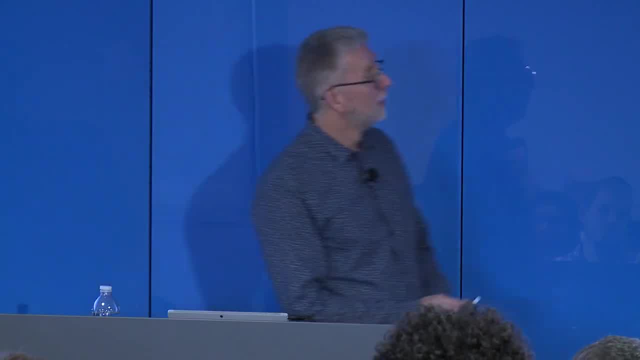 update and then you have a disturbance that's half a second before the next update and you get these awful oscillations. And if that's a robot, it's on the ground. okay, It's a pile of junk. So it's a terrible controller, Okay so. 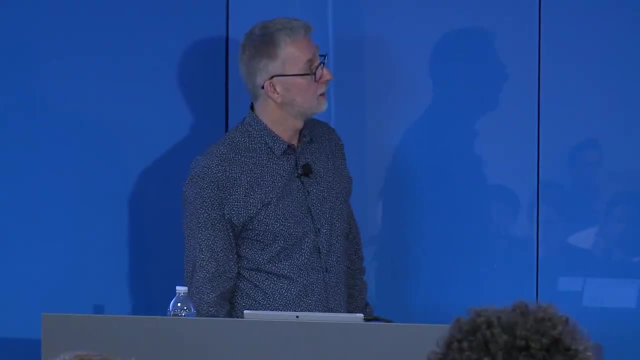 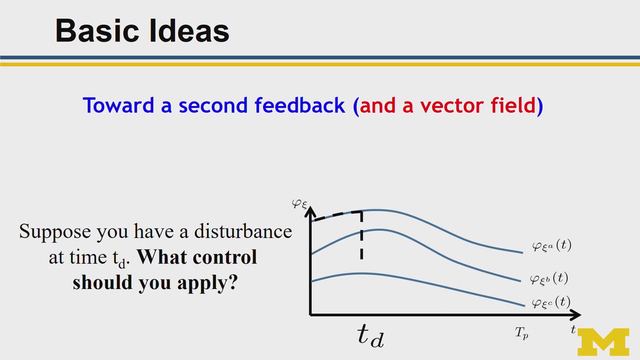 let's now see if we can build a different feedback, the one Dennis really built. So you're following the trajectory At time t disturbance, you get pushed off the trajectory. What control should you apply? The one that tries to drive you back here? Remember, before we just kept applying this. 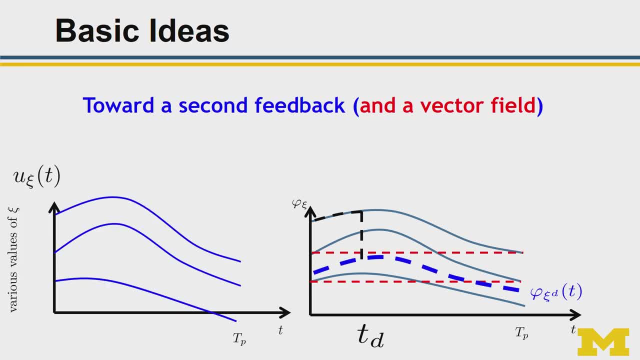 control. Wow, If you can find the trajectory that's passing through here and then index into the control that corresponding to that, that's really what you want to do. okay, It's obvious as soon as you see it. okay, So that's the. 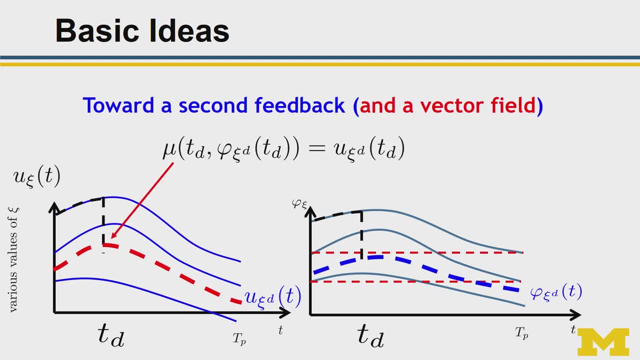 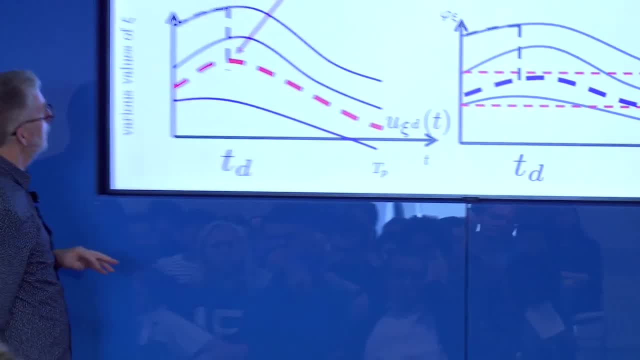 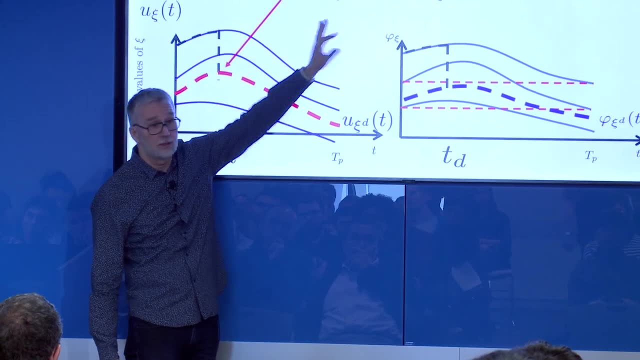 control you would like to be applying, and there's the interpolation condition you want to meet. okay, So you have a bunch of data, You've computed all these trajectories and if from those trajectories you can build the feedback that satisfies this implicit condition, then you're going to 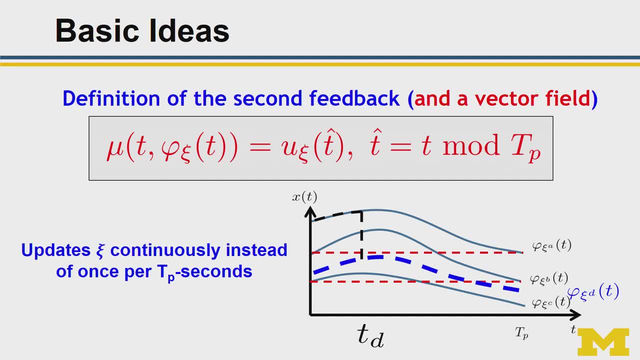 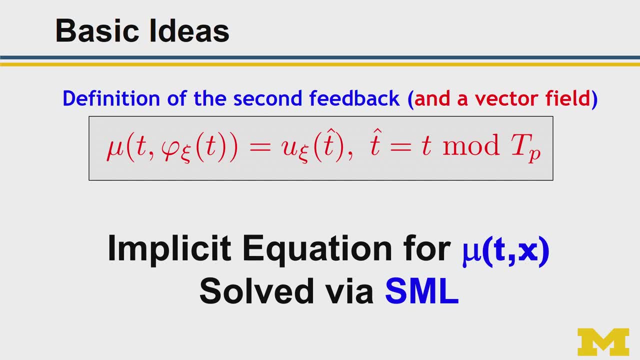 respond immediately to the disturbances. okay, And so that's what Dennis does. It's an implicit equation, and this is where he uses supervised machine learning to pull this function out of the data. So how do you do that? Well, you take an. 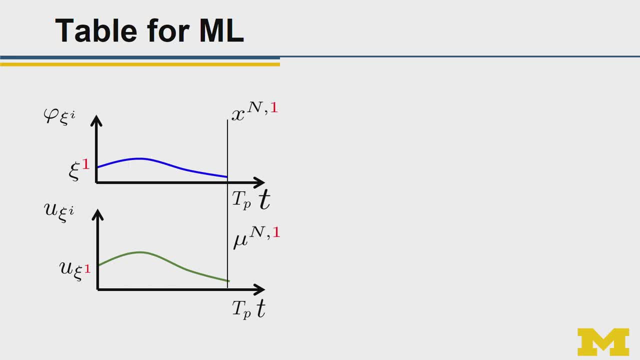 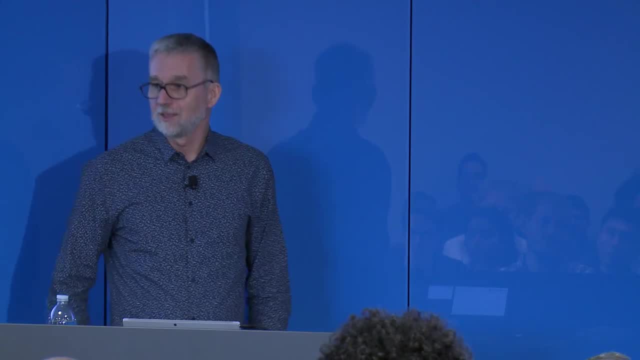 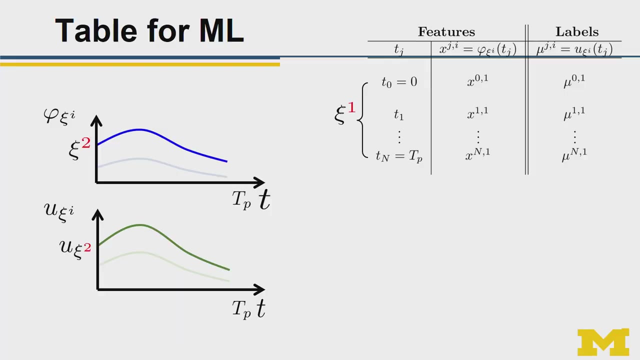 initial condition. you sample it at a whole bunch of times and you put that in your table, and then you use the words, features and labels so that you look like an intelligent human being. okay, What are you laughing about? It's true. okay, You take another initial condition, you sample the time and you 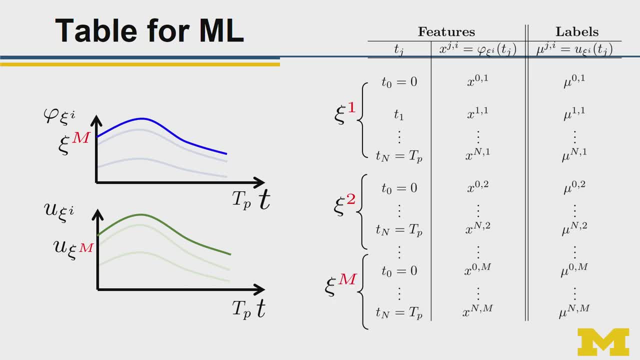 put that data in your table and you take another one and you fill it up, okay, And then you run your supervised machine learning algorithm. We just use the stuff in MATLAB. You try to learn the policy and then you look at the quality of fit on. 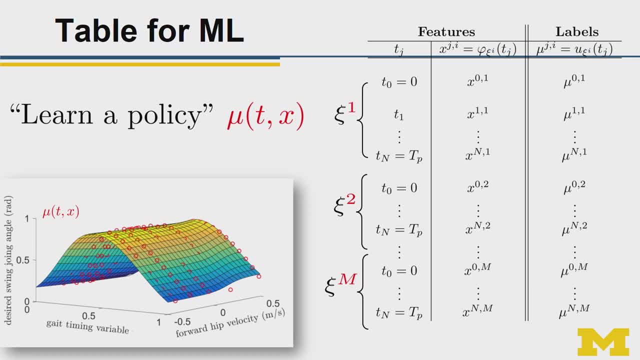 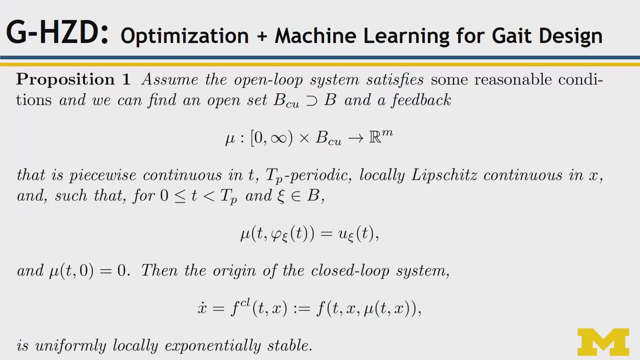 training data versus validation data, etc. And if you get something like this, then you've built the function okay. And the theorem says: if you take the open loop system and you build that bundle of trajectories and you can find a feedback control that satisfies this interpolation condition that we just 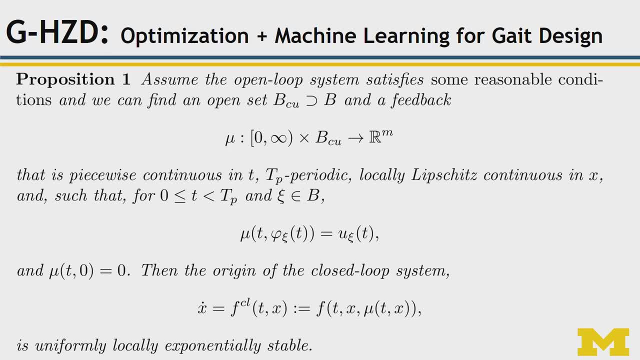 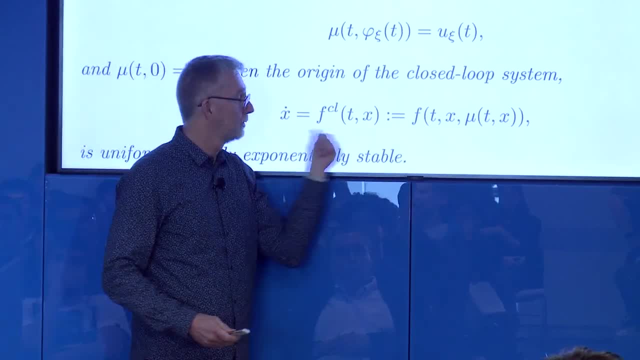 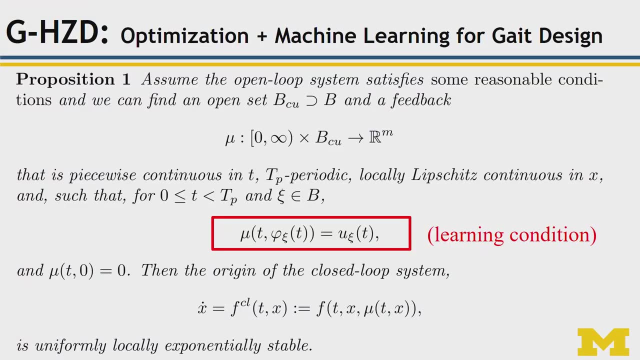 talked about on the data. if you can find that function, then the closed loop system will have the origin or, equivalently, your periodic trajectory as an exponentially stable fixed point. Okay, And it's the same argument from Poincare to prove that this works. okay, That's the learning condition, and then this is the closed-loop. 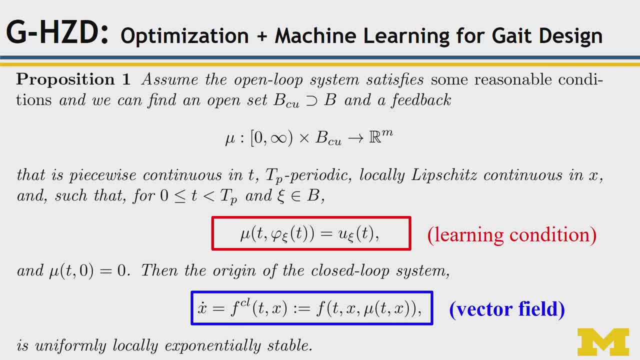 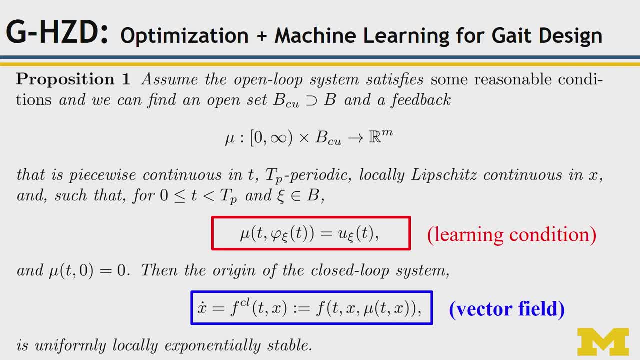 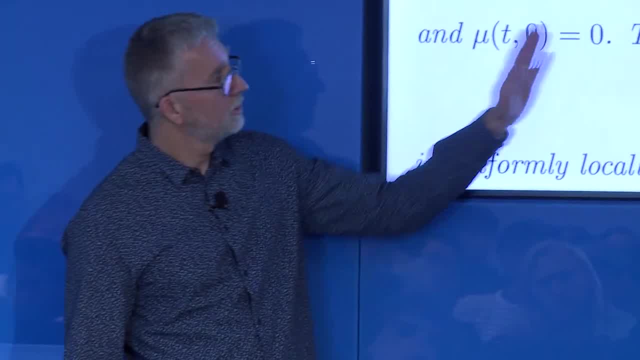 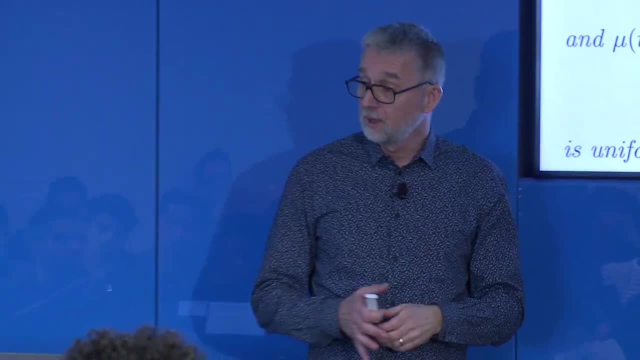 But the switching is state-dependent. but is it really so easy to do? It is, And because the way we do it is, we move the switching point to the middle of the step and then we switch on time once again instead of space. 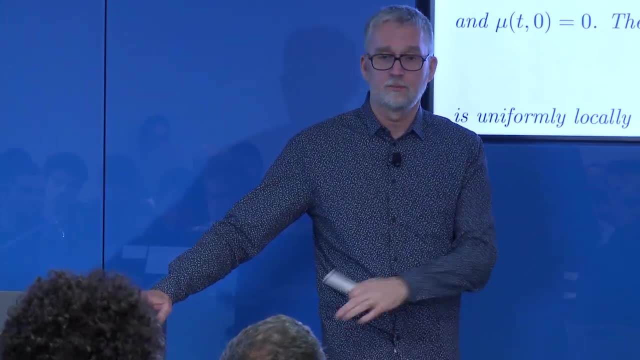 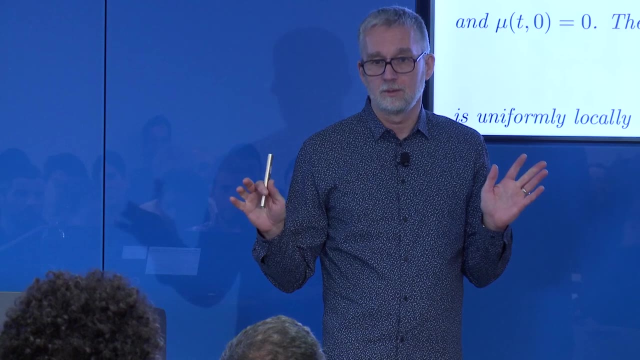 And the reason to do the switching here is because the swing leg is as far as possible from the ground. If there's a small jump or discontinuity in the controller, it doesn't cause problems. So that's how we turn it into a bookkeeping problem. 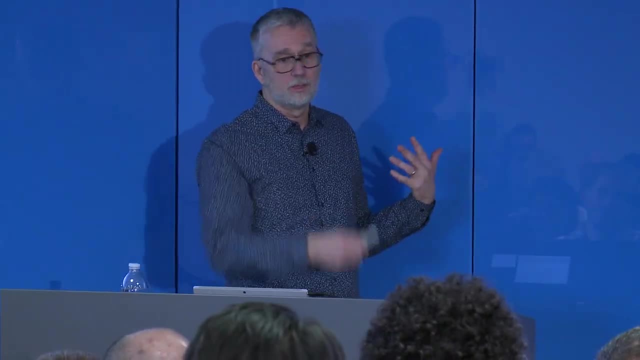 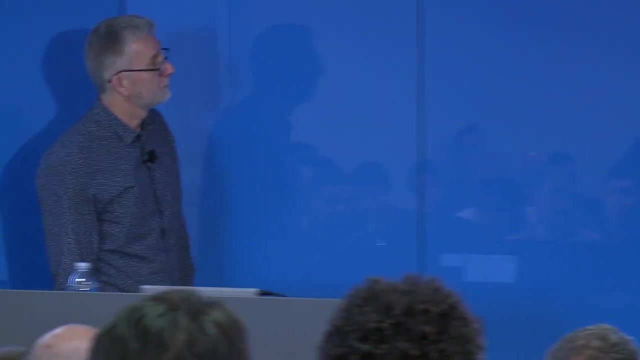 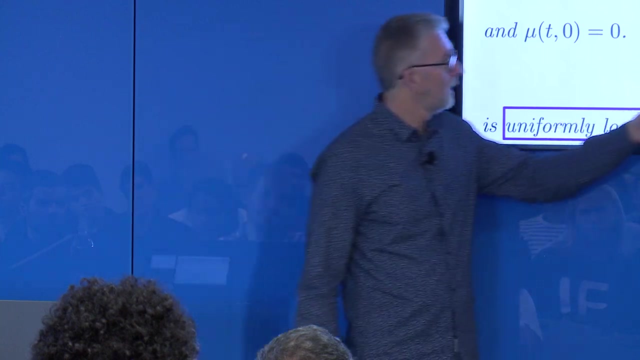 You have essentially two sets of ODEs and some switching conditions, but the switching conditions are just part of an entire surface. Okay, So you get uniform local exponential stability. Now here's the fun thing: The Poincare map for this closed-loop system is the same. 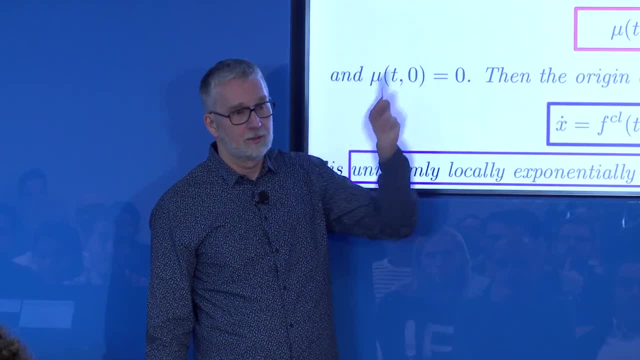 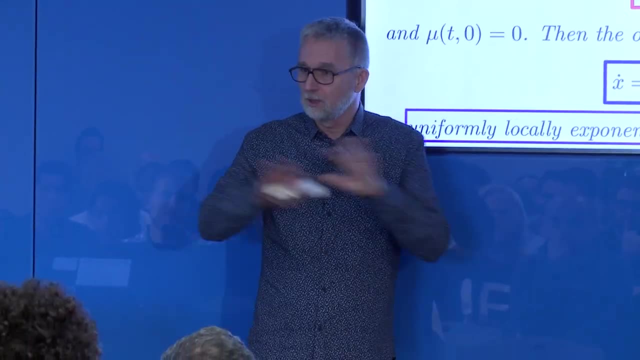 as for the bad one, Okay, I don't prove it here, but think about that. What does that tell you? Exponential stability on a Poincare map means almost nothing. It's not robust, Okay, It is totally not a robust idea. 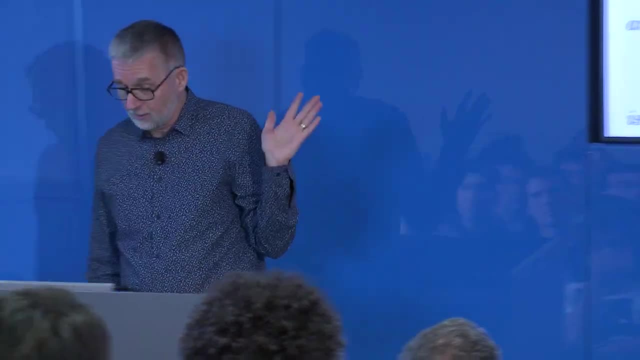 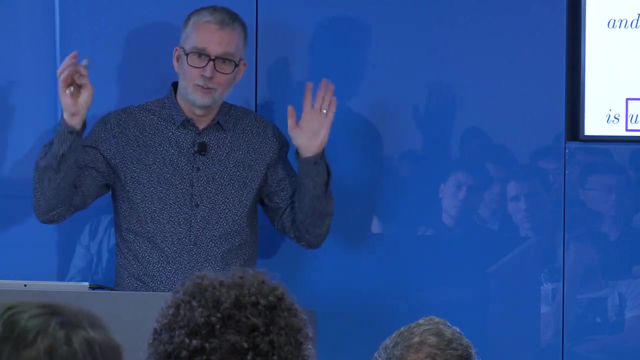 Okay, This is much. okay, they have the same Poincare map. What they don't have is the same disturbance to state stability properties. Okay, You need to think robustness. It's really hard, Okay, When you put this on the inverted pendulum on a cart. 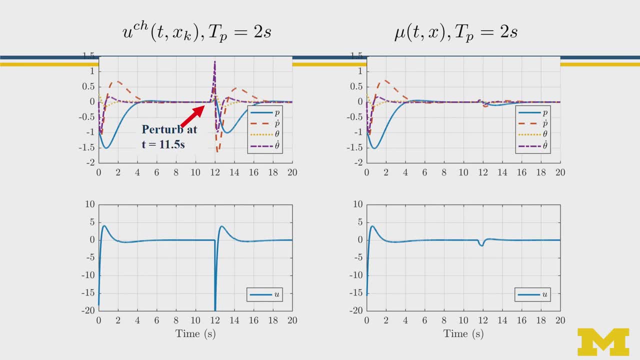 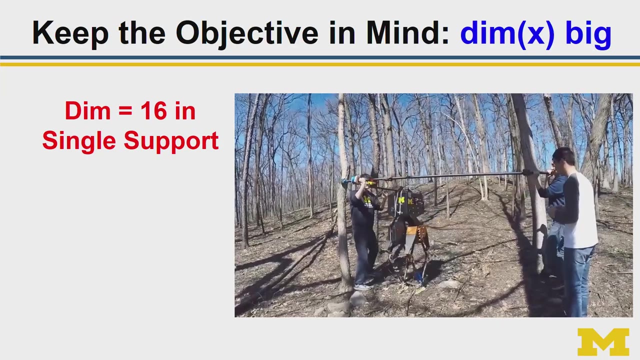 it's, it rocks, Okay, And of course, I'm going to show it to you on a robot, Okay, Because nobody believes simulations, because they always work, but that's so much better, Okay, Okay. so remember, I told you you want to put this. 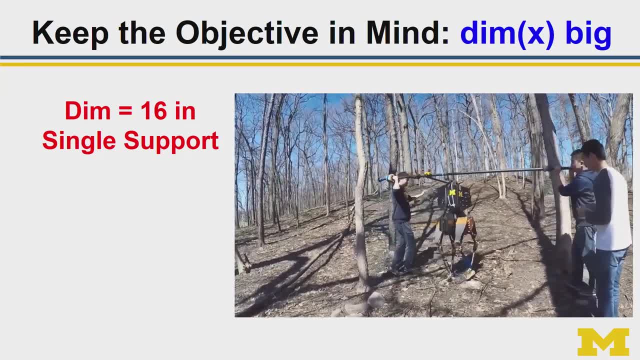 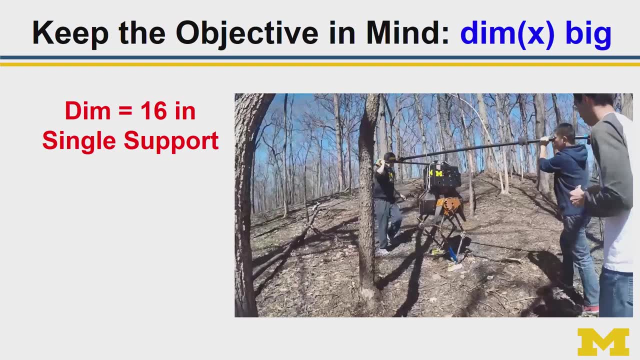 on a robot. they're high-dimensional and I showed you the basic method. It's really exploiting what you can do well: trajectory optimization and then organizing your plan of attack to build vector fields. Okay, Now we want to get this working on Marlowe. 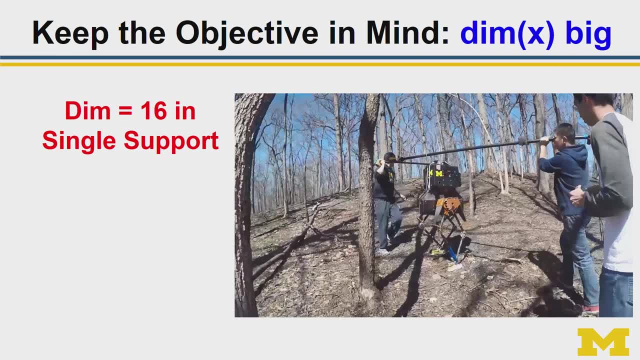 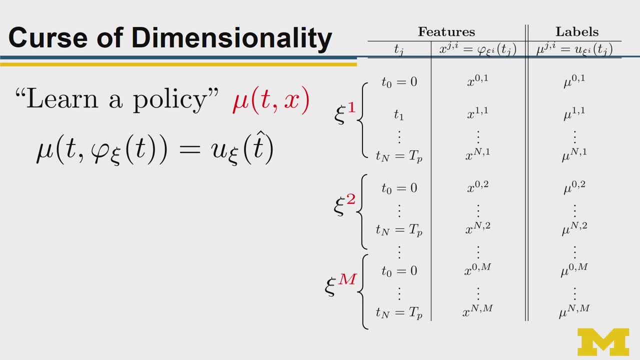 the Atreus robot and it has dimension 16 in single support. Okay, So we need to talk about curse of dimensionality. What's going on here? So, if I just do five samples in each state, space dimension, the origin, two on this side and two on that side- 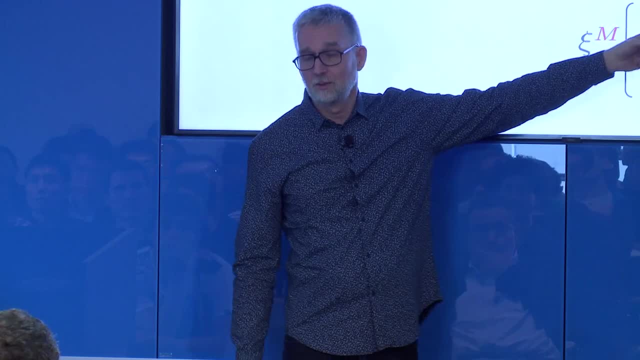 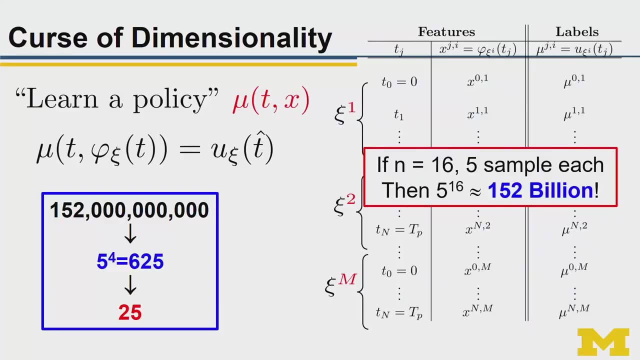 and I have 16 dimensions, that's 150.. So that's 152 billion optimizations. Okay, I don't care how fast you're doing them, you probably can't store them even on your computer. Okay, So I'm going to convince you. 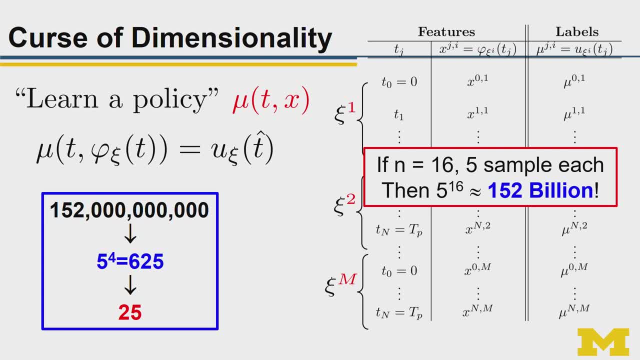 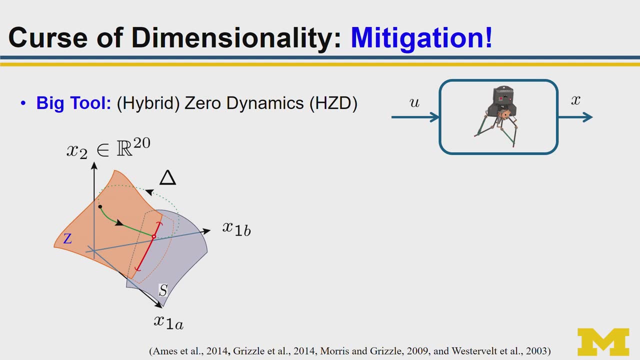 that 625 is easily enough. Dennis does it with 25 trajectories. Okay, Is that a gain that's worth going after? So that's what he did. The big tool, once again, is going to be invariant. Okay, So that's what he did. 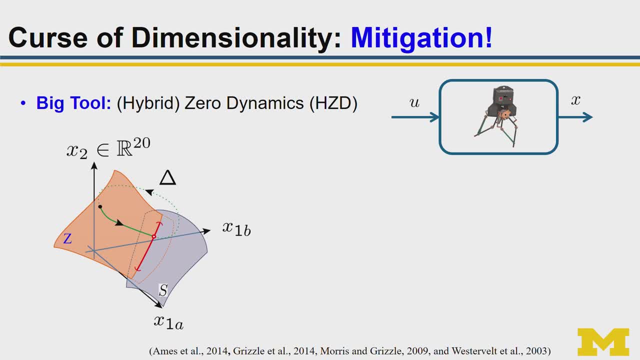 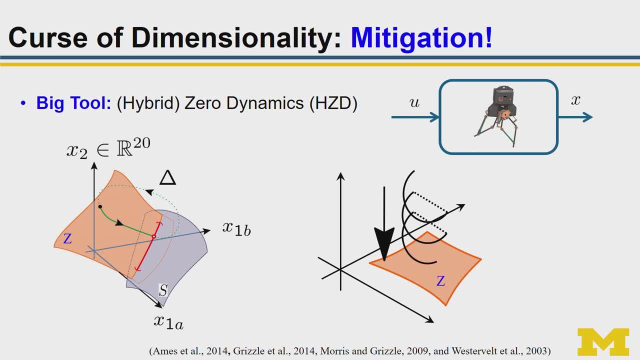 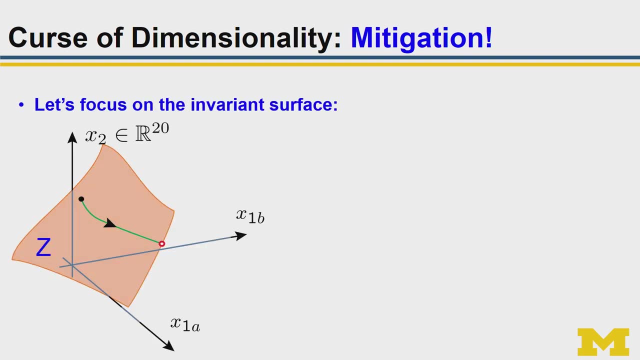 that's different than what we were doing before, But the big tool will be creating a hybrid invariant manifold having nice transverse dynamics. but he is going to build a much more beautiful manifold than I knew how to build ever, So okay. 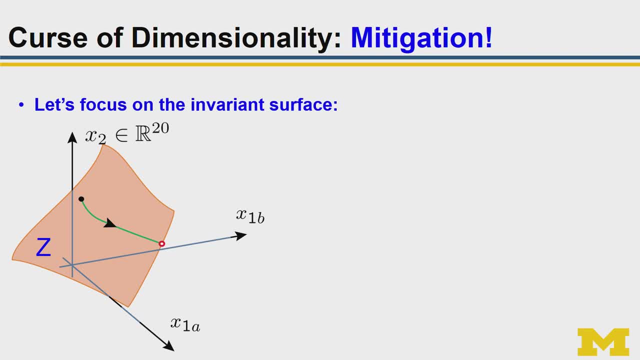 So let's focus on the invariant surface. So this is what we always did before. Remember, I emphasized for a single periodic orbit. then we built this entire controller. It's kind of crazy, wasn't it? But I showed you it working on three different robots. 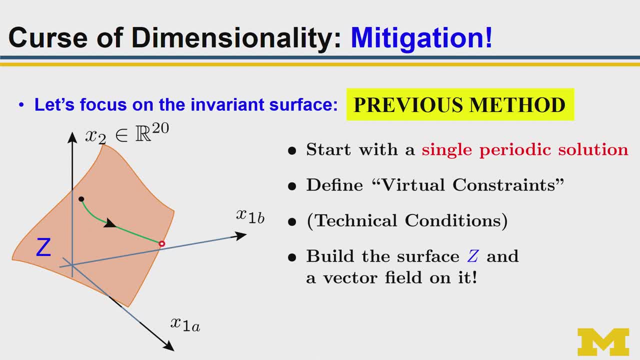 But what did it do? So here's the orbit. These virtual constraints define an immersion of that path, its position and velocity into the full state space. Okay, That's what taken, this trajectory, which is a path, and its velocity into the full state space. 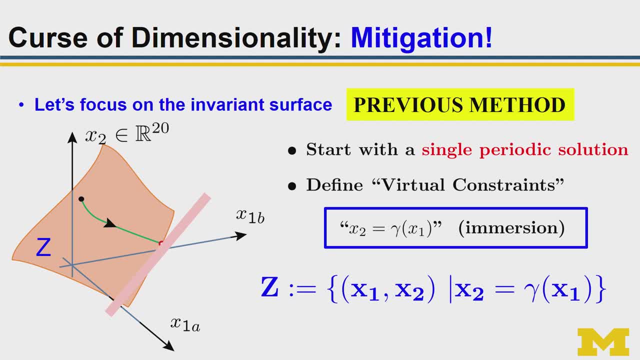 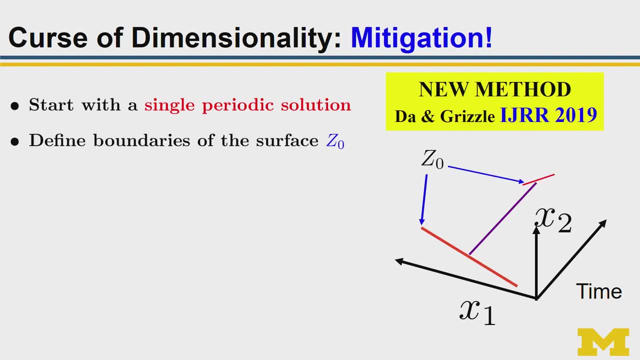 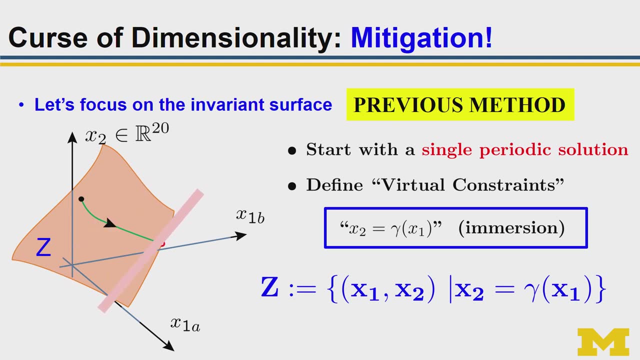 And that's what gives you the zero dynamics: manifold. Oh, okay, Here's what Dennis does. is he says: look, let me go back to this. Whoops going the wrong way, Wrong button, Bingo. So here, yes, this trajectory here meets all. 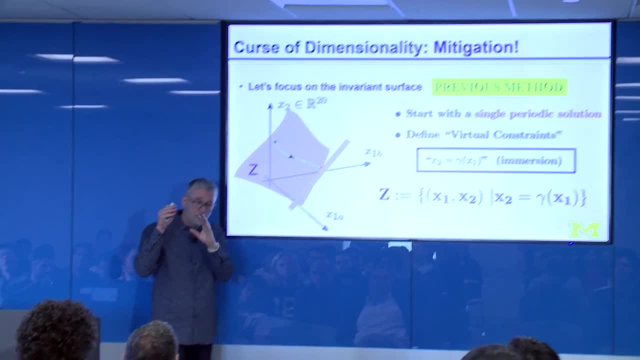 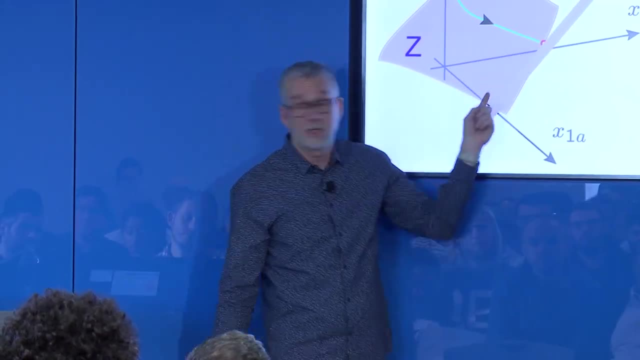 of my constraints If I want to go back to this trajectory. if they were inequality and they were strict, then I've got a small tube around here that worked. But when I get a little bit farther away, who knows if the new trajectory is created by this immersion. 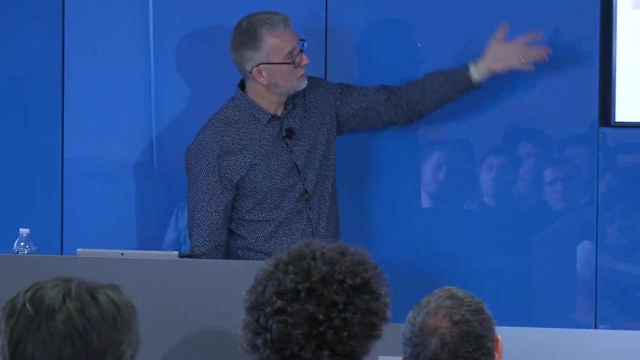 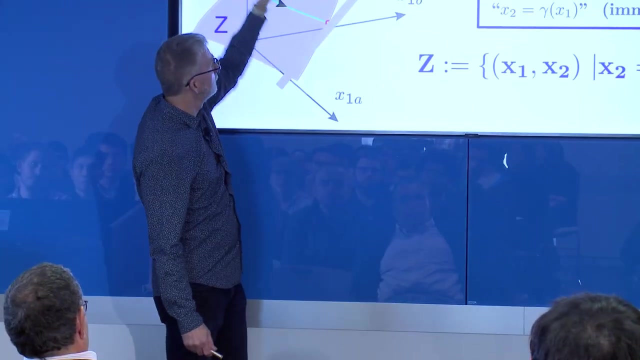 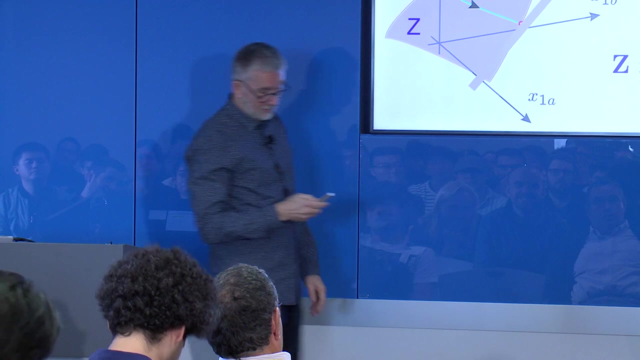 Even though they satisfy the mechanical model, they may not satisfy the actuator limits and the ground reaction forces. Okay So, these other trajectories that's called hope, Okay, This one, Oh, okay, Okay. So now what we're going to do is start. 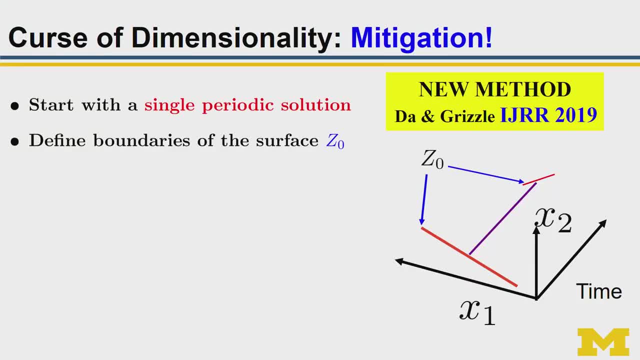 with a single trajectory And we're going to just take the immersion at the boundary, at the frontiers of the surface. So for this talk we're leaving open: how do you choose those frontiers? In the paper IJIR we give several solutions. 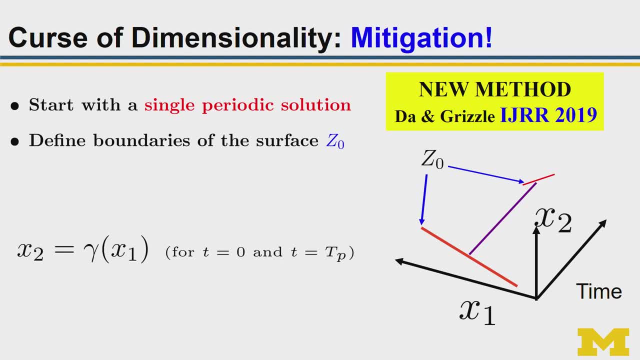 and we've got better ones now. But we've got some nice solutions there, And so we're going to have this immersion, but only at the initiating part of the trajectory and the end of the trajectory. In between we're going to use optimization, as before. 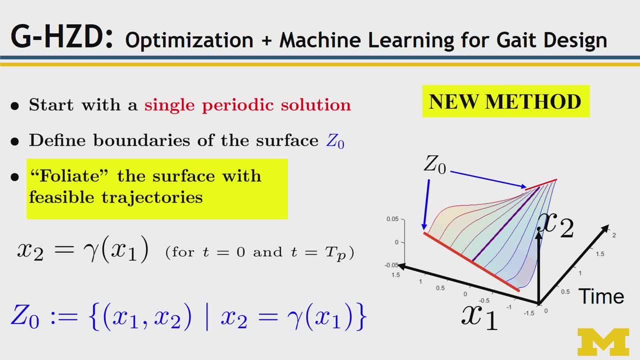 So we're going to take and foliate that surface with feasible trajectories, And so we're at the equilibrium point and we move out, And then eventually we get to where we can no longer satisfy the ground, reaction force constraints or the motor constraints. 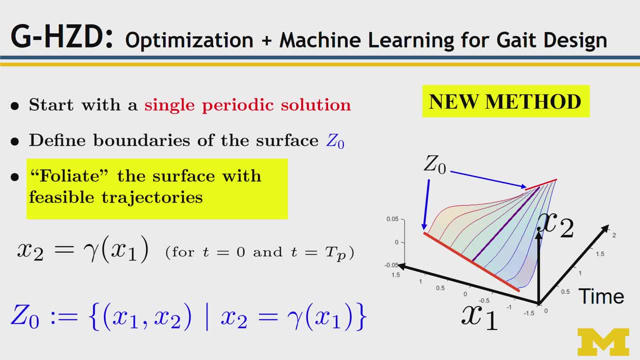 And so this is important information If we can continue our optimization out far enough to find where we fail. Okay, So how is this related to what Brent was doing, inspired by Hong Kai? Well, the disturbances that Brent was doing was creating a. 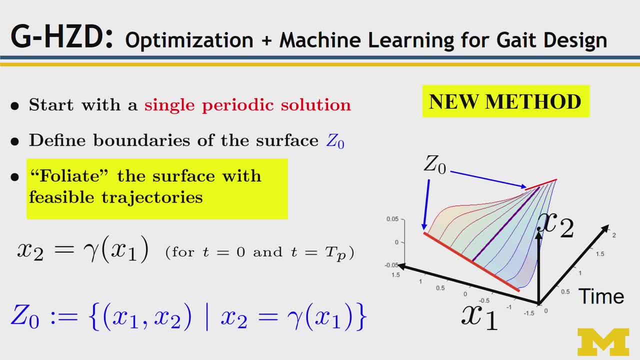 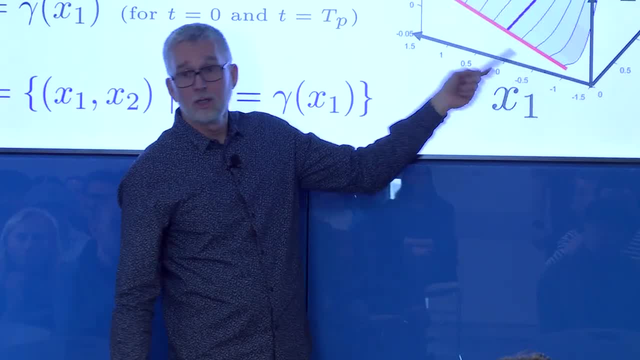 family of initial conditions from which the controller had to respond. We're doing it in a slightly different way, as we're doing a more organized search of the initial conditions and not letting them just be where you are. We're doing it far after a step. 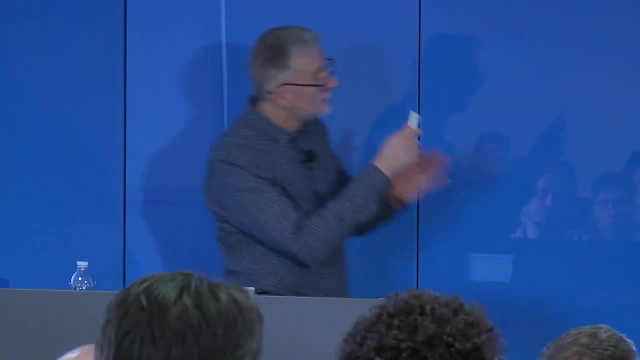 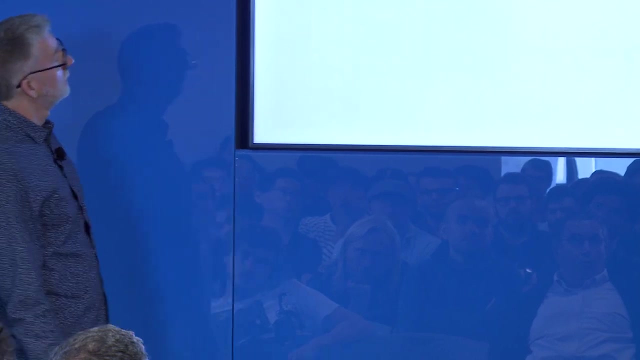 when the disturbance has been applied. Okay, So it's similar, but not Okay. So that's the way this fits together, But it's all about initial conditions, So the way you make this work, how are we doing on time? 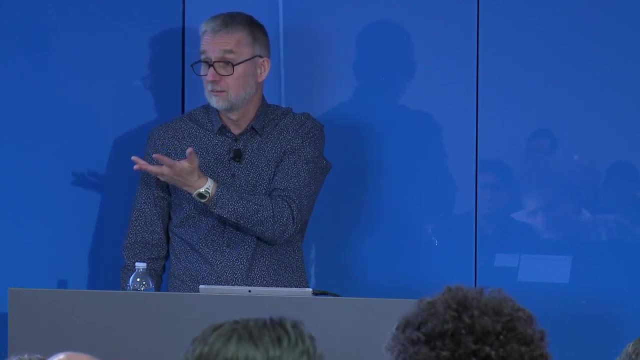 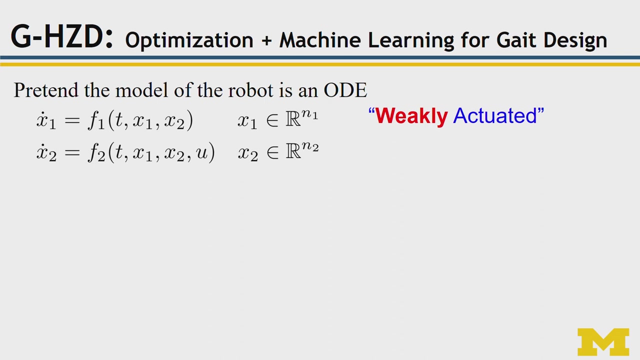 Two or three minutes were good, or Five minutes. Five minutes, Okay. So we're going to decompose the model into weakly actuated parts or weakly actuated parts. So what's strongly actuated on a robot? Big hip motors, powerful torque at the knee and stuff like that. 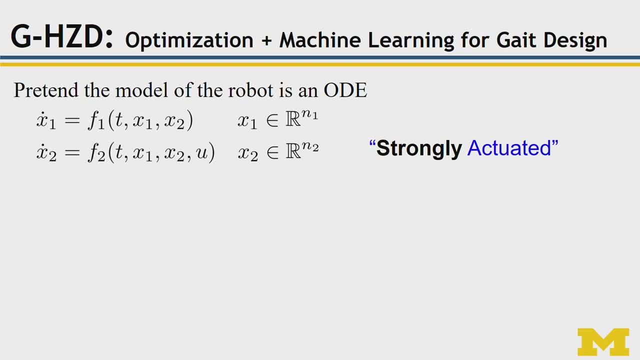 What's weakly actuated on a biped anyway? Well, the center of mass, unless you have a jet engine. so you've got direct connection to the world frame. you're very indirectly connected to the world frame through one leg on the ground. 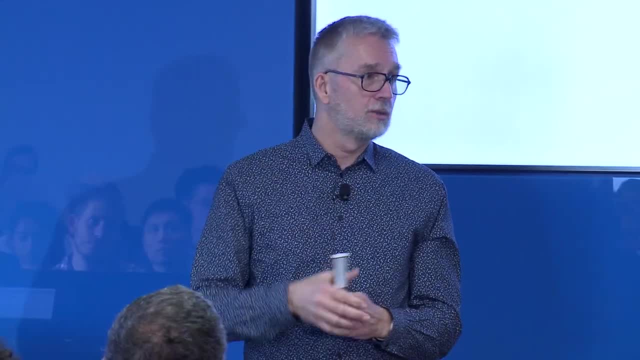 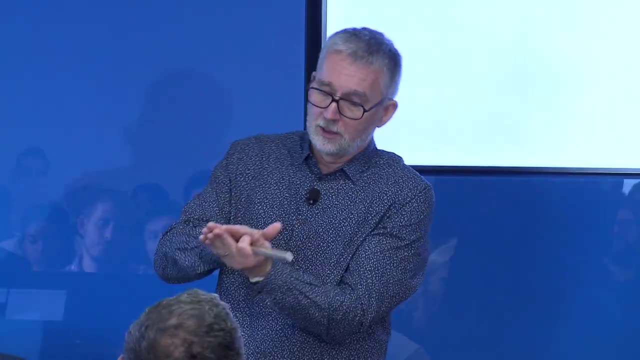 So that's a weakly actuated state. And if your ankle is not actuated, then it's literally an under-actuated component. But your ankle torque on a biped is limited by how much foot roll you can tolerate. Okay, So you'll have weakly actuated states. 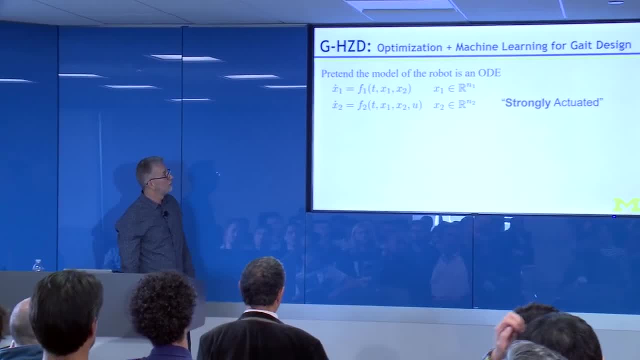 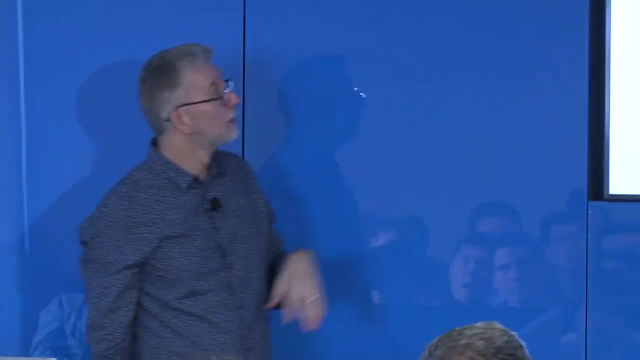 and then these powerfully actuated states. And the fact is, the weakly actuated states are low dimensional, So in Marlowe it's like four, Cassie it's six, Okay, Whereas X2 is 12 on Marlowe. 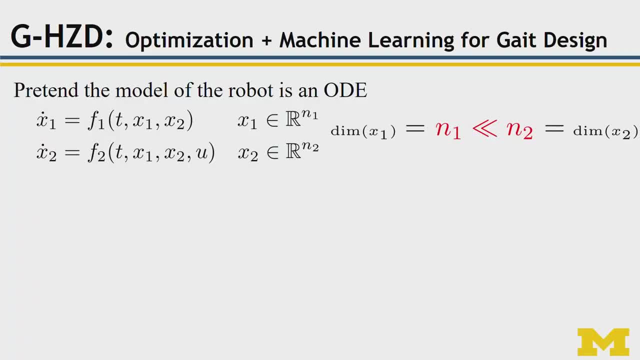 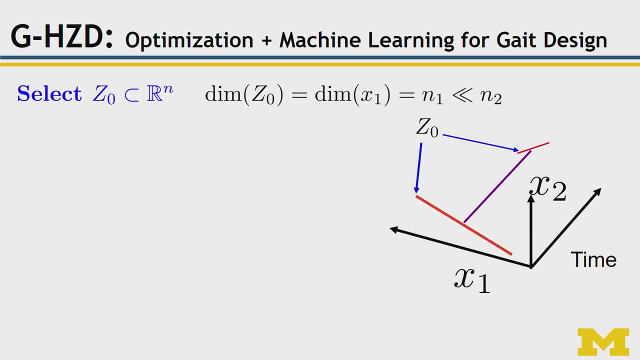 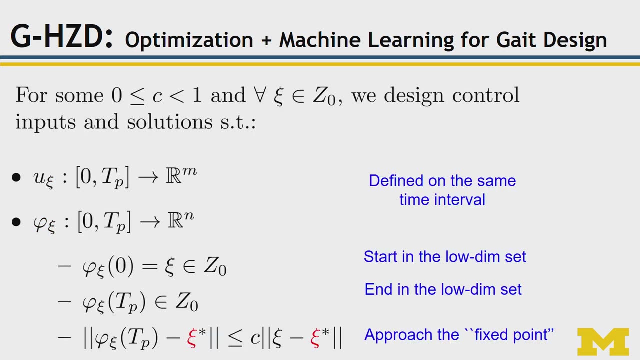 And it's like 20 on Cassie. Okay, So it's a huge dimension reduction here. So we design a periodic orbit, Just as before. we foliate the trajectory with solutions that satisfy the same conditions you guys saw before. 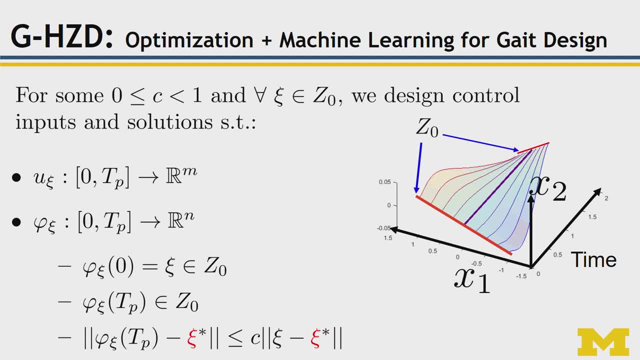 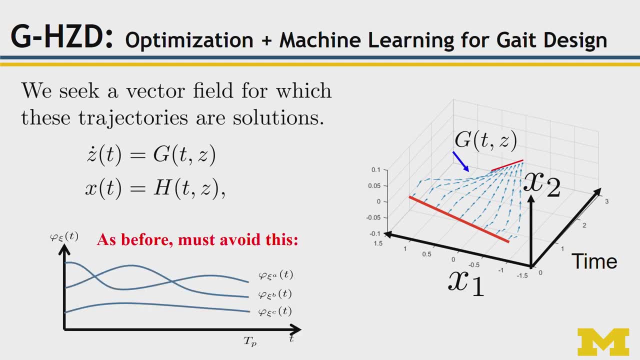 the same attractivity. We build that out and then we want to find a vector field. Now the problem is, we don't know how to find a vector field. So we're going to try to find a vector field, And the problem here is a little bit more challenging. 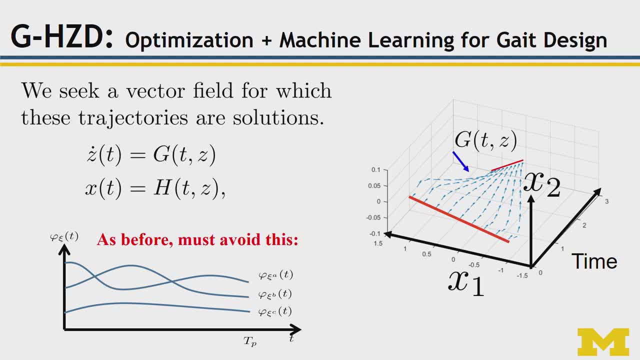 because in 3D these are not crossing Right, But let's project them to the plane, Okay, So you can easily get trajectories that are distinct in a higher dimensional surface, And when you project them, you end up with this kind of stuff. 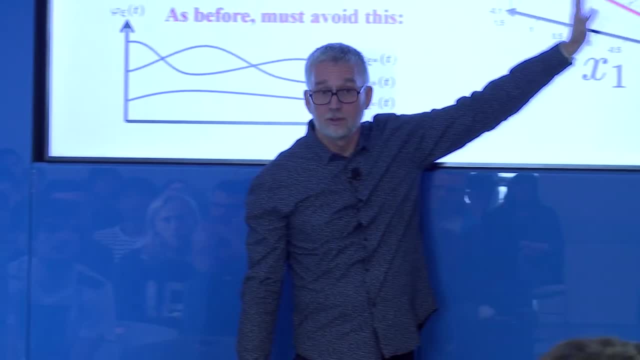 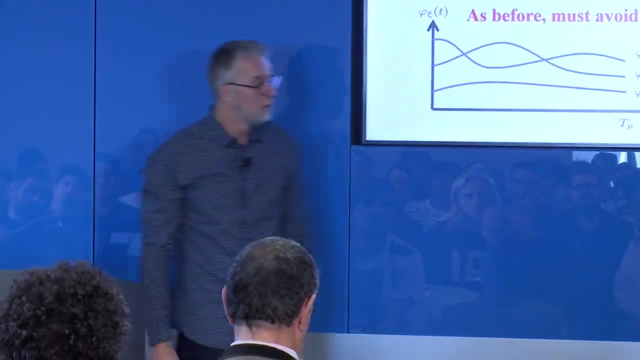 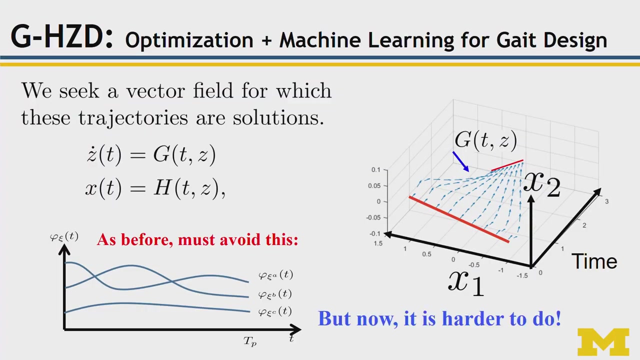 And that's a topological impediment for finding a Lipschitz, but it's not always to the solutions here. Okay, So you have to have that stuff in mind when you're doing your problem and setting it up. Okay, So just to say that we've thought about this a little bit. 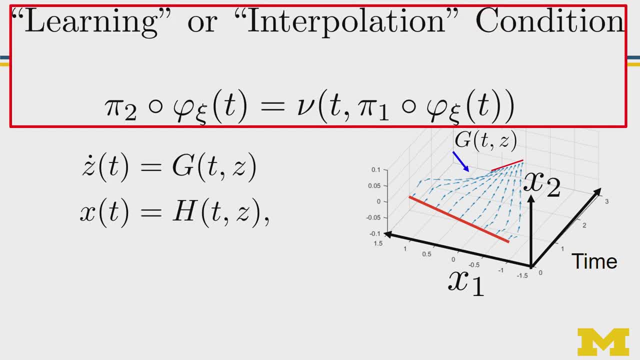 Okay, So it's harder now. You need to be a little bit smarter or a little bit luckier. whichever one works for you. There's a little bit more complexity in the notation. Okay, Because you're working with projected coordinates and stuff. 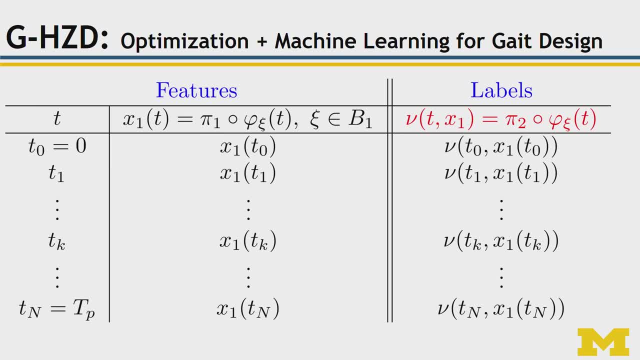 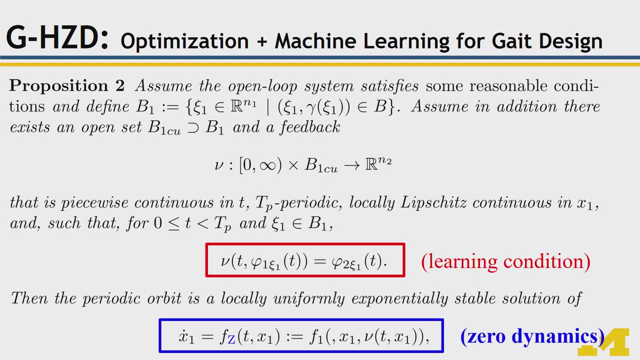 But you build up the same type of- you know, supervised machine learning And then you get a theorem that says: if you can build this bundle of trajectories and you can find a function that satisfies this projected version of the learning condition, then you have created a zero dynamics. 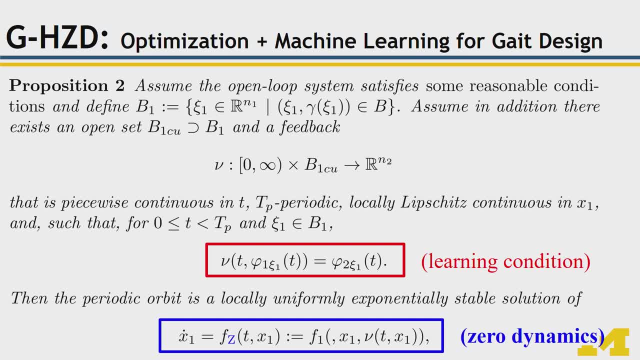 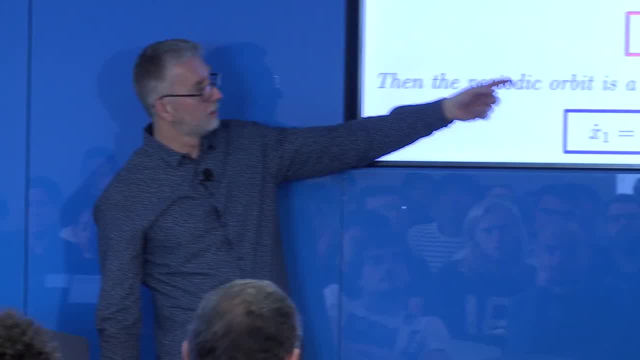 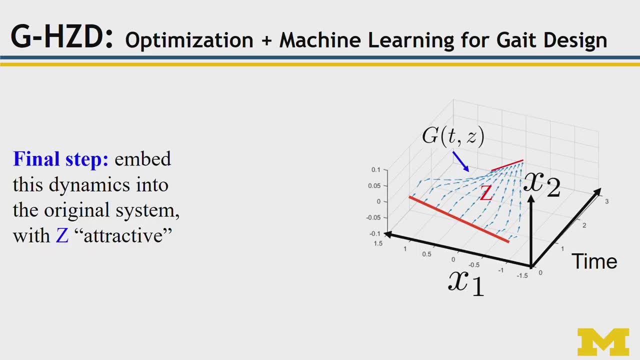 much different than any one I ever designed. This is a Dennis design, But you've got a low dimensional vector field on this manifold and it has your periodic orbit as a locally exponentially stable solution. And then, if your transverse dynamics are nice, 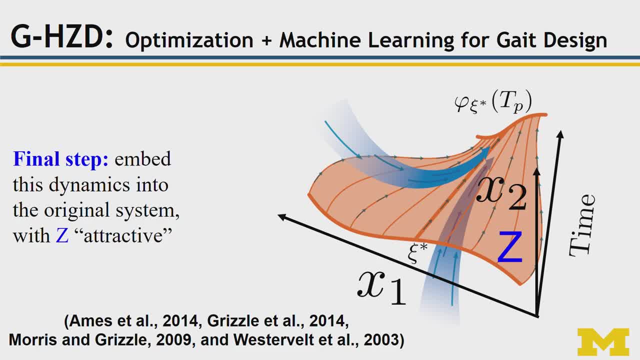 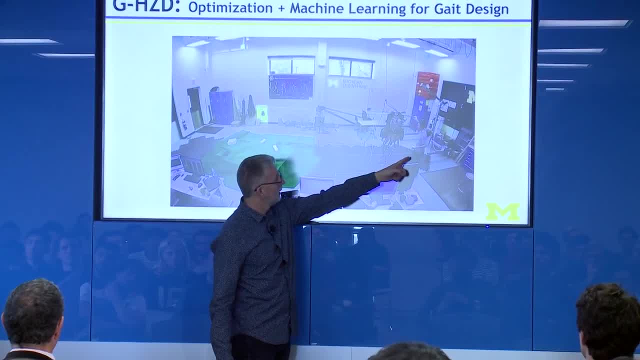 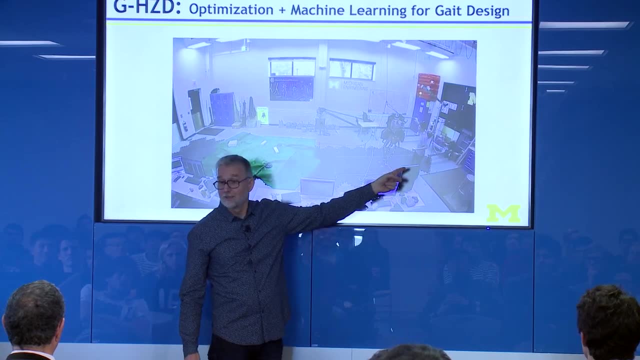 you can embed this in the full model and make it work. And so here's Atrius, Here's Dennis, Here's a student practicing the buddy system. He's supposed to be watching everything Dennis is doing and protecting him right. 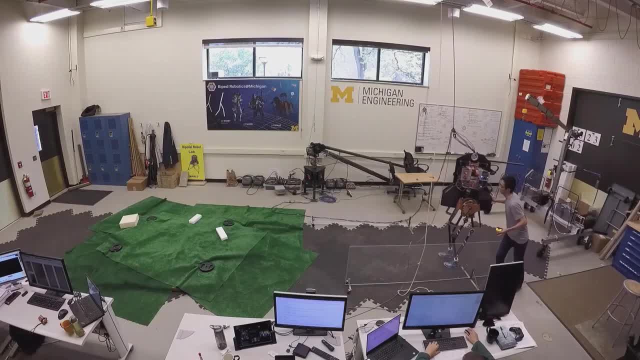 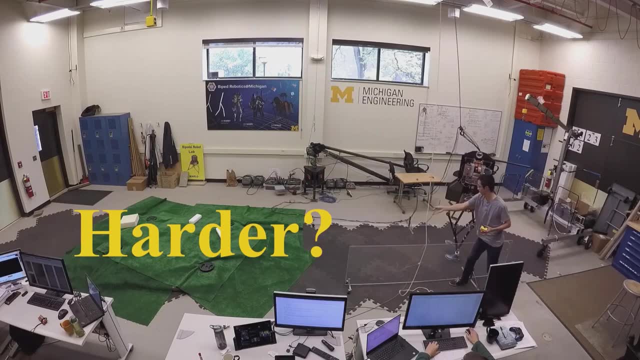 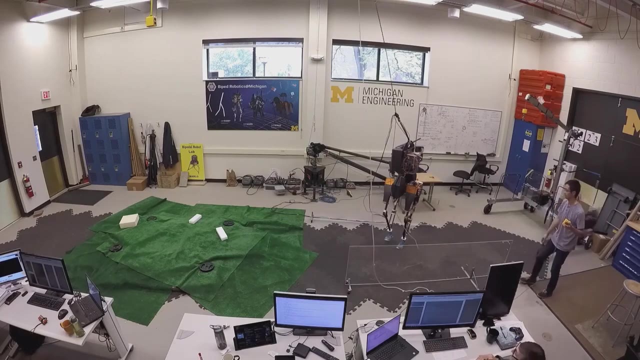 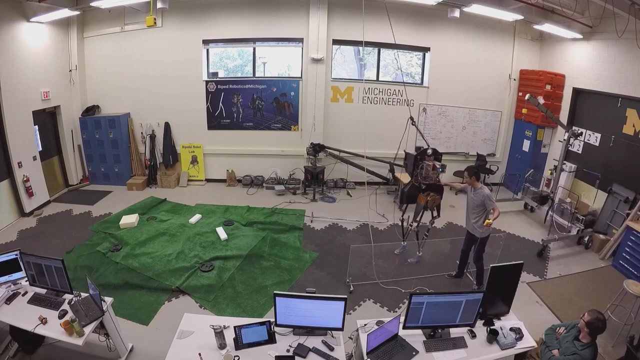 That's Ross Imani, okay, So you know, I've seen Dennis run hundreds of experiments, Boring, boring until it's not okay. Whoa, Something interesting is happening here. okay, I think this is Dennis owning up on film. 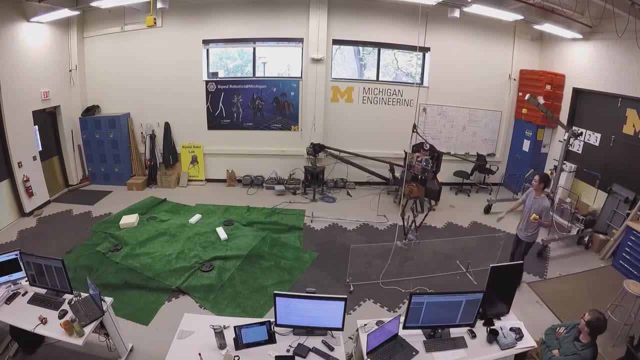 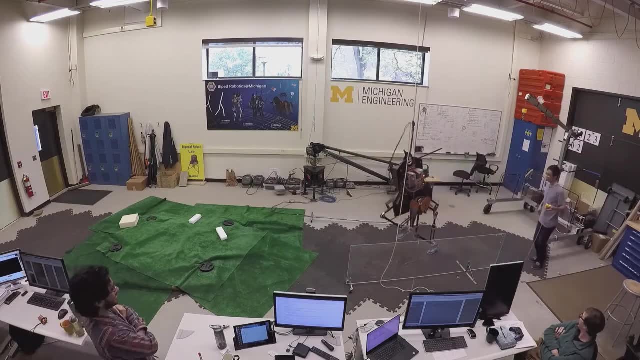 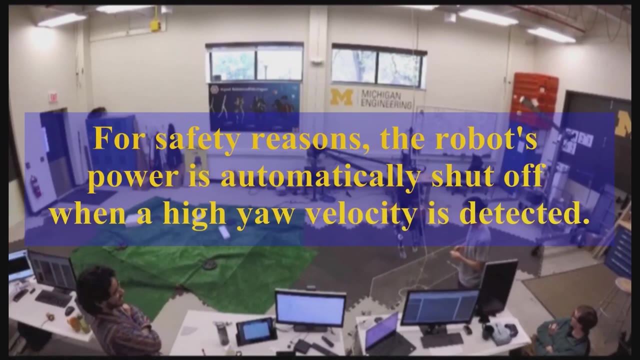 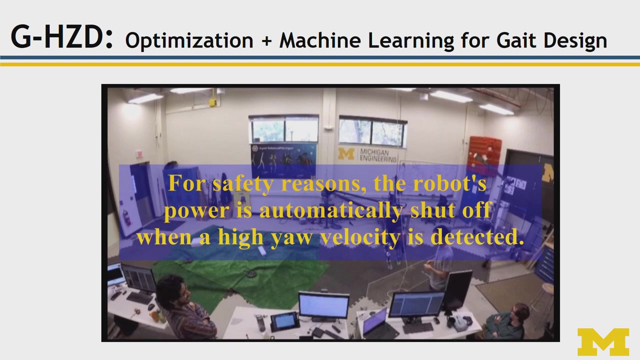 and some machine learning going on here, And so we have a safety system that, if the yaw rate gets high enough, we shut down the power to protect the robot. Seem pretty smart, Sungbae, Yeah. So that's what happened there. 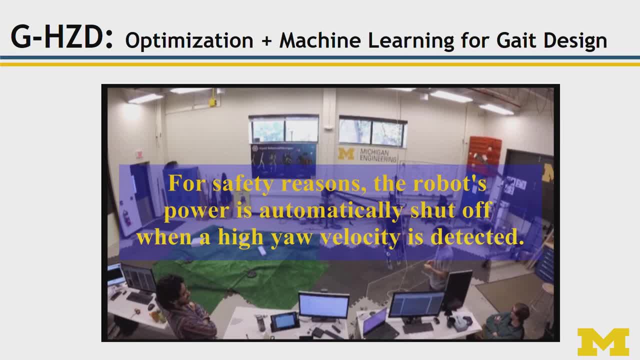 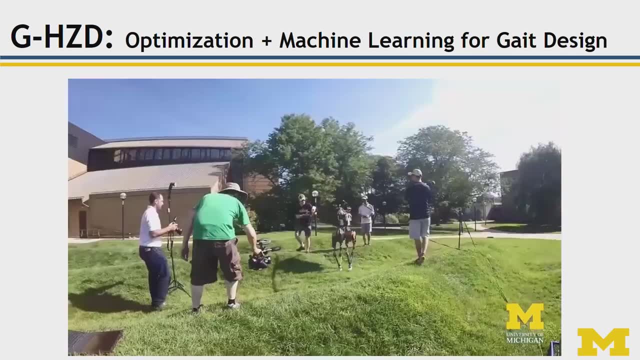 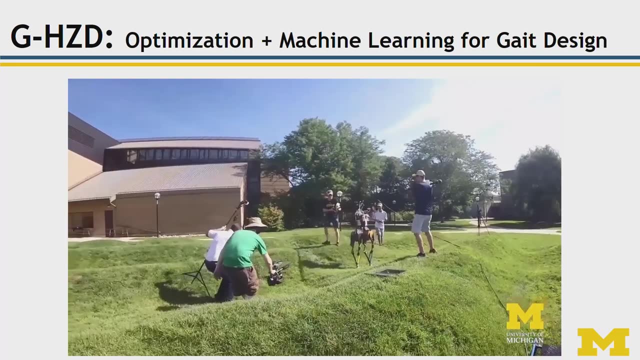 Dennis put torque on it and it spun around and bingo, Okay. So Dennis was able to go on the wave field with his control ideas. We can only do the small humps, but remember that's where we caught fire before, So we got all the way down. 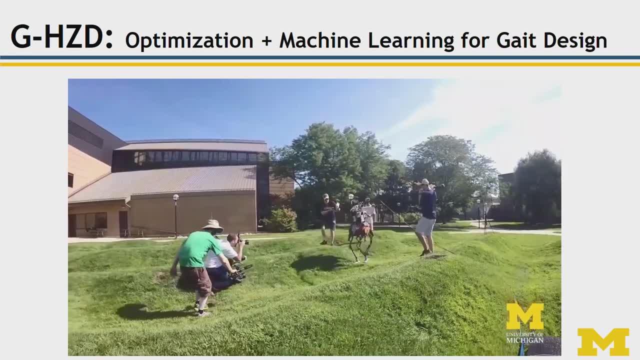 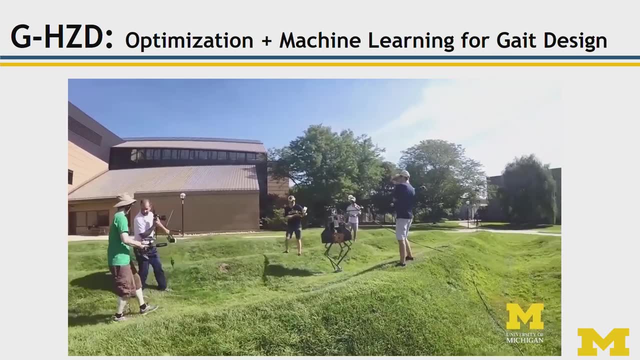 Discovery Channel is not there, It's just local people from the college. okay, So maybe that's what took the tension down on the robot. Maybe it has nothing to do with the better math, It's just that the media was not present, you know. 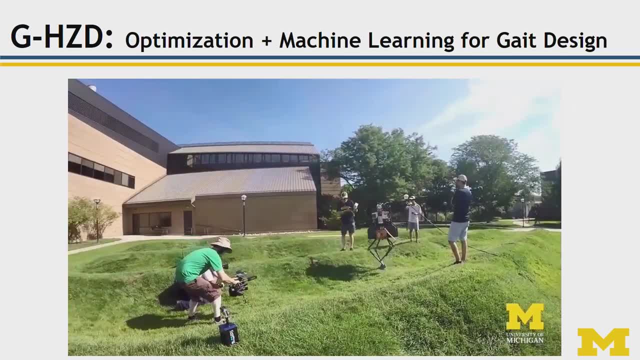 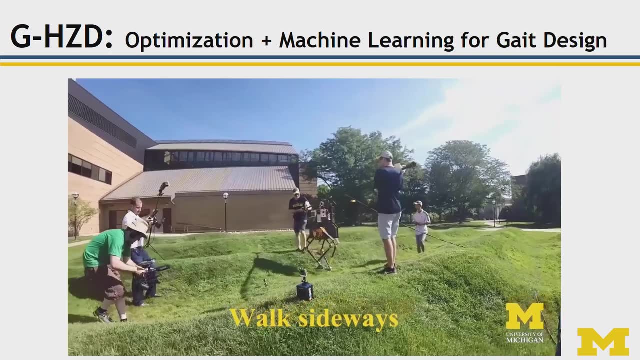 I'm open to all sorts of explanations for this. Now, Marlo doesn't have a yaw control in the hip, so you can't just turn her, but we have omnidirectional walking, So if I want to go over here, I can do it like this. 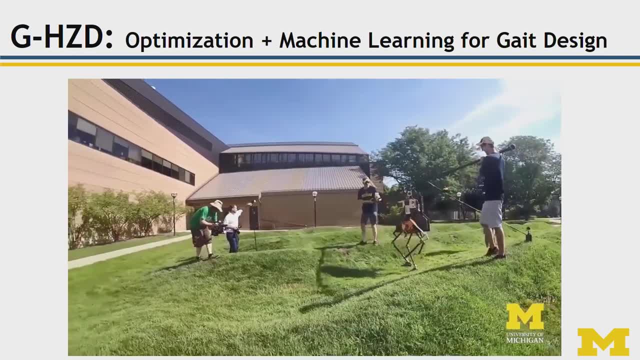 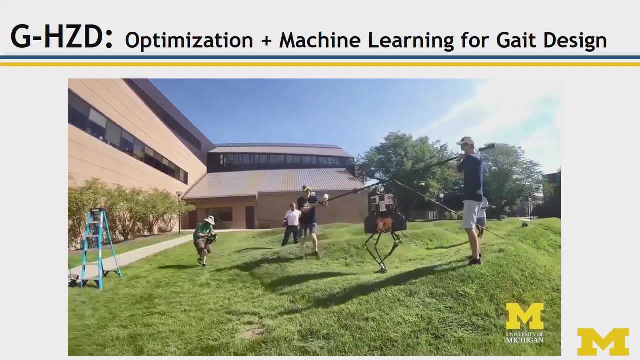 and then I can do it like this. So that's how we're controlling Marlo. It's already showing very amazing robustness, okay, And it looks flat in between there, but that's just because it's being cut with these little. 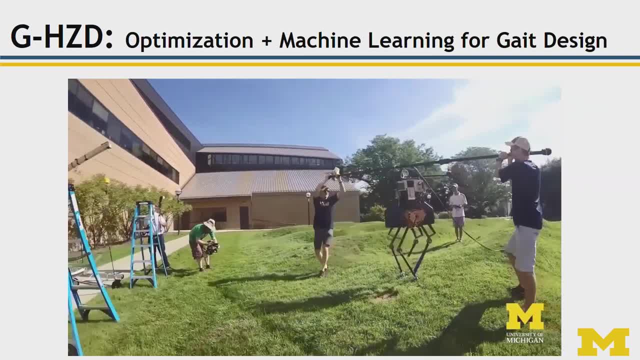 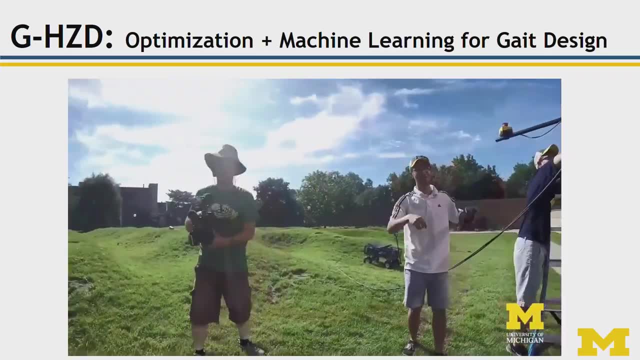 weed whackers. It's full of holes. okay, It's a mess. If I blindfolded you, you would be in the hospital with a torn ACL for sure. okay, And so we got there and back and yeah. 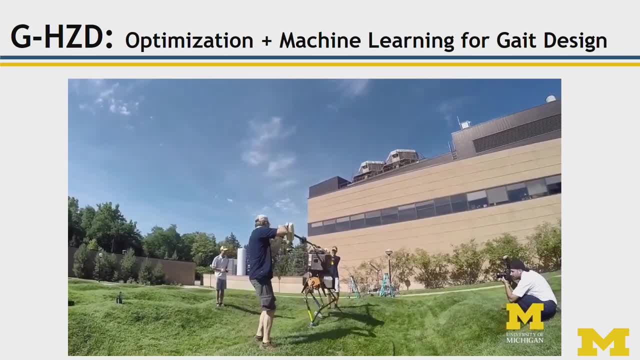 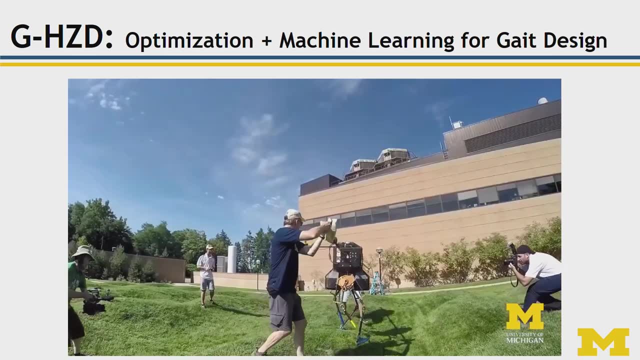 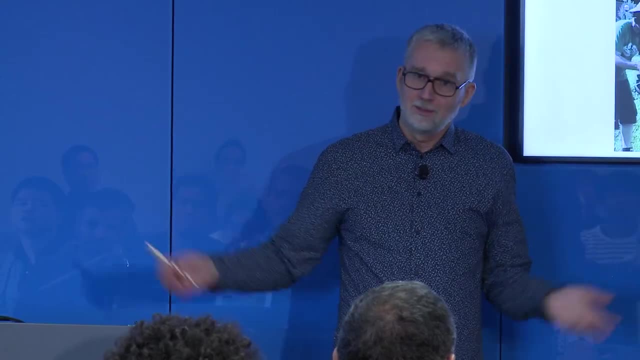 So could we do something on the big humps, okay? And then we just snapped a leg in two And the problem is the depth from the top of that hump to the bottom is longer than the leg. So this is showing a limit of blind walking, okay. 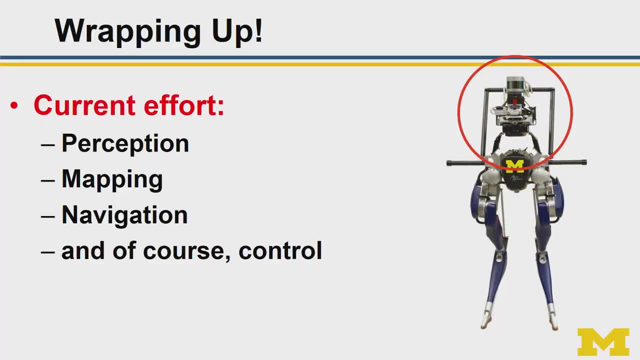 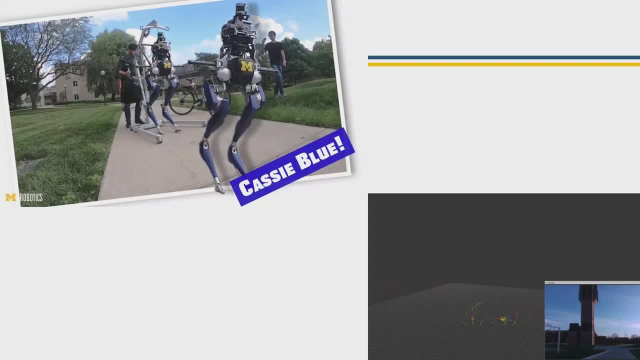 You can't go blind walking forever and that's why we've gone with the torso, and you saw at the beginning some of the stuff that we've done with that, And I'll stop here. People can watch the video and I can answer questions, okay. 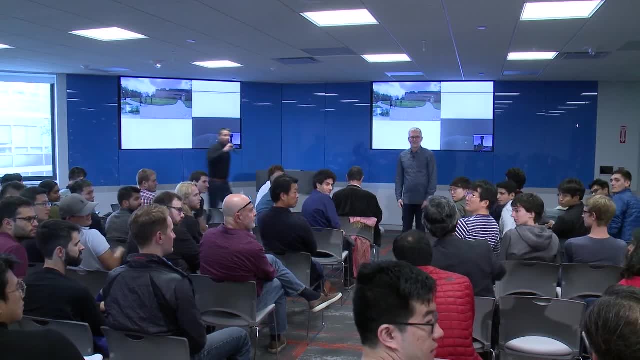 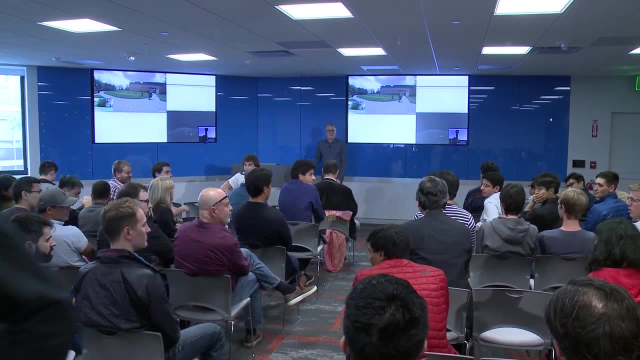 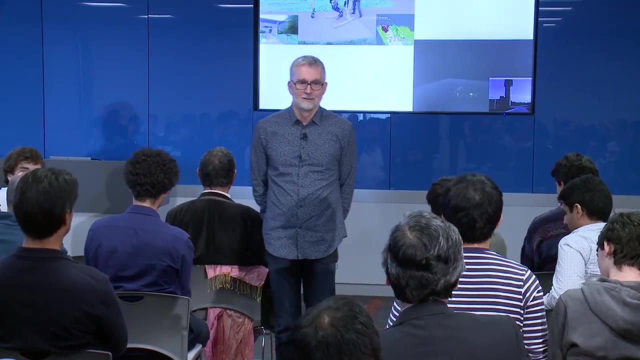 Hey Harry, Thank you, I learned something new, so I appreciate it. Oh, This may not be your question, but just, you know TP, that period, you know what happened if TP fluctuate and is any mechanism to regulate the TP? 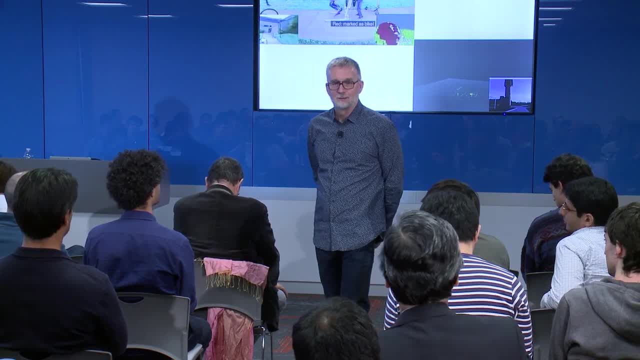 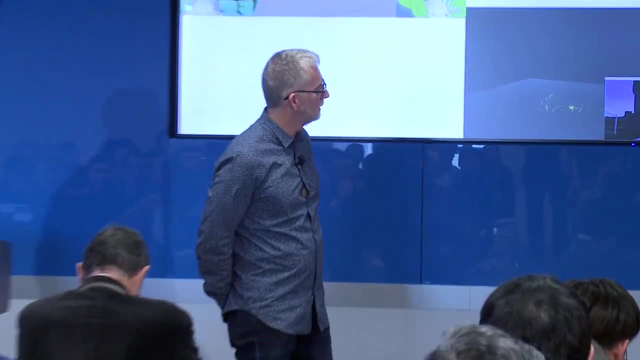 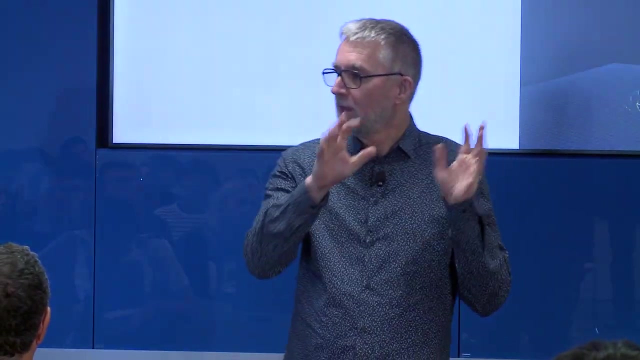 or you know, variation of the TP is not, you know, really bad from the theoretical viewpoint. Yes, we try to turn those into basically event-based decisions. So that's TP is the time On the robot. it's more of an event-based thing. 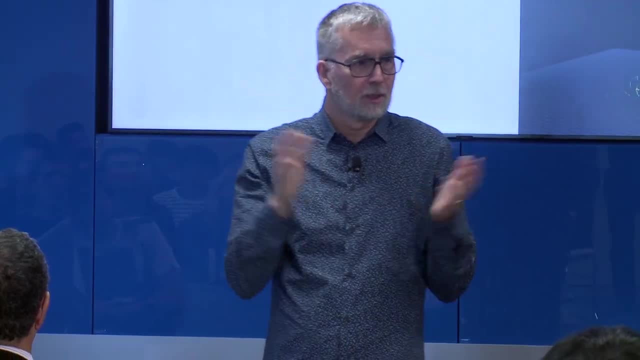 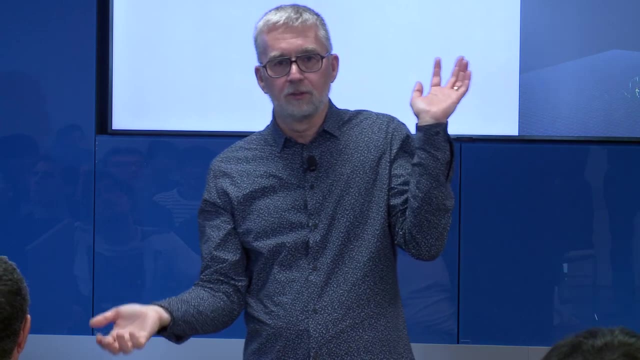 So if the robot slows down, it's not terrible. But also, what we'll do is we'll design that manifold. you see, We'll design hundreds of them for different walking speeds, And what we actually do is during the gait. 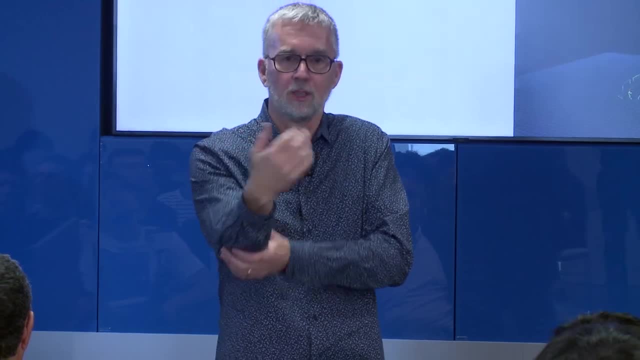 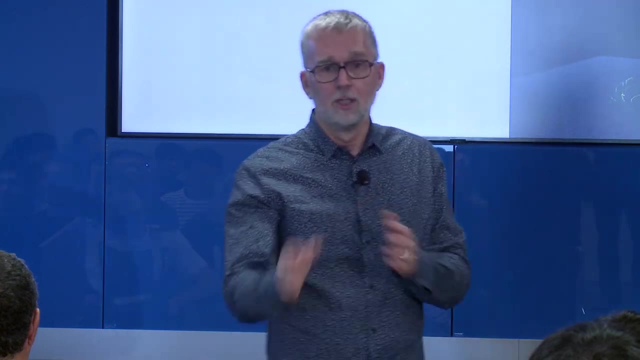 we are interpolating into the correct manifold, which does correspond to the walking speed, which is what's setting the period it takes for the next foot strike. So the foot strike is taking place within about 5% of what the nominal period was designed for. 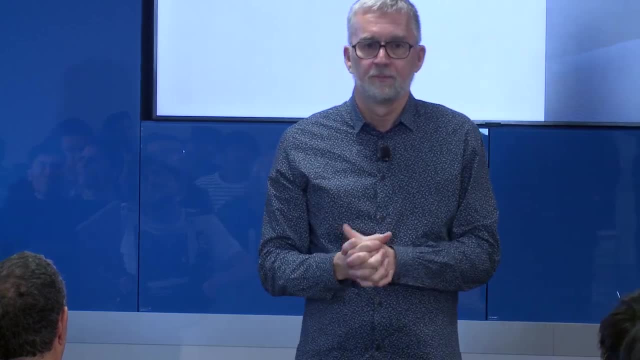 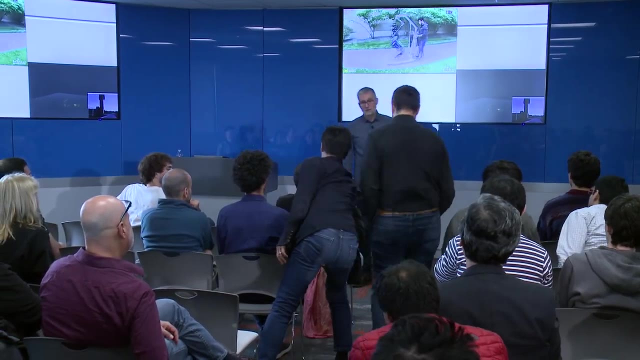 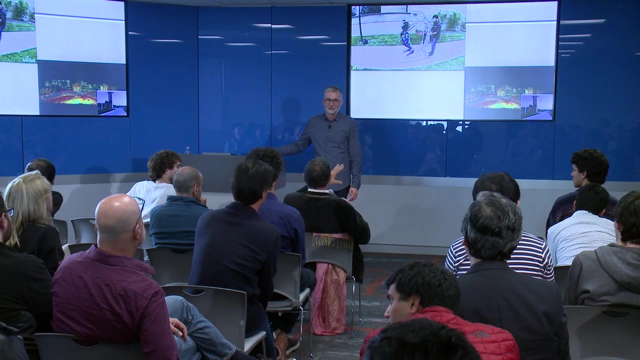 So all of that works out well. People won't let you talk without a mic, Jean-Charles. You show experiments at the end. Is there a way to kind of know in advance the robustness to terrain and stuff like this to quantify that? 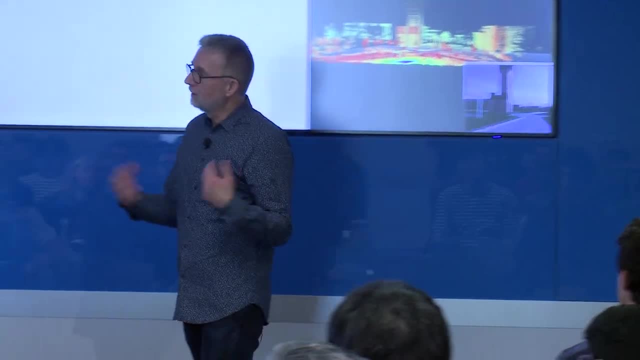 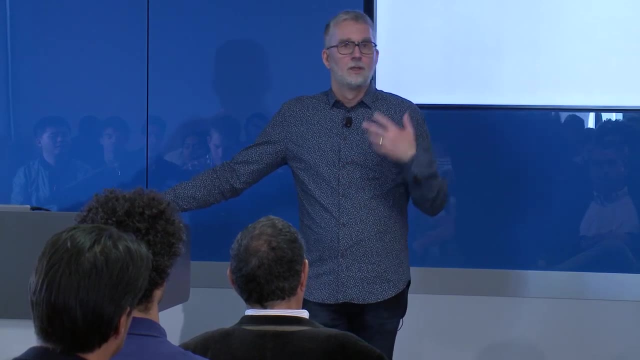 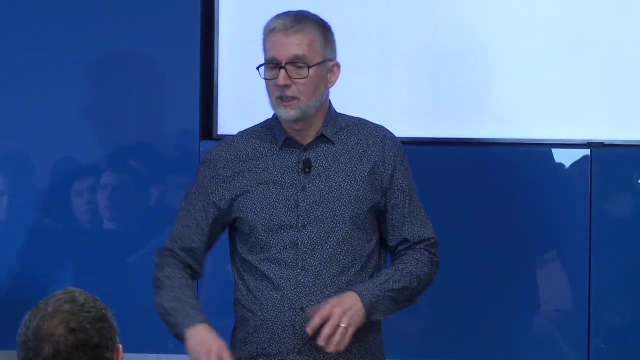 So our ways currently are very indirect. I mean, this is what we're doing. This is really brilliant work, but it's certainly not the end of the answer is that we have learned that it's better to be robust to slopes in the frontal plane than in the sagittal plane. 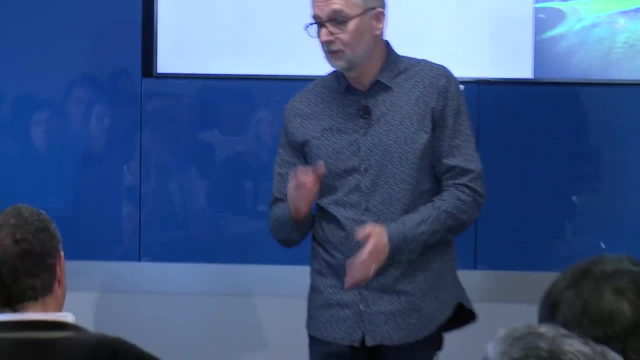 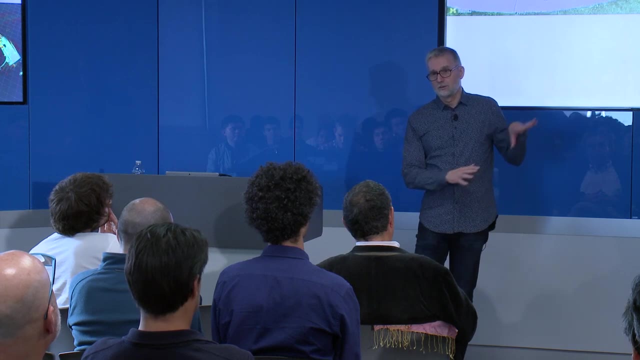 just because it's harder to move this way than it is this way. This is a very symmetric move, So we have understood that and so we build in a lot of robustness to lateral disturbances and we spend less time on the others. 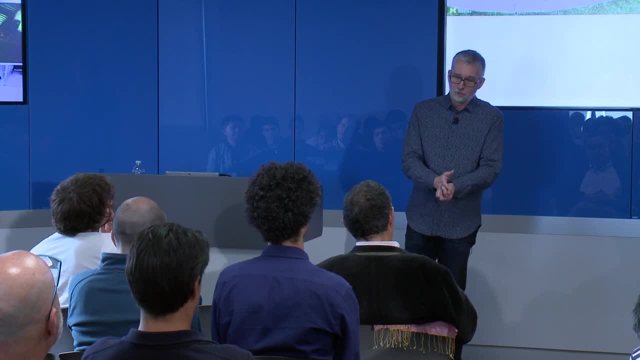 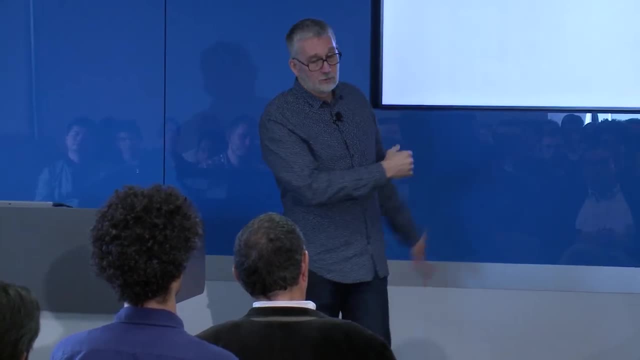 And so that will vary for every robot. So what I'm saying? the answer is no, We don't know ahead of time. We can simulate it and have a guess, but from working with this robot and then working with Cassie, 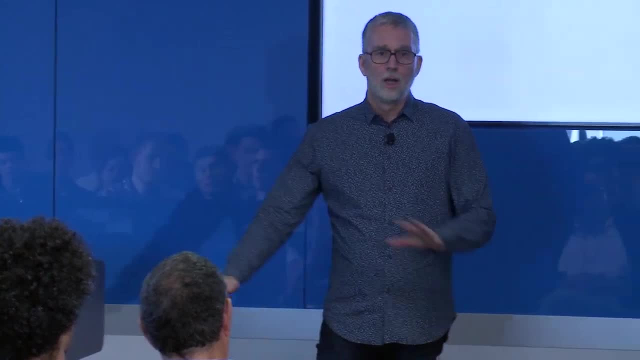 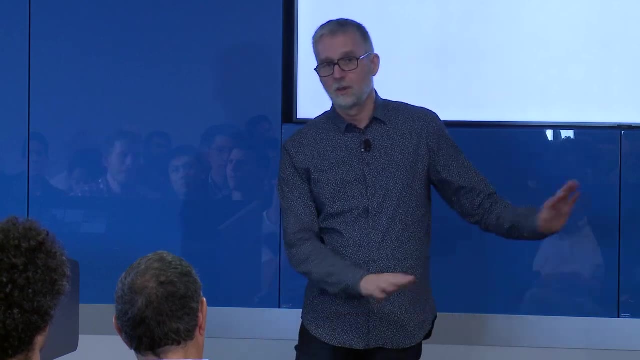 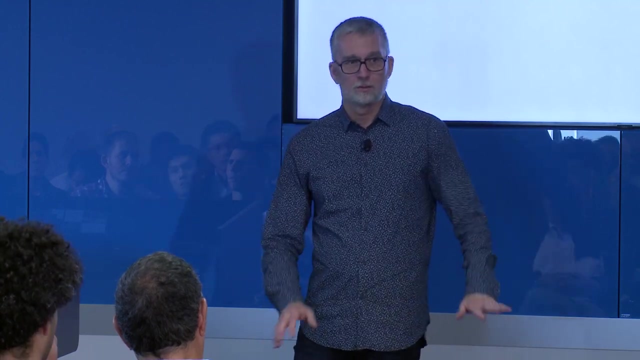 it would be different on Atlas, It'll be different on quadrupeds. Where is the weak point in the motion? that the legs put new forces onto the robot and then you have to focus your robustness in where the mechanics has a difficulty getting rapid footfalls. 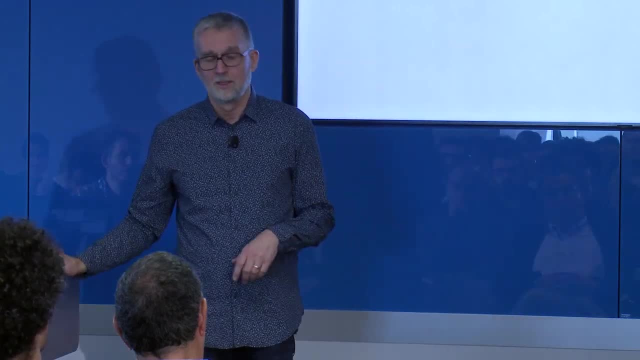 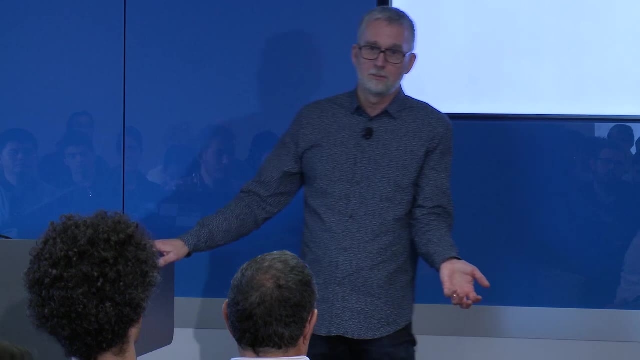 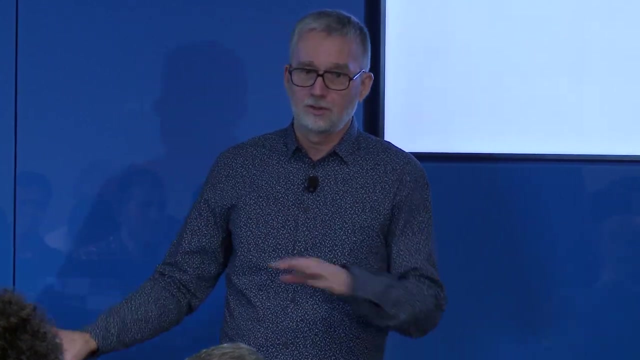 to create new forces on the center of mass to keep you upright. It's still art, but this makes it much faster to go from concept to a successful experiment. so I think that's the role of mathematics. In the end, we would love to have a certifiable theorem. 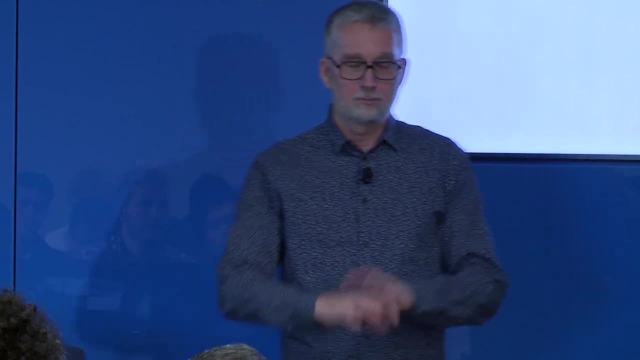 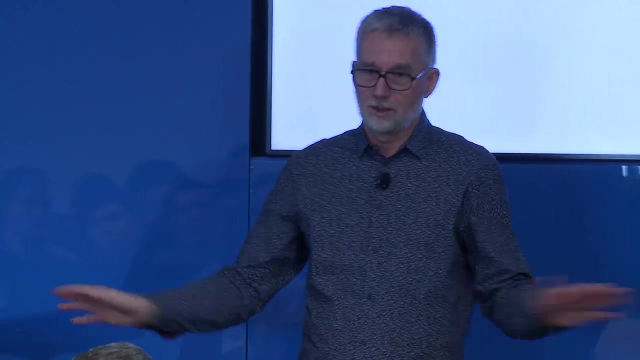 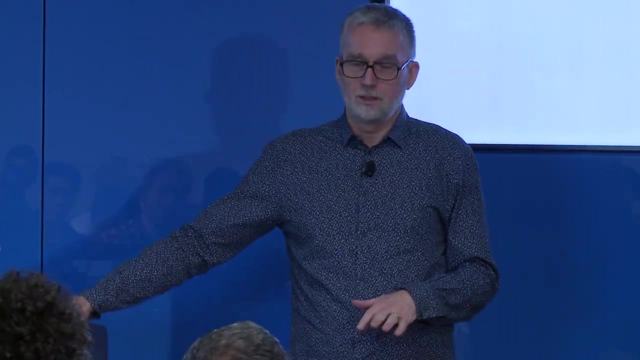 saying for all of these possible terrains I described by splines and I put rates of changes on the normals and things, but we're not there, We're a long ways from there, So this is not certifiably a correct solution by any means. 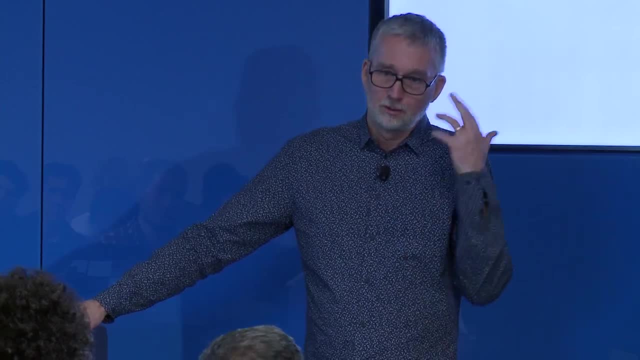 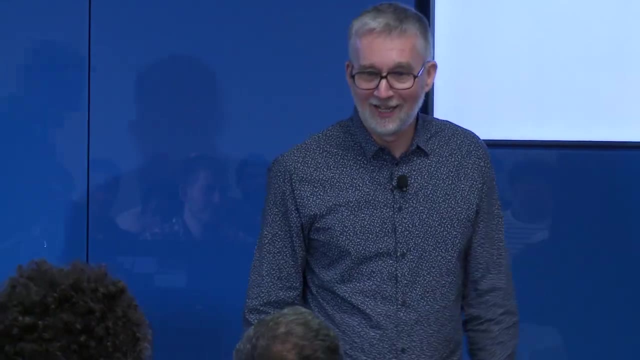 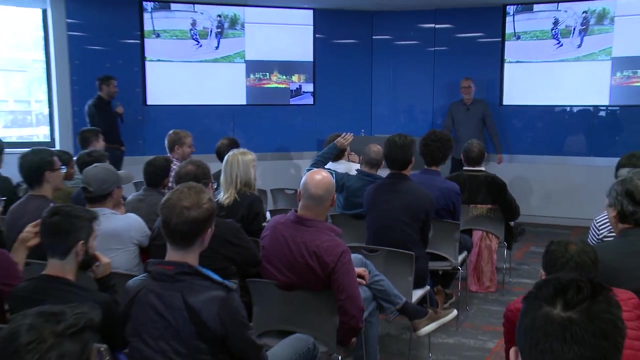 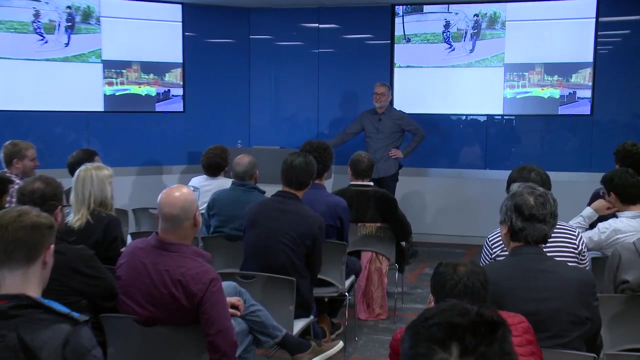 It's hacking with fancy mathematics and good insight built into it. I just admitted that on film. okay, And it's all your fault. It's all your fault, Jean-Jacques. Thanks for that. Thanks for that honest answer. So in propositions two and three: 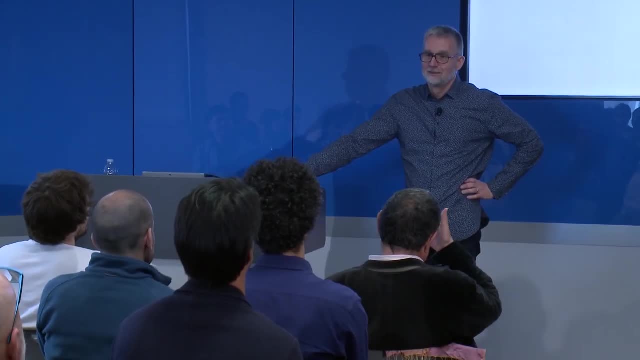 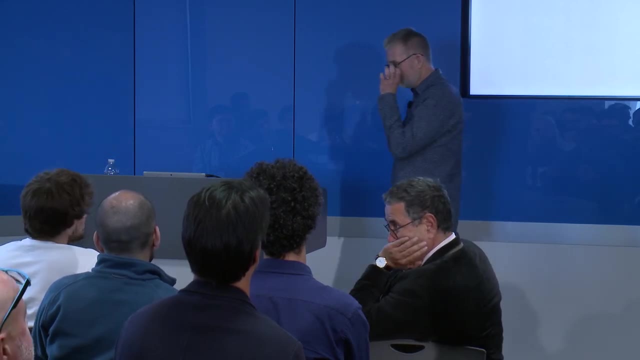 you had the learning condition for phi and nu, so it seems like that's predicated on how well you can do the classification that you showed. Do you have any sort of intuition or insight into how well does it classify that you're trying to actually learn? 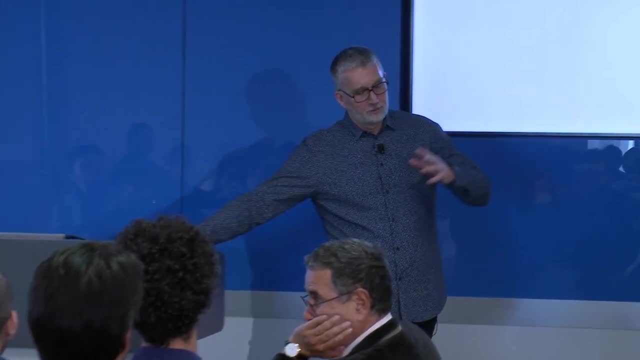 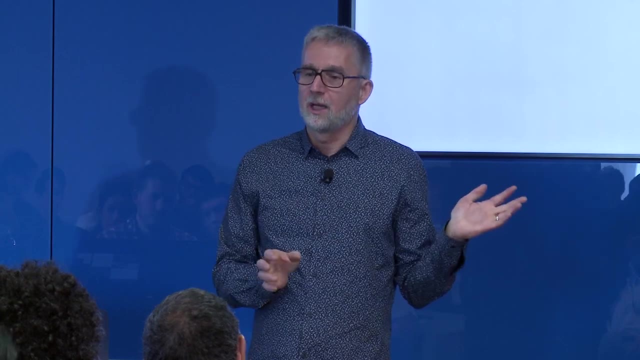 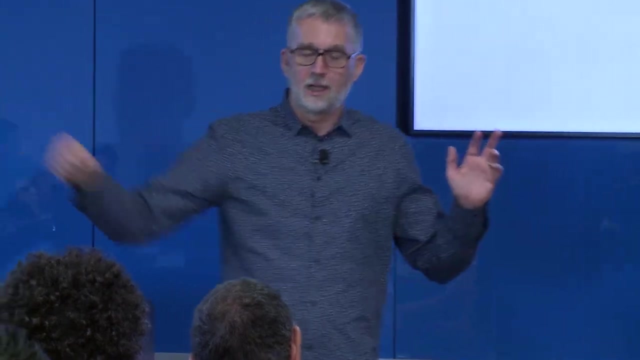 Yeah, so imagine that the boundary condition you have is coming from the vector fields and you're getting feedback, And then you actually just took that feedback and moved it forward and got the vector fields from that, and then they would all be distinct, okay. 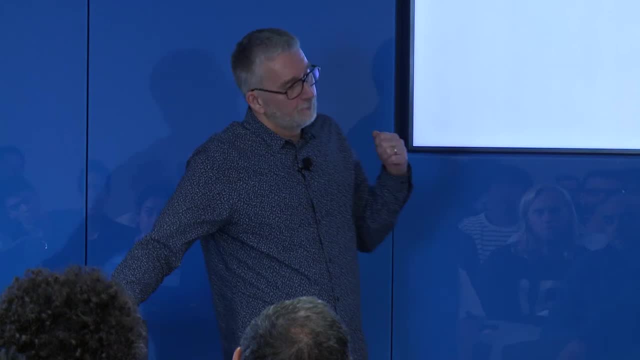 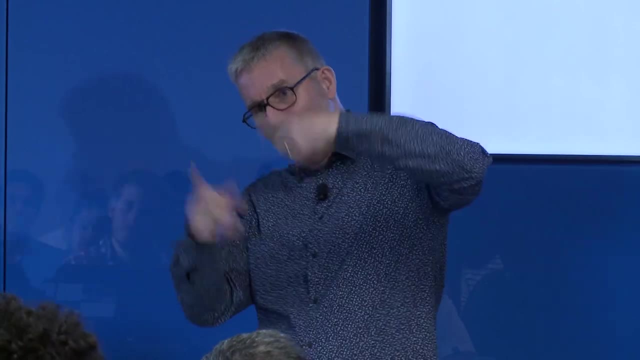 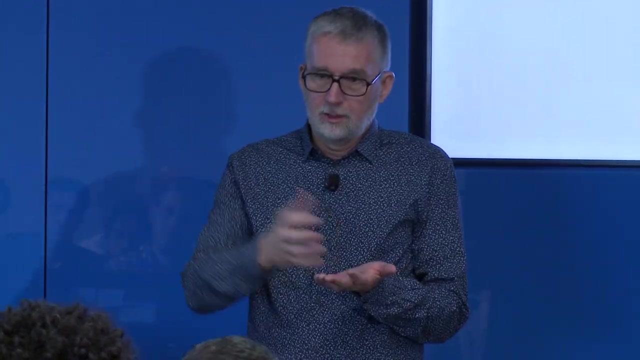 So that would be a Hamilton-Jacobi-Bellman type thing. So if you had something that's like a feedback, that you could do it. but we're trying to build this, so this is you know. so what we're doing now is: 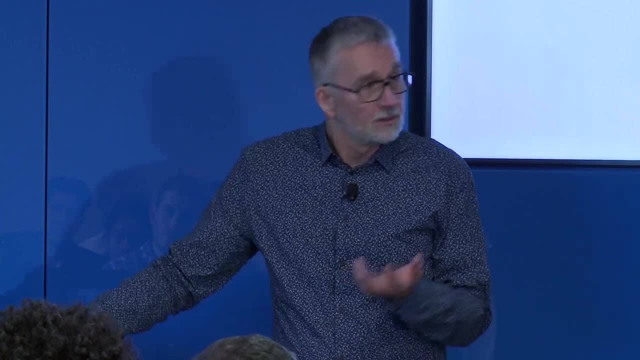 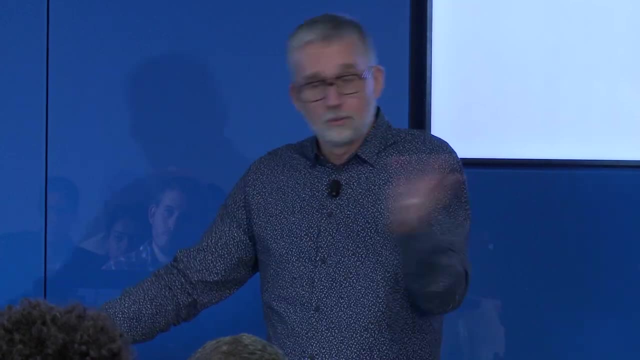 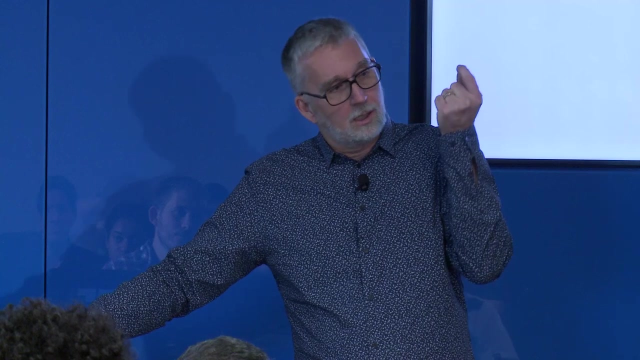 we're trying to theorize along one of these periodic trajectories. Okay, so fine, you solve the time-varying hybrid LQR problem, You get a cost function and we throw away the feedback. And then, to design the manifold, we fix the weakly actuated states. 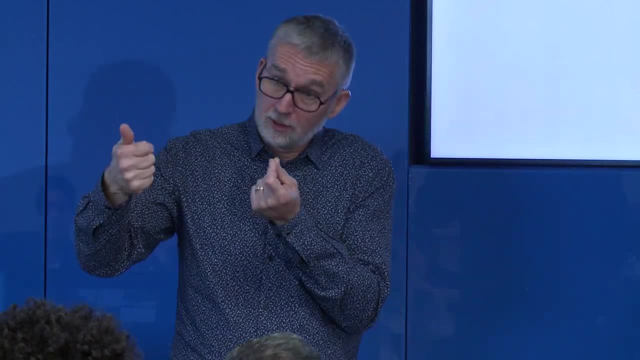 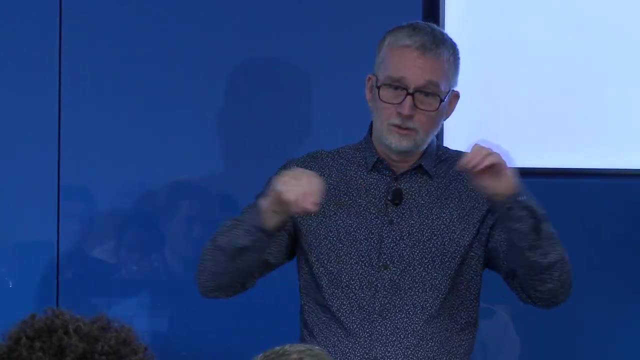 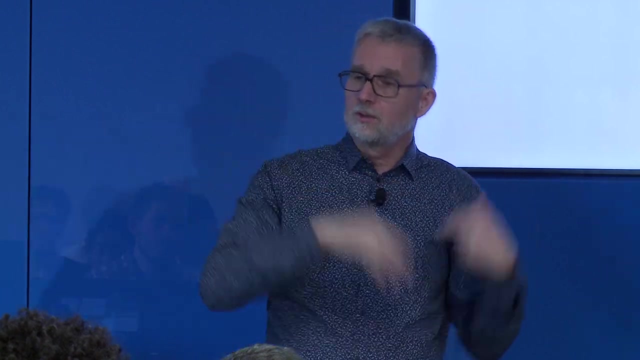 and then choose the strongly actuated components to minimize the cost to go from that point, And then we'll include the physical constraints on the nonlinear model when we're doing this. So we're using the LQR to give us something that's like a Lyapunov function. 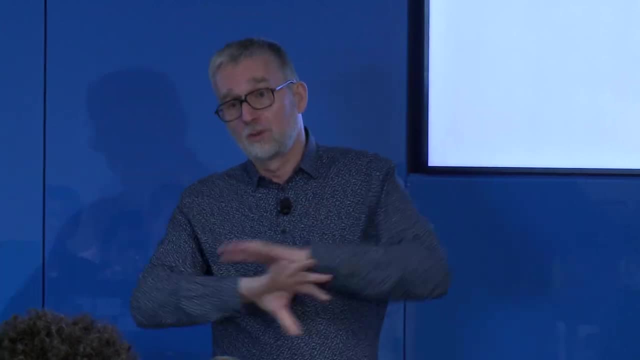 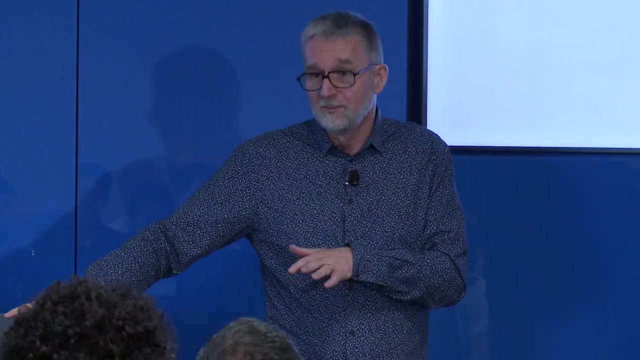 a controlled Lyapunov function. And if I had a true controlled Lyapunov function and I were doing that, my trajectories, I believe I could prove, would be distinct. So that's what we do. What Dennis did was something simpler. 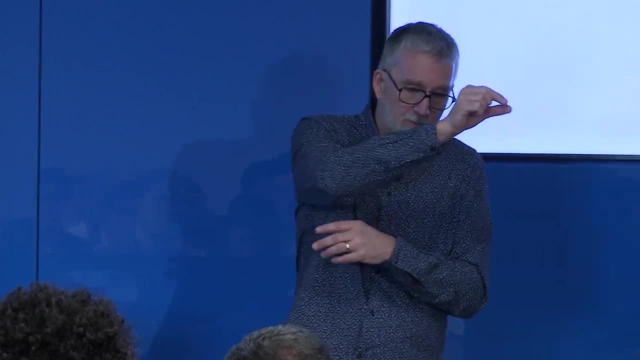 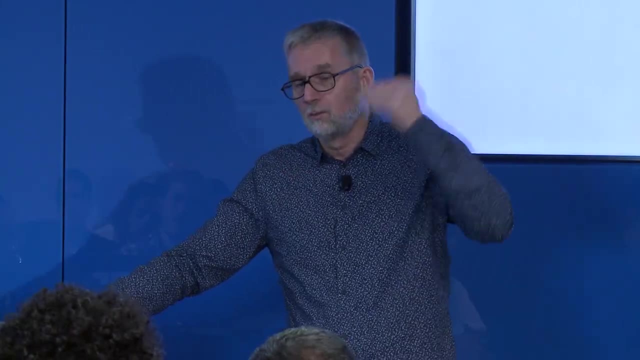 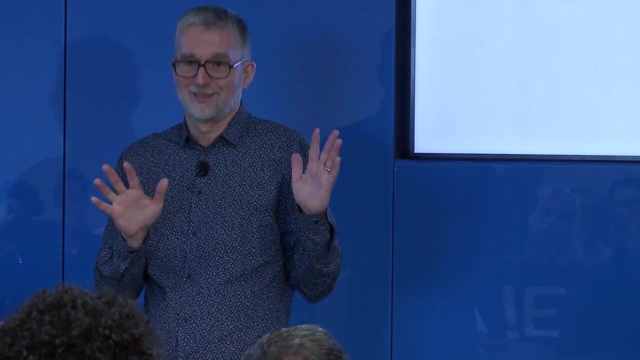 He said I'm going to have a bunch of equilibria corresponding to walking in different directions at different speeds, and I will build these surfaces from one set of these to another and piece them together, And so that gave him kind of nominal stability. 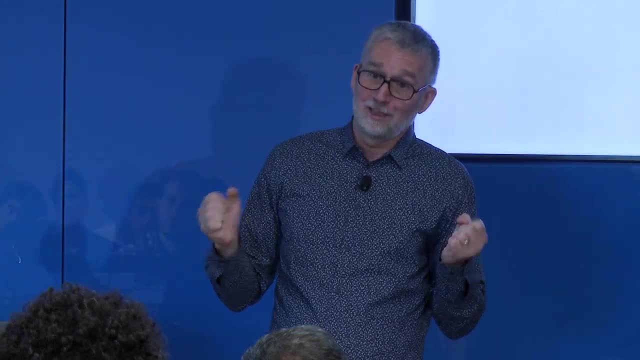 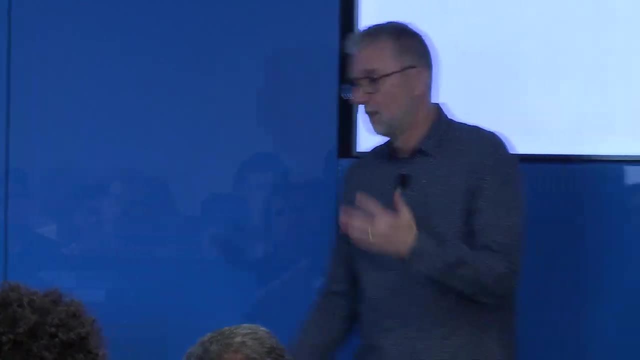 So at least it's not anti-stability fighting against you as most possible and then it gives you the maximum probability of having crossings and stuff. So I think it's an area that's wide open for somebody to come in and do a much more refined mathematical analysis. 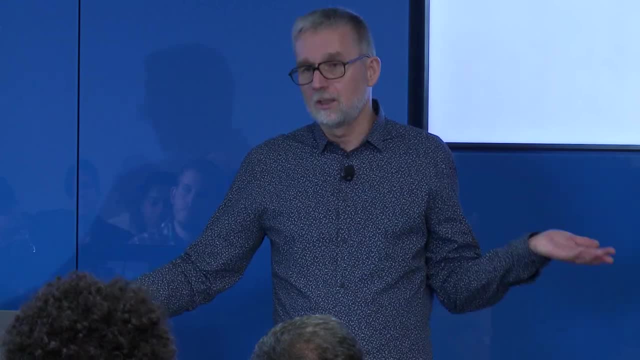 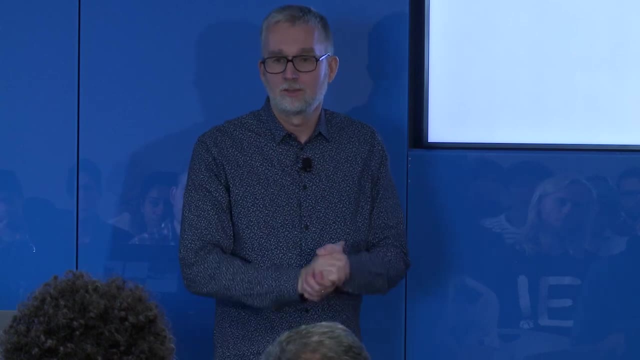 than what we've done. But I think we've got a really nice proof of concept and a conceptual framework that someone can come in- who's maybe of Jean-Jacques' stature- and clean this up. But I'm probably not able to do that anymore. 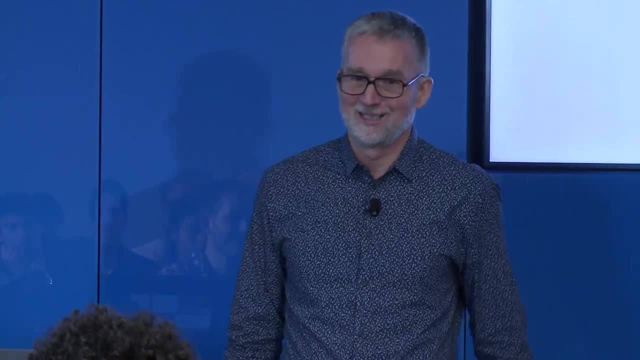 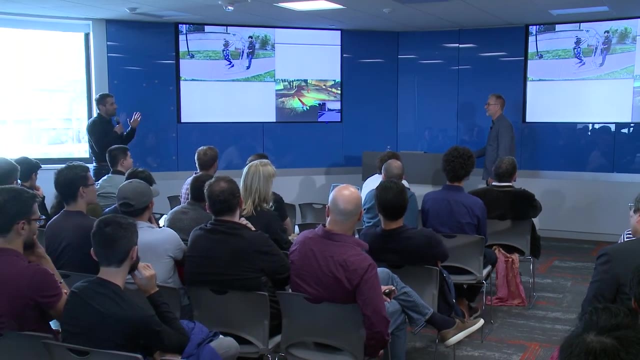 When I was 35, yes, I think I would have done it, but I don't know if I can do it anymore. Okay, I'll take the opportunity to answer some questions because I wanted to push you a little bit more on the hybridness and bookkeeping.